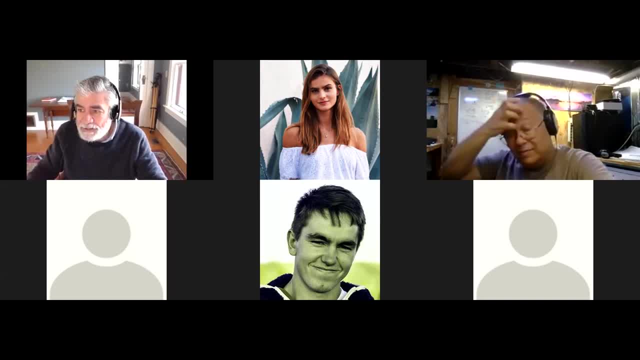 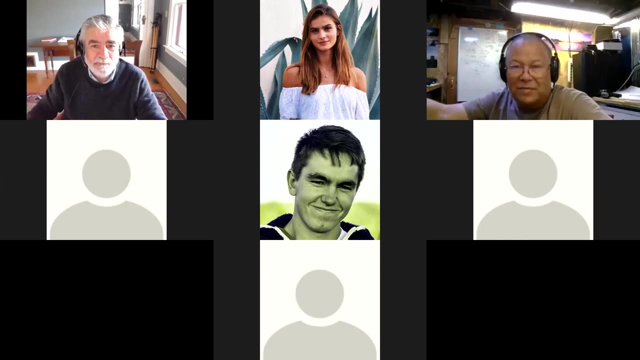 writing OCaml was also a little bit idiosyncratic. Oh God, maybe I should just try to like open a new link. All right, because this page is not very Here. we go So, let's see. So I mean, if we go look at Staten's algorithm, just real quickly. 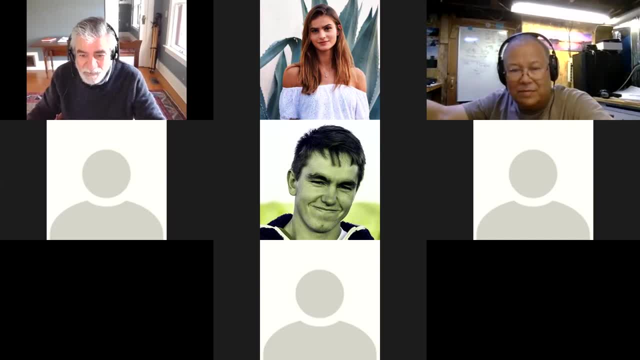 because I know a number of you spent time trying to get it to work and then Finley figured out the problem, which is what I suspected was. the problem was that, David, They were getting stuck whenever they had an implications in the assumption. 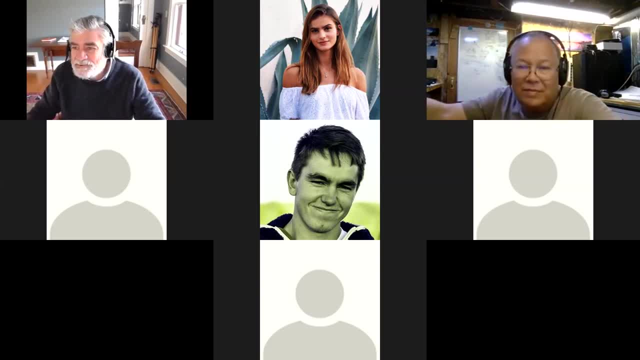 And so it's. Can you see that? Is that big enough? You're not sharing yet. Ah, so you definitely can't see it, right? No, no, we see you in Oregon, where you're not sharing. Right, yeah, okay. 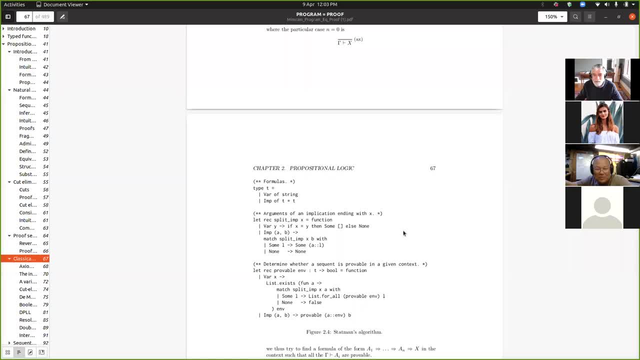 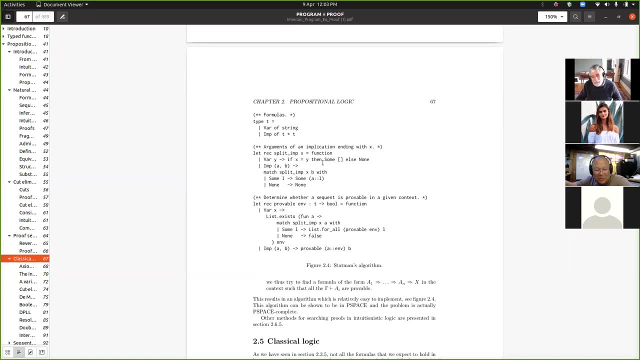 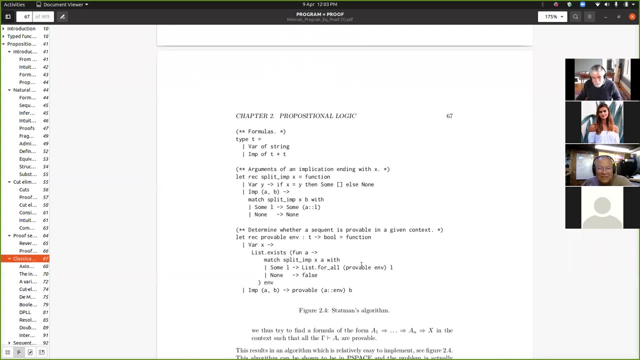 Okay, so here we are. We're going to go back to the Staten's algorithm here. Much better. And the problem is is really: is this? Well, I don't know, Where do you see the problem? Is the problem in here? You want to like? 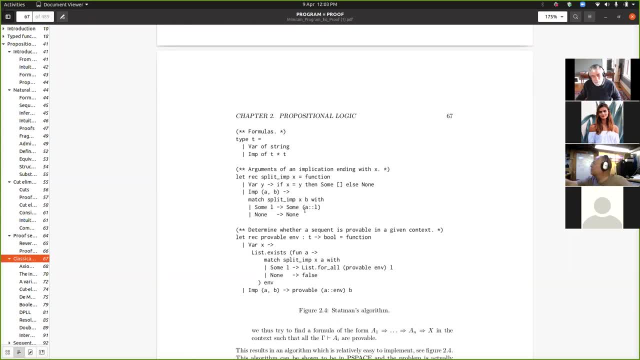 instead of putting Just putting A on here, You would be nice. You could either solve it two ways, I think. Fin, what did you do? You solved it by In the implication case of the provable function. then you want to. 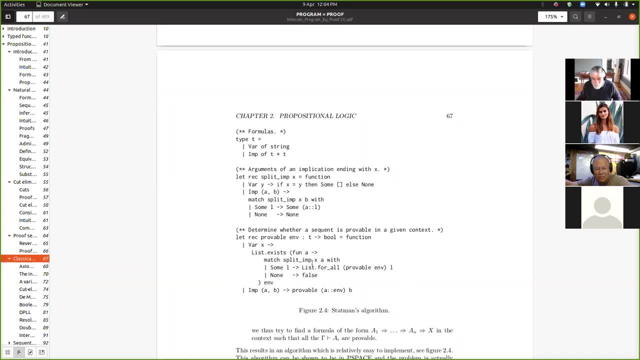 Yeah, Not just cons, that you want to make sure that you're keeping variables at the front, This one right here, Yeah, Yeah, I think another option could be in the split to put implications at the the end, or something like that. you know, maybe could you do it up here. well, that one's kind of. 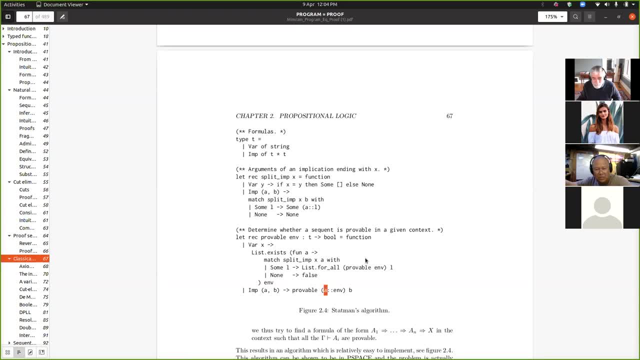 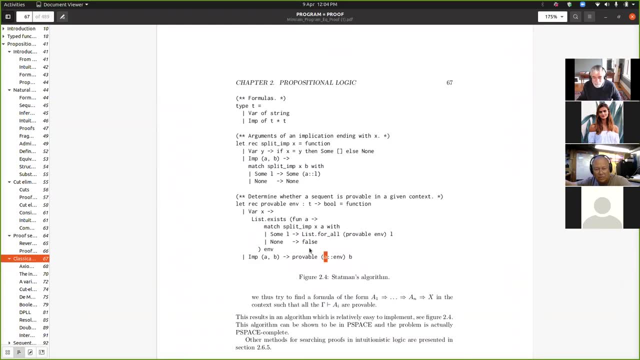 weird, because what it does with that list that it builds there is it just tries to prove everything in it. so it doesn't really okay. it doesn't matter the order of that list so much. what matters is the environment, like the order again, uh-huh, ah right. 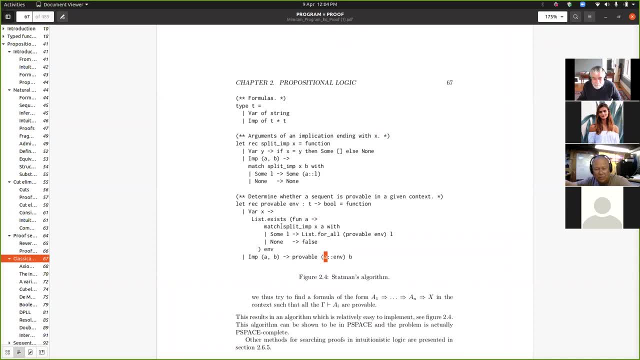 so this: here you look at a and you say, um, if it's a variable, you just stick it right on, and if it's an implication, you travel down the list until you find a spot where the next thing is not a variable and then you insert it. if i- i just glanced at your answer- is that 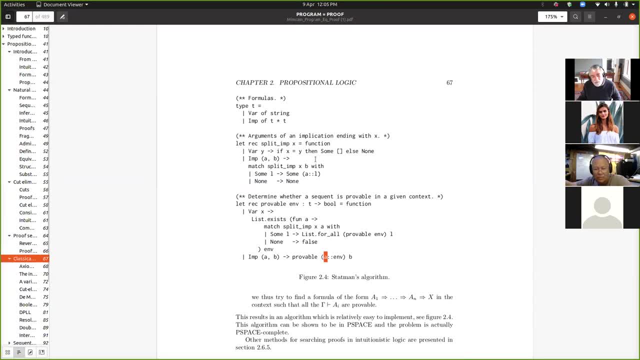 correct. yeah, that's what it does. yeah, so that's pretty interesting. have you sent mail to mimrom? no, well, you need to. i mean, he asked people to fix things and it doesn't work. my first suspicion was that somehow the fact that okama was called by value and haskell is called by name might be. 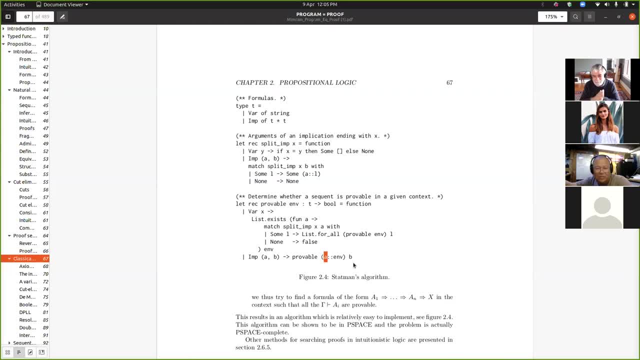 causing a problem, some difference. but that didn't really make sense, because usually you go the other way. like i didn't run it no camel, though i assumed it worked, although last night i was like, oh, i should program it no camel and see what happens, and then just get this. 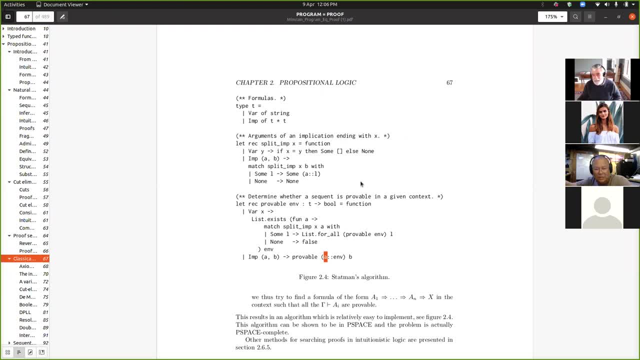 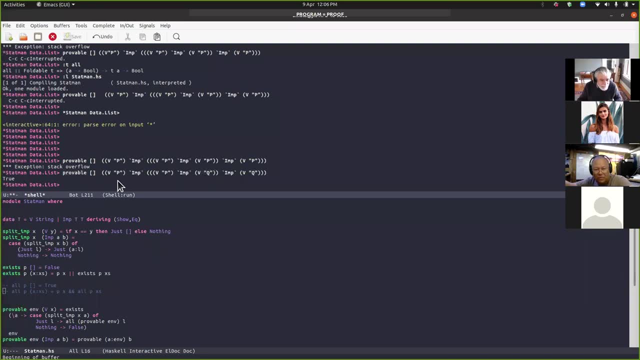 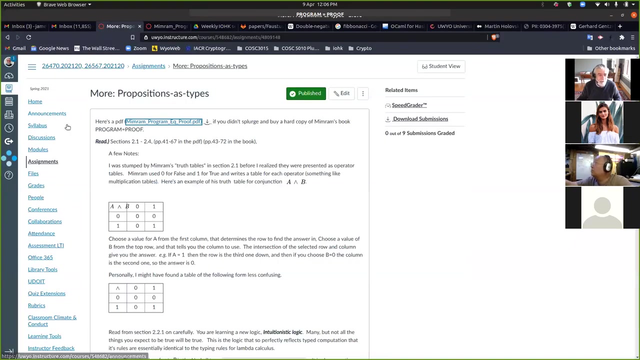 code and put it into camel and see what happens. i guess you did do that and did the same thing. um, i don't know, do i still have it here? oh yeah, here's. here's the code without his fix, and you know, i guess maybe my note really says it um better in the announcement, like some simple. 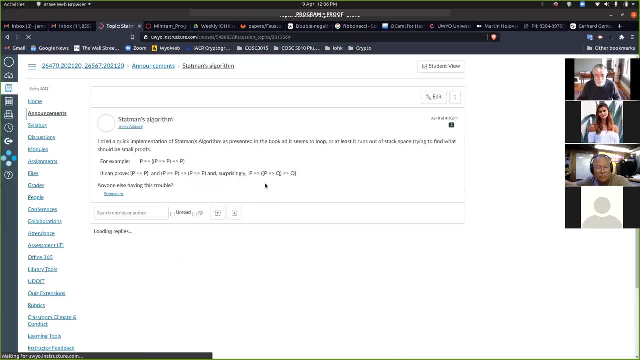 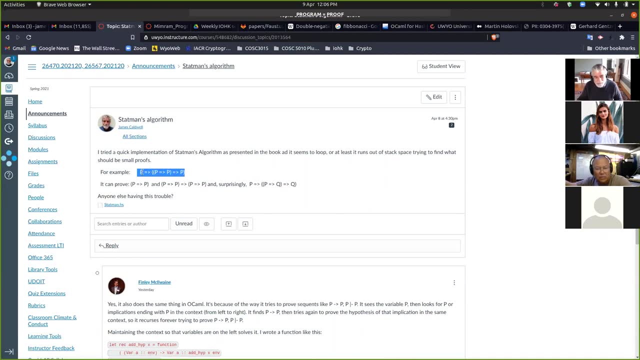 things, lots of interesting things are provable with it, but it misses some. so, like this one is not provable, because what happens? first the p gets put over into the context and then the next thing that happens is p implies p gets put over into the context. 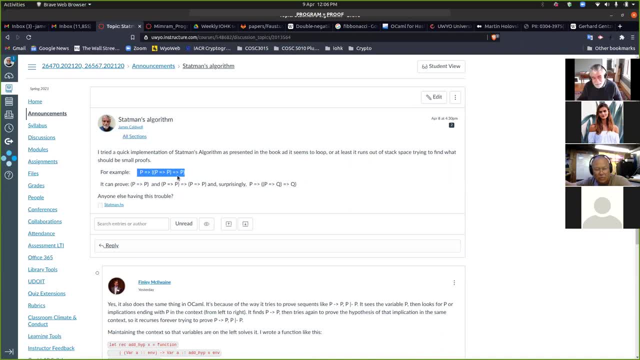 but that's to the left of p, and so now we could, should be able to get a proof. but it sees the p implies p and it kind of gets stuck in a loop trying to process: p implies p, which is true. so p implies p is um provable, so it shouldn't be a problem. but it should also at that point find the fact. 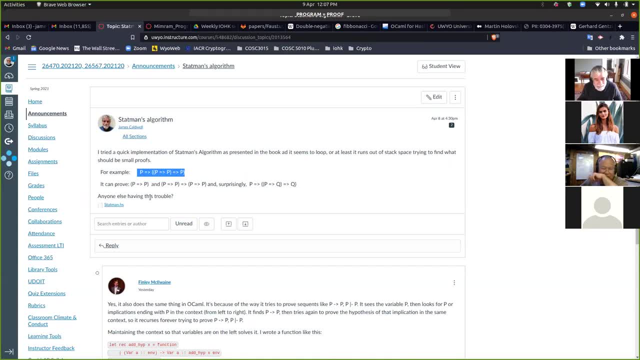 you know it's looking at a context with p and P implies P and it's trying to prove P and that's an axiom. but it can't see it because the P implied P is to the left of the P. It can prove P implies P. 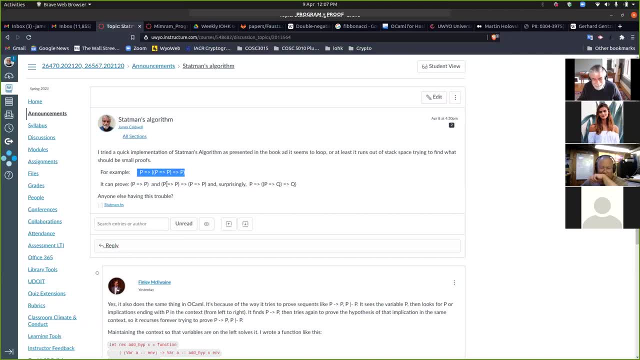 it proved: P implies P, implies, P implies P. That makes sense, Cause this is just an instance of this one I just substituted in this one and it gets this one. That's weird. So anyway, I would say send mail to Memram. 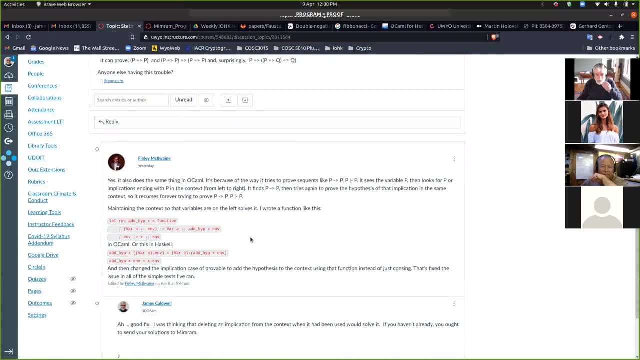 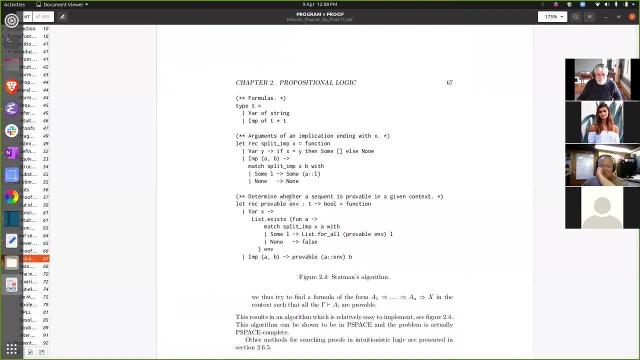 tell him, you know, tell him both his OCaml code and his Haskell, and it doesn't work in Haskell either. I think that's pretty, pretty cool. So when I looked at, let's see, See, he's using this also. this really to me. 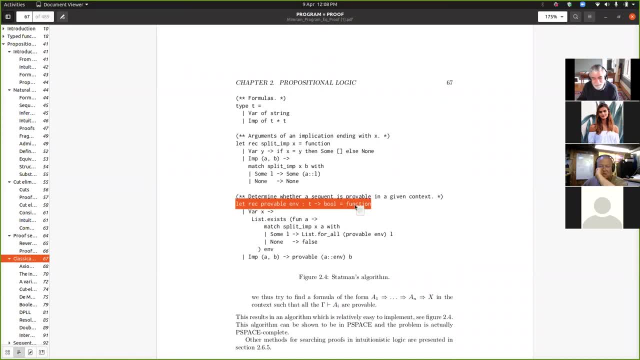 kind of ugly OCaml style where you know you say over here function, and then you list this and you list this. I mean there's kind of a Haskell style that, but it makes the code pretty hard to read The fact that what you don't get 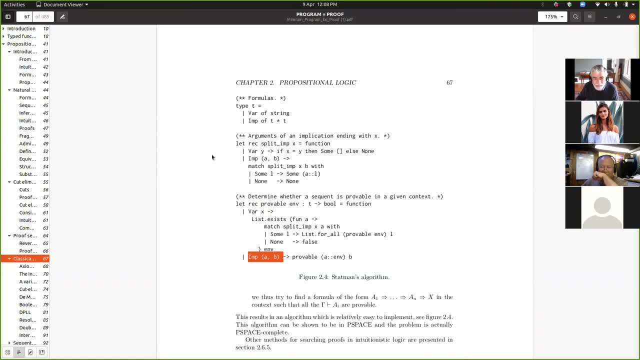 if you don't like, dig a little bit deeper into OCaml, is that split imp is a function of X and a term one of these T things, And so you kind of miss that. there's this third argument, if you not like, more well versed in OCaml. 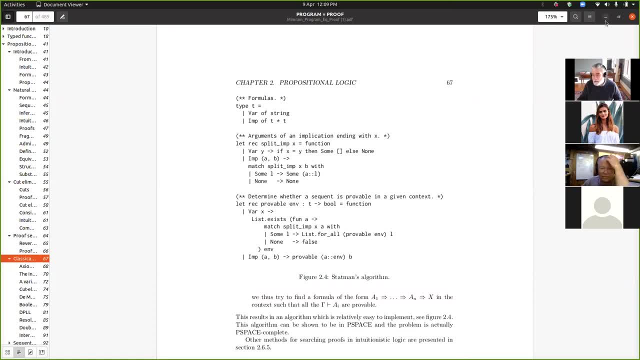 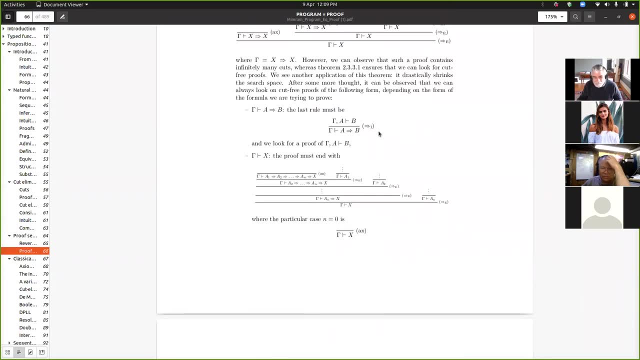 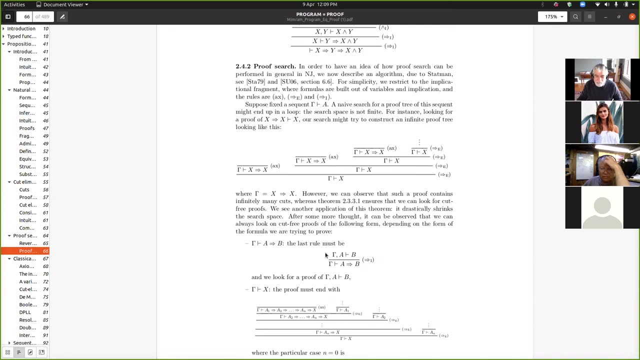 it's a little harder to read. This code could be easier to read for non OCaml programmers. So anyway, good work, Finn. That was nice. So we'll do some proof today. Maybe we'll do that. Do that one. 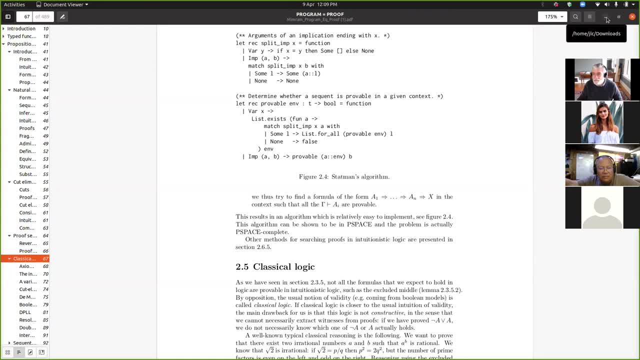 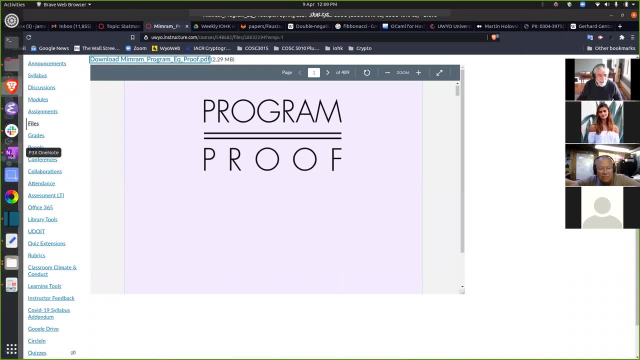 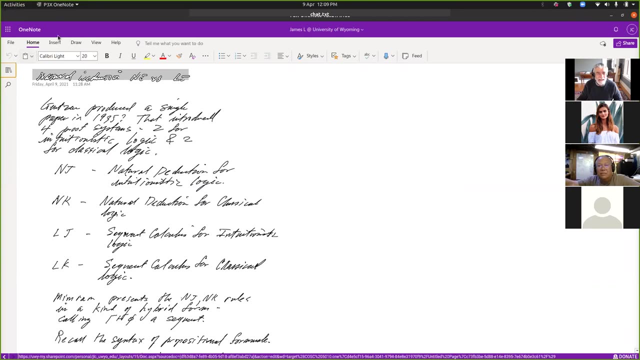 And we can see how it works in the sequent style. So, oh, this is interesting. I mean kind of like out of desperation. I searched one more time and I found that there's one note for Ubuntu now and I think: look at this, I can. 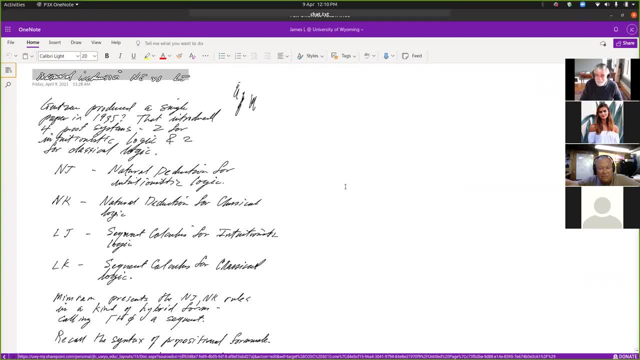 write on my iPad. this is what I've always wanted: to be able to write on my iPad and have it show up. so I've got my notes. it's a little bit of a lag, but um, I've got my notes here for today. you know they're probably not enough for the whole time, but um, 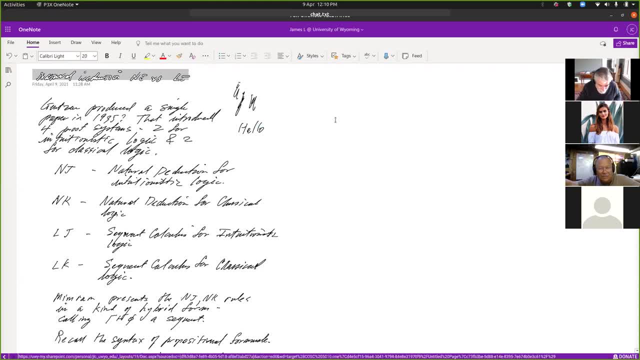 oh, what do I want to do? I want to go to the eraser and just erase this, okay, so you know, Wadler touched on this and you've been looking at um NJ natural deduction and I tried to in the reading of the NJ natural deduction and I tried to in the reading of the NJ natural deduction and I 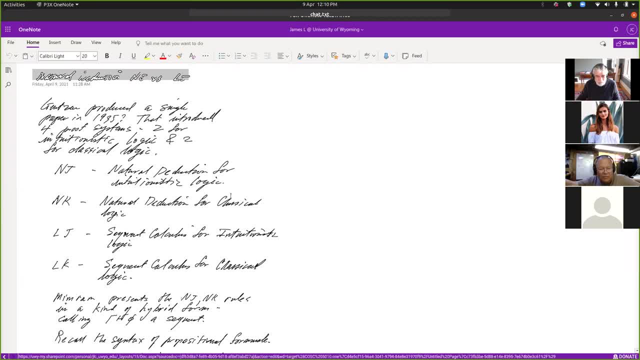 knew it was a long story and I had to read to it separately and then use it here. but I failed because I actually couldn't help but reading Skip the classical natural deduction part and I also had you skip the sequin calculus, even though, as I said and Wadler's talk, I kind of prefer the sequin calculus. 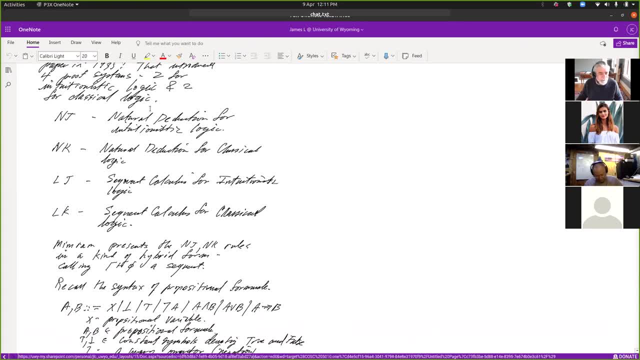 and I'll show you why. so I mean, we'll look at the sequin calculus rules and see them, but this was Gentian, it's not 1935, what did Wadler say was? is it 1935? it was 1935.. 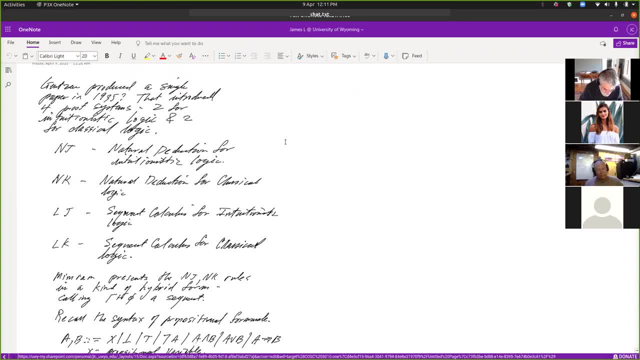 1928? Or 34, maybe I forget. I try looking it up. I have the actual paper right here but it doesn't have a date. You'd think in this book where they published all of Jensen's works, they'd have- and this is a translation of the original paper. It's: 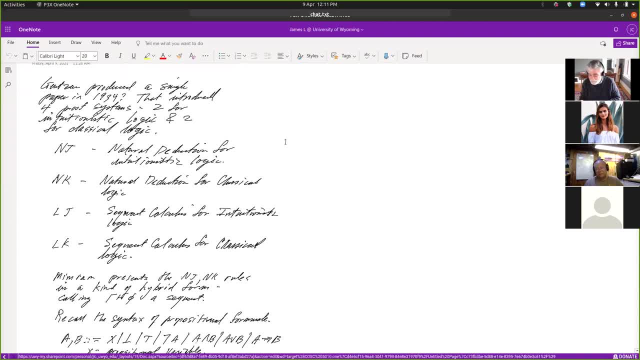 called Investigations into Logical Deduction and it's probably one of the most important papers in logic in the last century Because he invented. you know, we had those Hilbert style systems and I did some proofs in a Hilbert style system and it's just like you're. 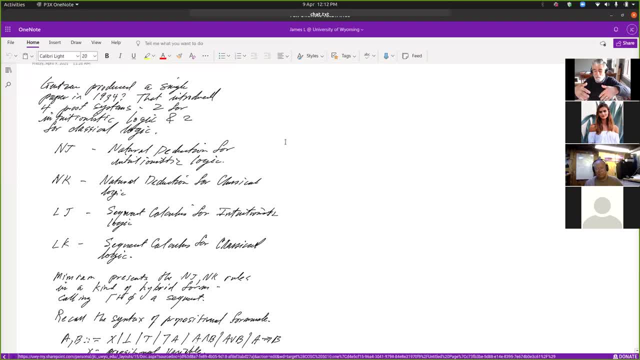 always trying to work from the axioms to the goal, And Jensen and some others before him or around the same time had been trying to figure out a better proof system that matched more closely the way that mathematicians do proofs, And Jensen came up with four systems. Now the interesting thing here it also, I think. 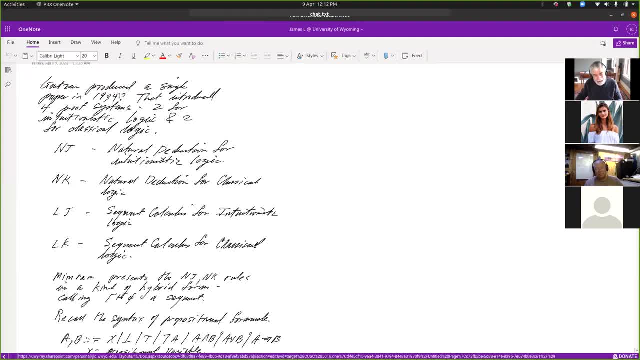 really is is that at this time, you know, in the in the 1930s, intuitionistic logic was kind of like vying for dominance over classical logic, although it had a terrible uphill battle to fight to be able to do that. But 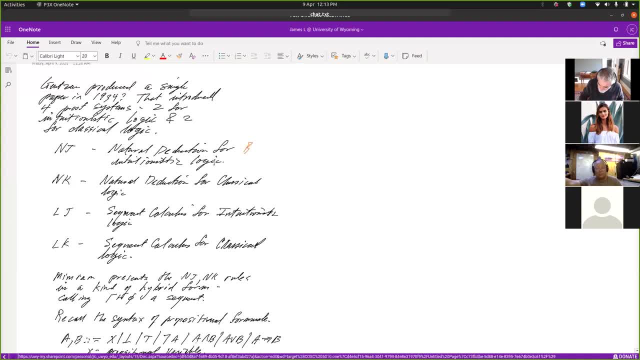 this logic was developed by Brouwer In response to you know the, you know the. you know the paradoxes in set theory that that Hilbert was reacting to and trying to say, okay, we're going to make sure, we're going to see if everything we're just going to make a uniform. 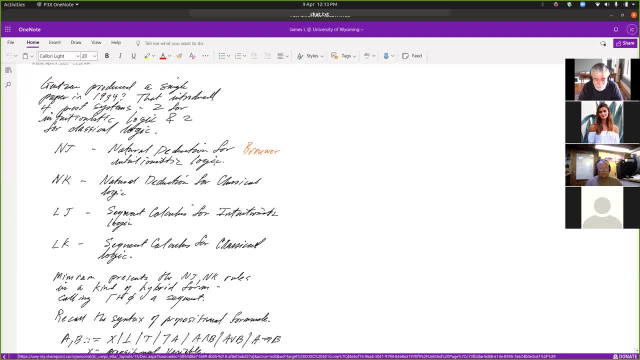 proof, decision procedure for mathematics And so. but Brouwer's answer was no, look, the problem is excluded middle. The problem is the formula P, not P. And he said: look, if you want to have evidence. the classical notion of, of disjunction. 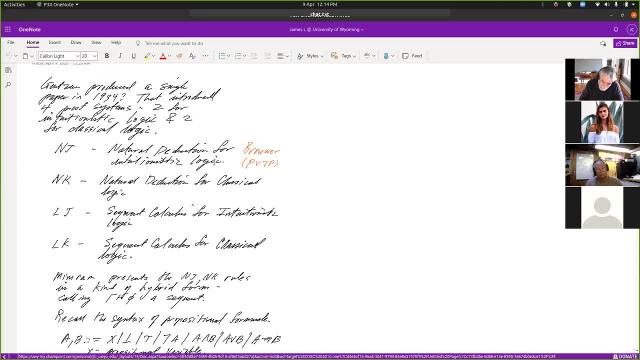 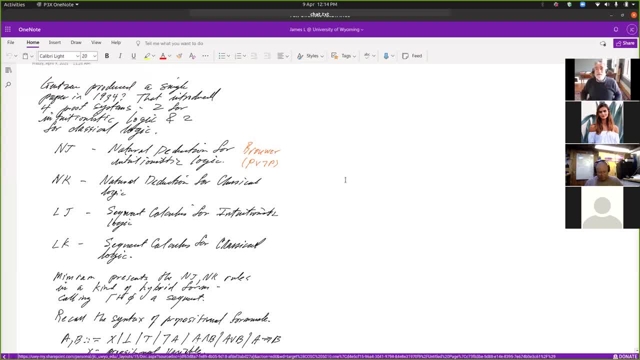 Oh god, I used to know a really good example, I think it's something like: there are two irrational numbers. How does it go? Oh, something like, oh, two irrational numbers. numbers say A and B, such that A to the B is rational. 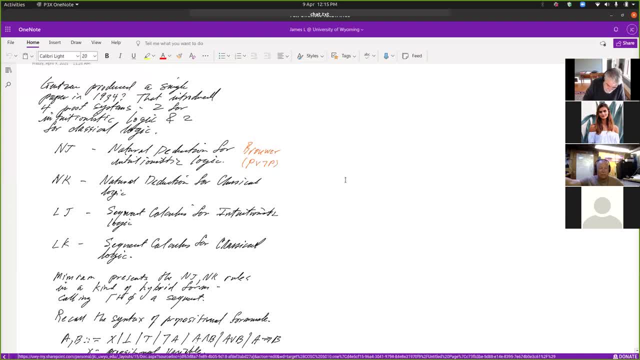 And so then you look and you say, okay. well, look, either the square root of 2 to the square root of 2 is rational. We don't know what the square root of 2 rates. the square root of 2 is. 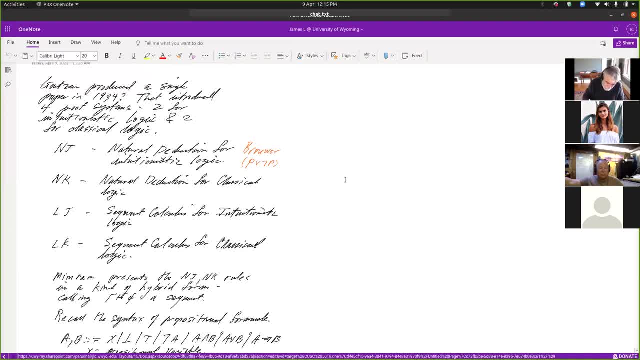 Or actually, maybe since then number theorists have proved it. But you say: or if not, square root of 2 to the square root of 2 to the square root of 2 is equal to square root of 2 squared, which is rational. 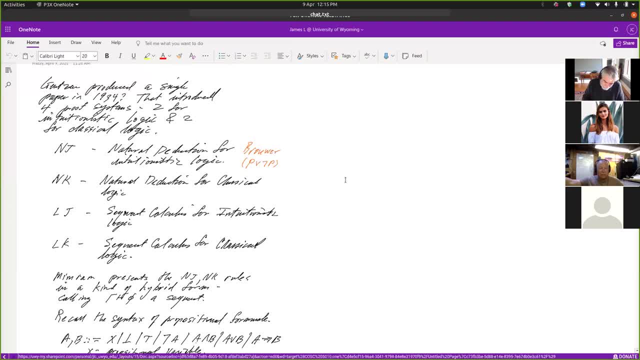 So this proof proves something that has been since proved by number theorists- And we know which one it is, although I forget and I don't really care, But it's a good example of a proof that uses excluded middle. So I guess I should say: 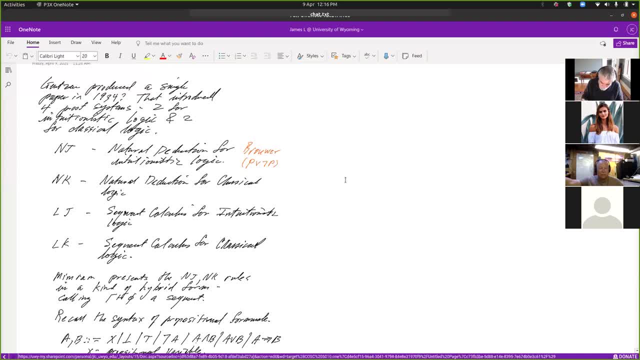 square root of 2 to the square root of 2 is rational or not? If not, well, and if it is, we're done. So I should be maybe more a little bit more careful here. So, if it is, let A be equal to the square root of 2. 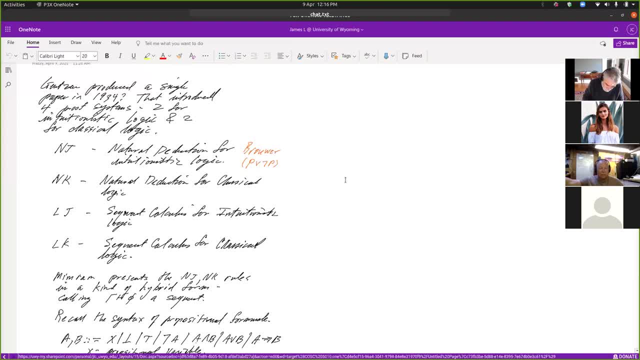 and B be equal to square root of 2.. If not, then let A equal square root of 2 to the square root of 2. And B be equal to the square root of 2.. So this is an example of a proof. 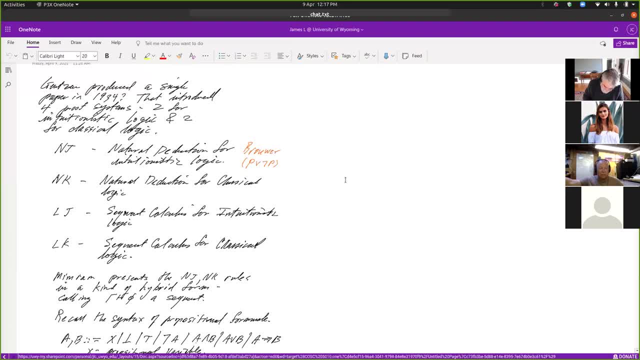 that Brouwer would say: you haven't really proved this. You've proved that it's impossible, that there is not some square root of A and B, such that A to the B is rational. but you have not told me what A and what B are. 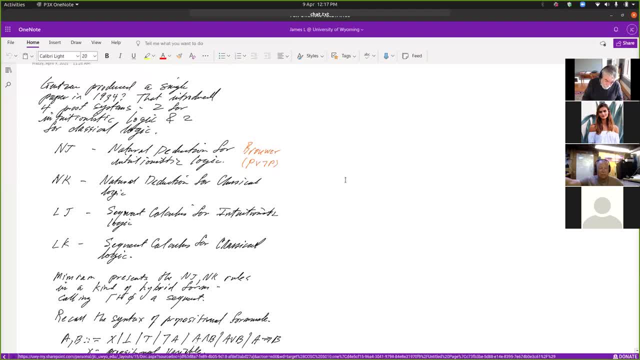 So have you written something we're meant to say? Okay, Huh, Excuse me, Have you written? we can't see what you've written. Oh, oh, I'm sorry. Right, I need to. oh God sorry. 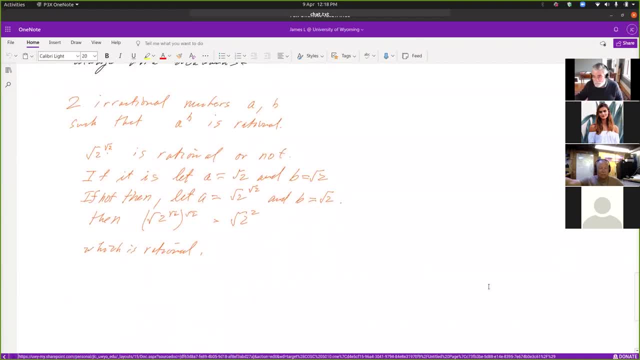 I need to scroll on a separate on my mouse here to show you. So there are. so you know there are two irrational numbers, A and B, such that A to the B is rational And it starts off with a P or not P thing. 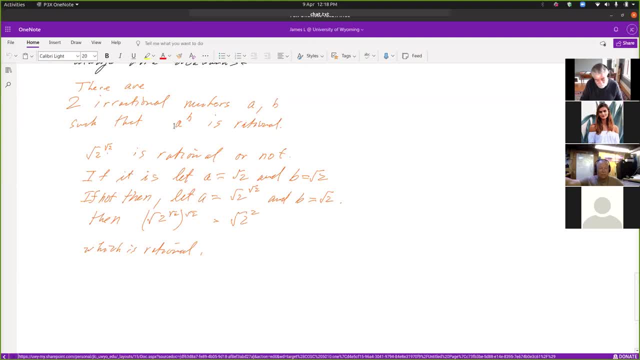 Because it says: square root of 2 is rational or not. square root of 2 is rational, But if it is, we're done, We know what A and B are, And if it's not, then let A be square root of 2. 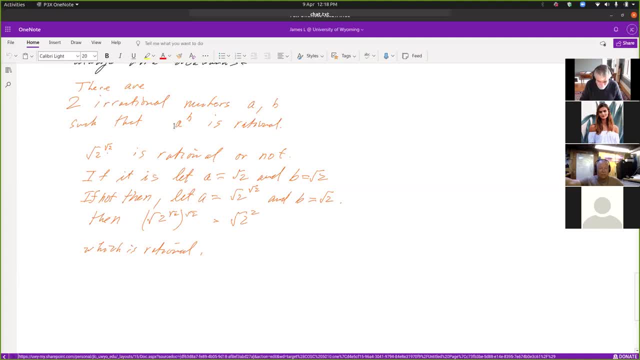 raised to the square root of 2 and let B be square root of 2.. Then you get this. so this is equal to 2, which is rational, And I mean, if you try to think about it. I mean, what is the square root of 2?? 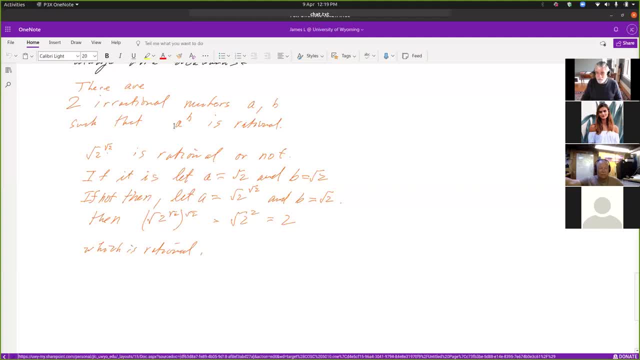 1.1413.. It's an irrational number. It's an infinitely long expansion of decimal digits, And Brouwer would say this is no proof, Because you have. you haven't really told me what the rational numbers are. Now, if you wanna say it's impossible, 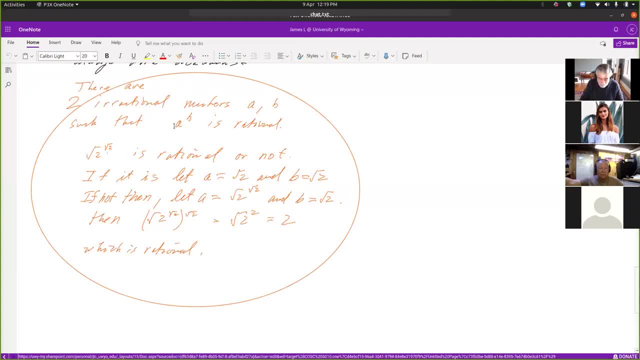 that there are two rational numbers, that it's impossible that there are not two rational numbers such that A to B is rational. he would agree with this. So this is proving essentially that a double negated version of this is true intuitionistically. So we'll try to talk a little bit more. 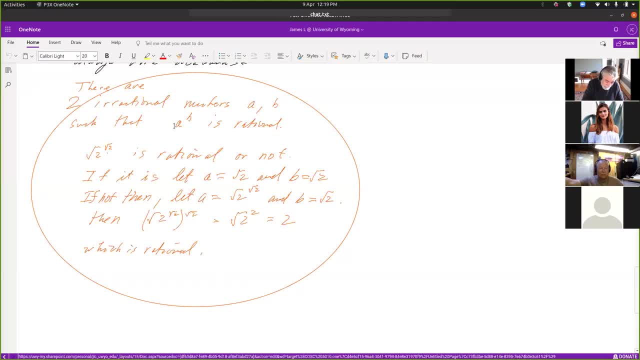 We'll talk a little bit more about that, maybe, But so I mean the fact, though, that Genson was so felt, it was so important to do the intuitionistic versions of natural deduction and sequent calculus as well as the classical logic version. 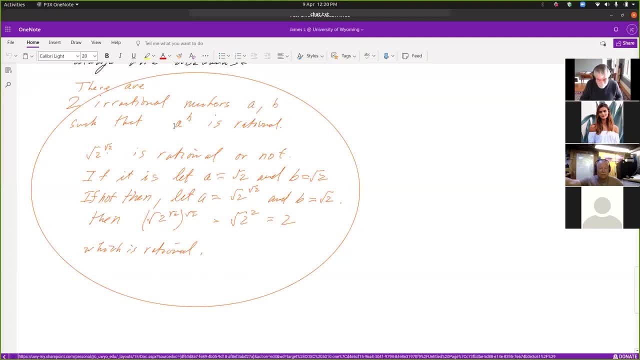 And you know if you read, if you look at that part and saw the only thing for to get the classical version, you just write down gamma, turnstile A or not A. That's a rule. I think you have to scroll again. 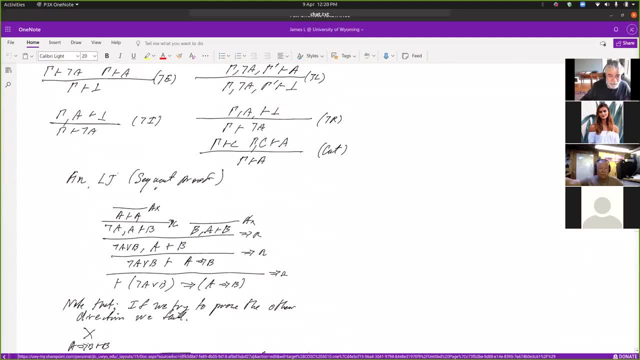 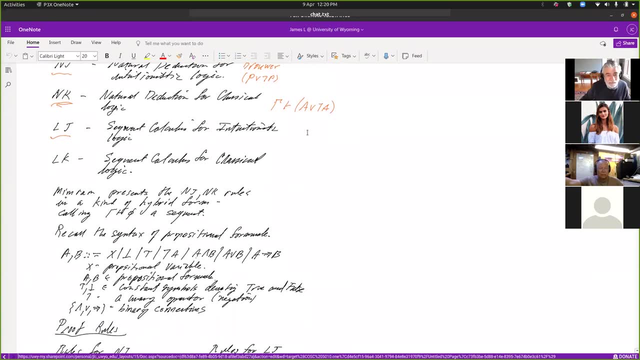 Ah, thank you. This is a little bit confusing because I have to scroll on the separate thing. Let's see: what does he do to add in there? Classical for classical, he just adds gamma, turnstile A or not A. In fact, I think he might do it the other way. 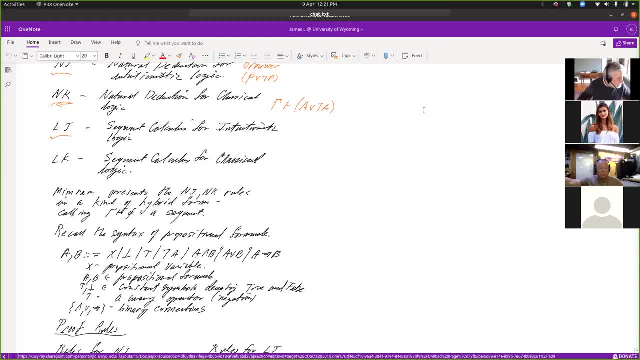 He might. he might always write not A or A, which I find a little bit backwards, but- And we're gonna see something interesting about the sequent calculus. So how'd it go? trying to do the natural deduction proofs that I assigned? 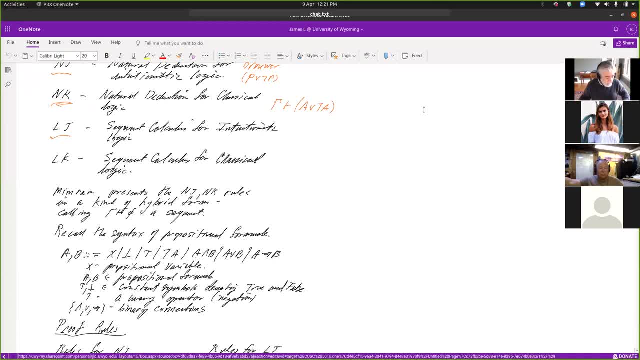 Did you find it tricky to figure it out? I mean, it's kind of a puzzle. Did it take much time? I found I had to look at various additional examples, but once I got the swing of it because there's commonality and similar approaches. 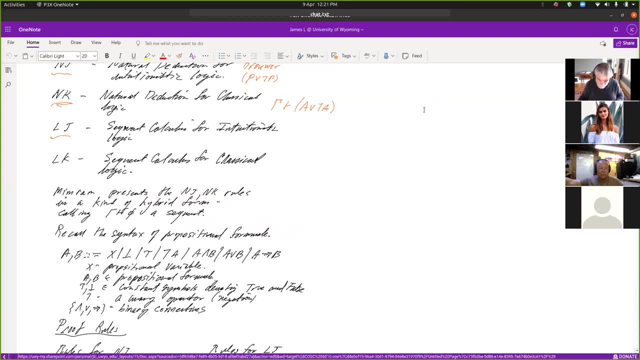 between a lot of the examples I found. once I got that into my head. it's just a matter of starting somewhere, trying to follow a path and seeing where I got and then backtracking if it wasn't going where I wanted it to. 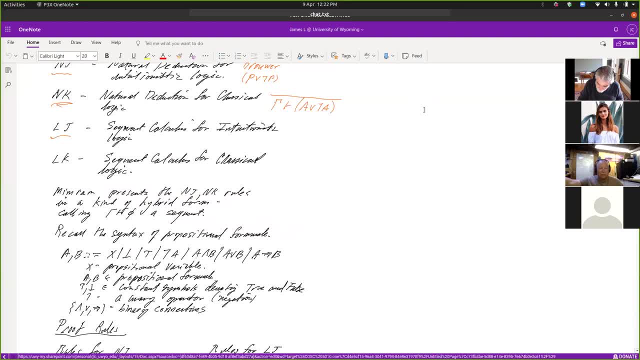 Uh-huh, It takes some, and so LEM, that's the law of he names the rule. LEM and that's the law of excluded middles. You just add this and you can plug in any any formula for A there. 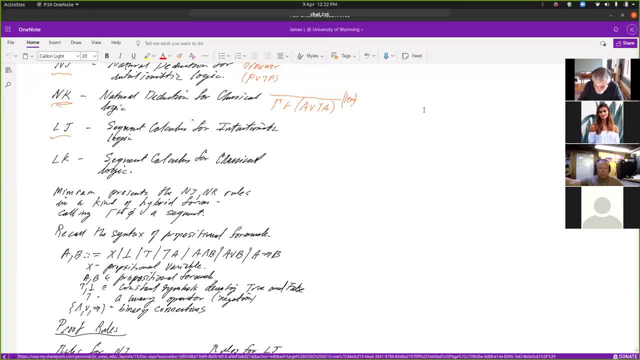 and you and you, you know that's true, And so you can reason forward on that. And then what I wanted to do today was maybe show you the sequent calculus for intuitionistic logic and how it relates to the thing that you did the homework with. 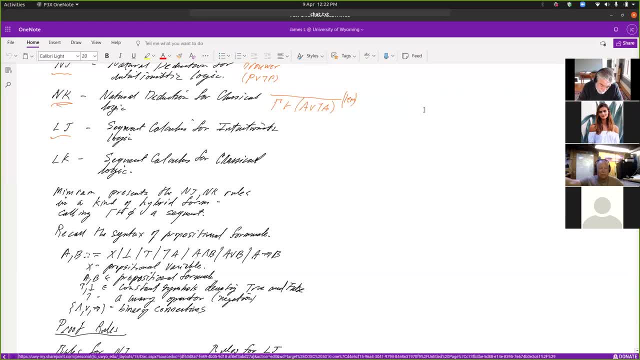 the natural deduction, And I mean we don't have to do it, but the sequent calculators do have the way for classical logic is rather interesting, because you don't have an axiom like this. You just allow multiple formulas on the right of the turnstile. 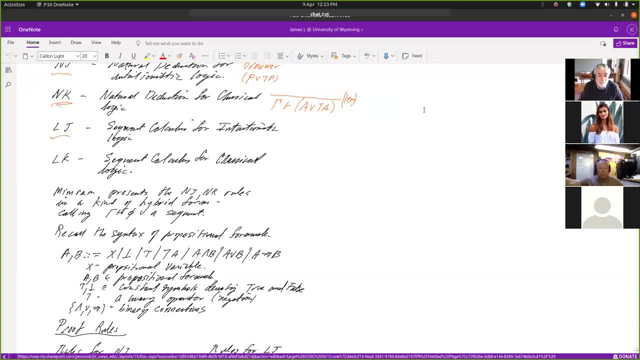 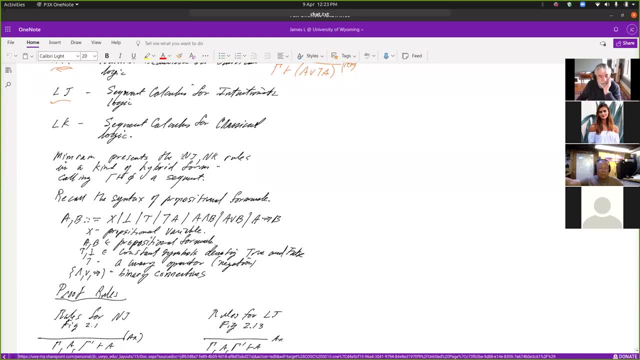 So you know. I wanted to point out that MIMRAM presents the intuitionistic rules in a kind of a hybrid form by calling gamma-turnstile-phi a. what is it gamma-turnstile-phi? Oh, how come I can't get that to work? 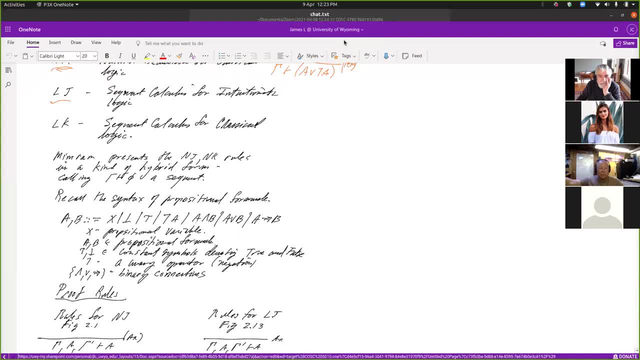 Uh-huh, Okay, annotate, That's okay. I don't want to scribble all over this thing. anyway, Maybe I'll just use the spotter and use the spotlight. Whoops, This thing here. gamma-turnstile-phi. 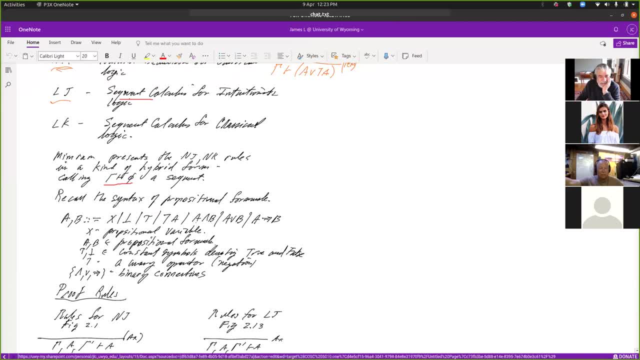 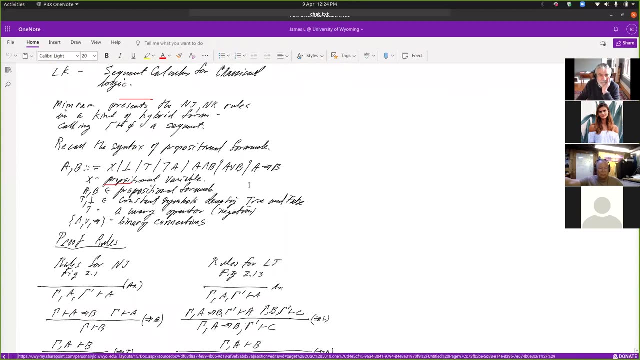 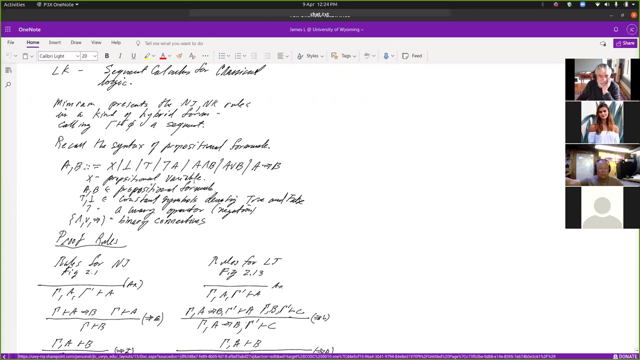 He calls a sequent And so. but when he presents his NJ rules in that form- and you know, if you had tried to do any of um these assignments before you heard Phil Wadler's talk- you'd say, wait, his rules look different. 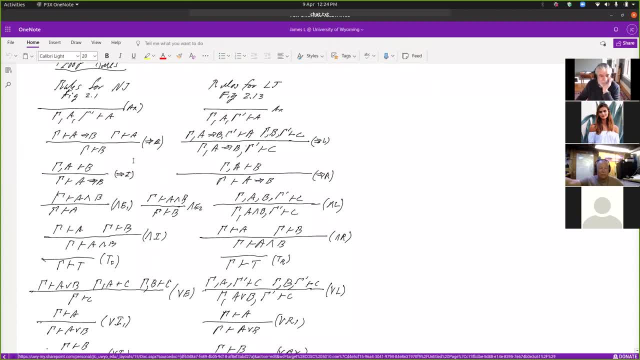 Like he's doing something different. The form of his rules are different And that's because he never had the gamma. He just writes down the formula And then you plug the assumptions at the top And as you discharge, then with implications on the bottom. 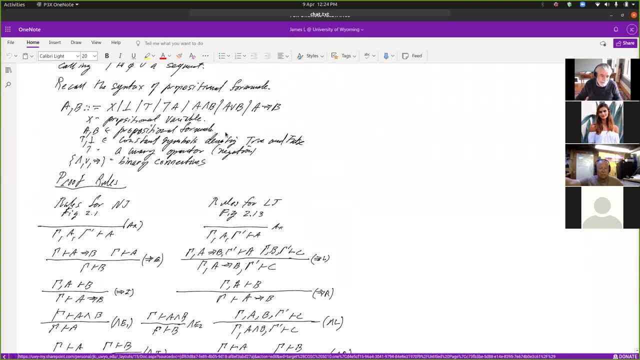 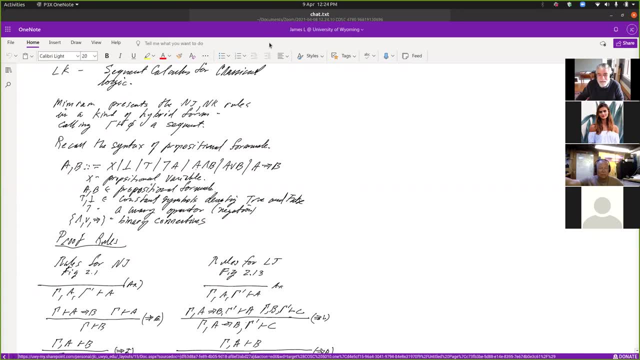 you write them out. But anyway, here my main. so let's look at the quickly the syntax. I think you all got this. So the syntax of this is that that. what happens with that? Okay, yeah, 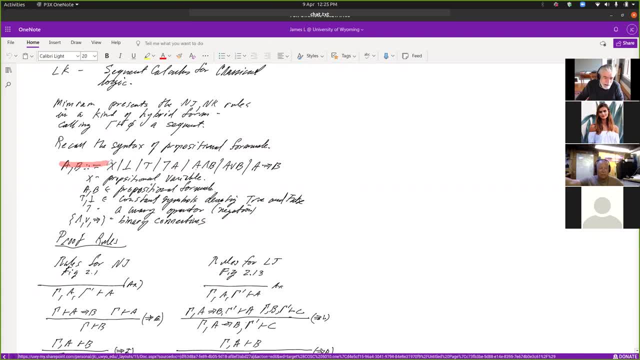 The syntax is that you either have a propositional variable, you have false, you have a symbol for true. Those are constant symbols in the language. You have not a which is unary operation which, in the proof system you can see, is the same as negation. 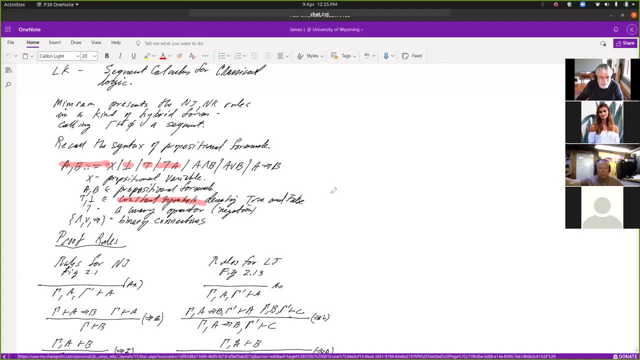 And then you have conjunction and disjunction and the implication. So that's the logical language that we have for for these proofs. Now, what we don't have yet and we couldn't add, it's not. it's very easy to add actually. 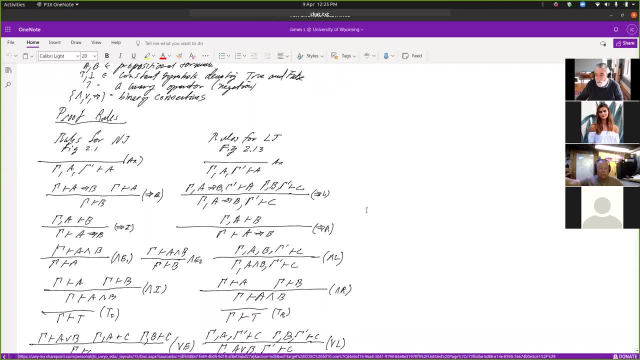 is the rules for for all and exists. And then you get first order logic, And Genson did those, all of those, He didn't just do propositional logic, He did first order logic. So anyway, these are the, these are the rules for NJ from figure 21 of Mimram's book. 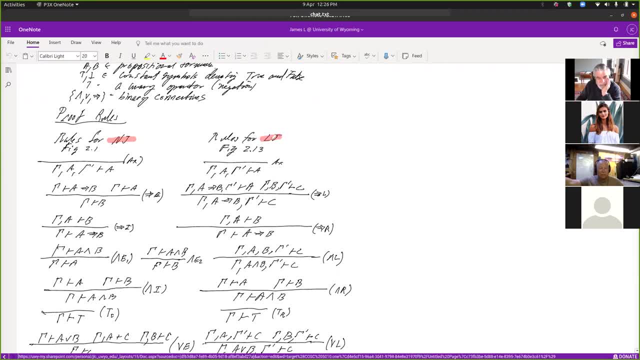 And these are the rules for LJ. So this is the sequent version- is the L calculus and the natural deduction is the N. So I'm still confused, And I mean the answer that I got from Wadler was there's less writing. 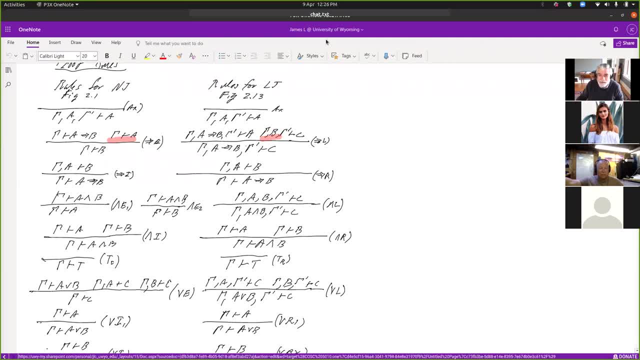 And okay, Maybe that's okay, But that's a reason anyway. So what I hear, though, from philosophers is that this captures, especially without these sort of pseudo sequence that Mimram introduces. Philosophers seem to think this is a singleton. I'm not sure if that's a children's book or if that's not. 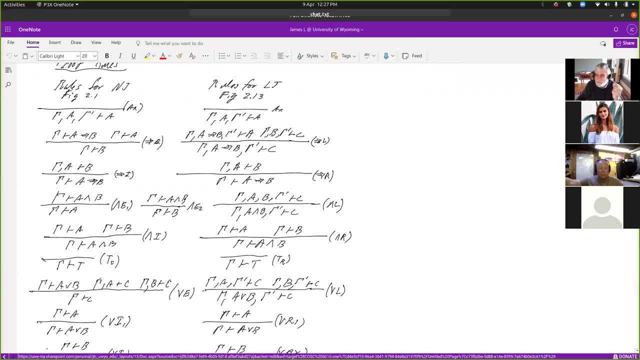 But I'm not sure if that's what you or maybe people in philosophy think, And I'm not sure if that's what you or maybe people in philosophy think- captures the essence of human logical thinking. and if you have trouble using these rules, then you really can't think very clearly. and I'm telling you, if you take um. 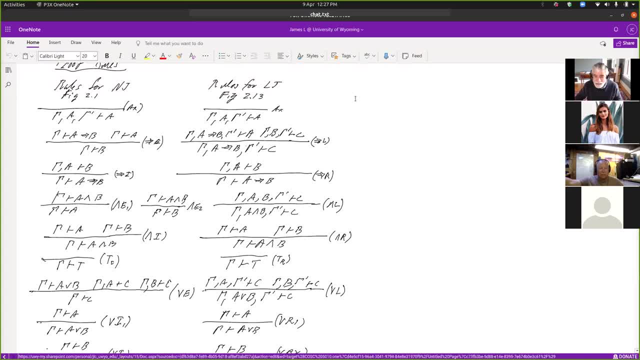 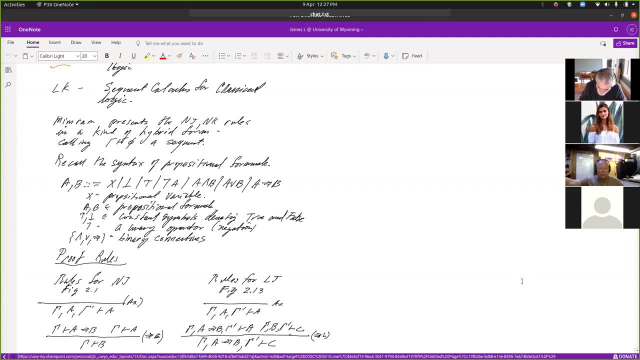 let's see, let me scroll back up a little bit where I have a little more space over here. if you think of kind of like um, if this is the set of all um formulas and then this is the set of all um classically provable, well, we know that um. you know, like we can't prove not p or not p. 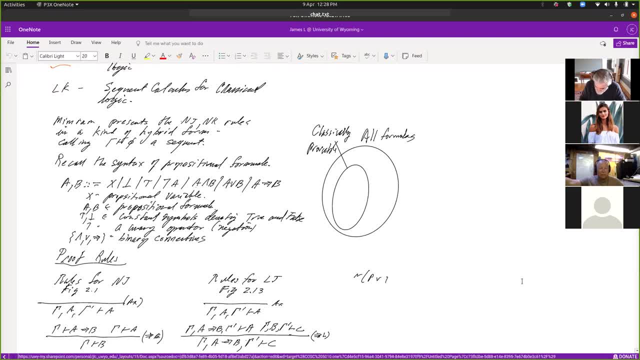 well, I mean, we can't prove near p or not p is what I meant to say. um in intuition, intuition is the way to do it. intuition is the way to do it. logic. so we know that p or not p is is somewhere in here. let's say it's right there. but then that means that the intuitionistically provable ones, 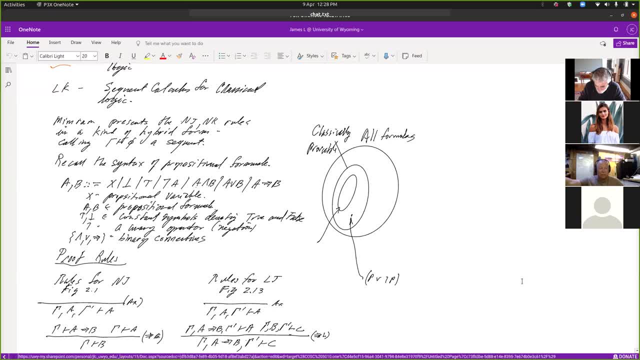 are smaller and in fact, there is no intuitionistically provable. it's not like it over, it's not like there's a point out here. there's something that you can prove intuitionistically that you can't prove classically. okay, so now there's a big caveat on this thing that I just showed you, because I show you this. 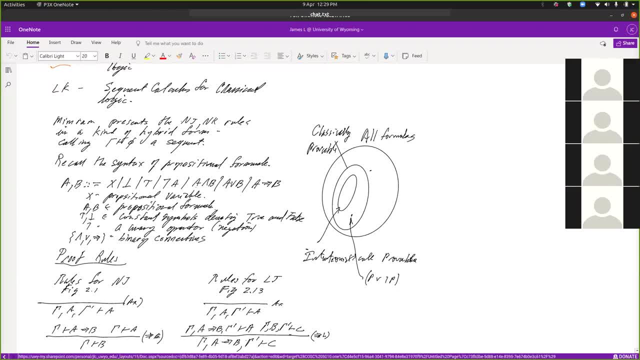 and then you go like: oh wait a minute, intuitionistic logic is not very strong, it's it's weaker. but then we're going to see that it's actually. you can prove all of these things by. I'll show you in a second. but if you take one of these formulas out here, 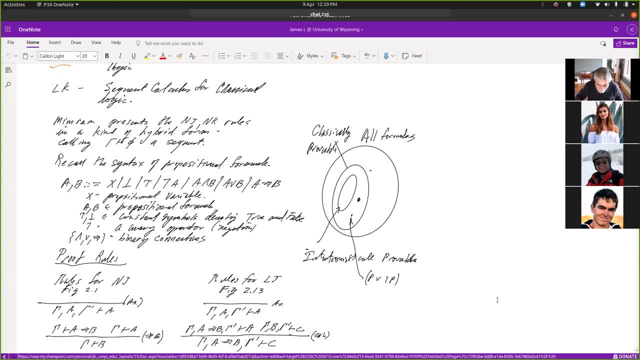 and you take the um, the classical rules. so if you take, you know, not nj but lj, I'm sorry, n uh nk, which is the classical natural deduction. so, oh no, I don't. what is this? oh god, somehow or other, this damn thing took me into some weird environment. okay, 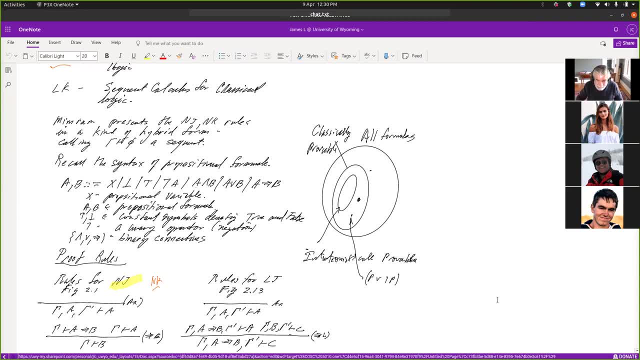 um. so if you look at a point out here like um, p or not p, well p or not p is not hard to prove in nk, because the way you get nk is. you add that as an axiom. but suppose you try to prove something else that's in this space. 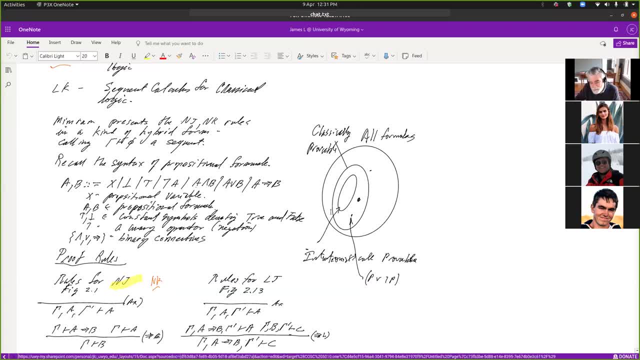 that's classically true but not intuitionistically true. and if you do that, the proofs are really hard and in the worst case what you can do is you can just sort of take um, you can, you, you can basically make a truth table. so what you could do is you can like say okay. 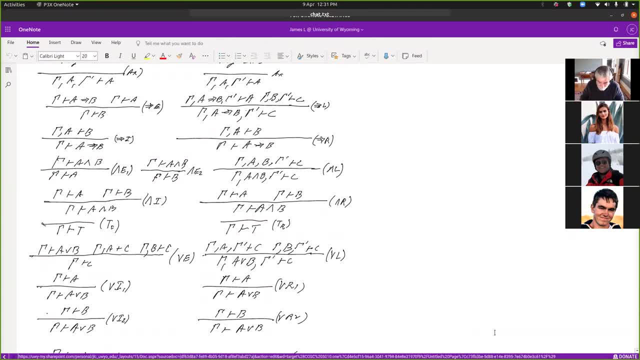 um you can use if, if your formula has um five variables in it, you can make five instances of the use of excluded middle and then you can do your or rule to try to work those down. so if you have p and q and r, you know, or p and q. 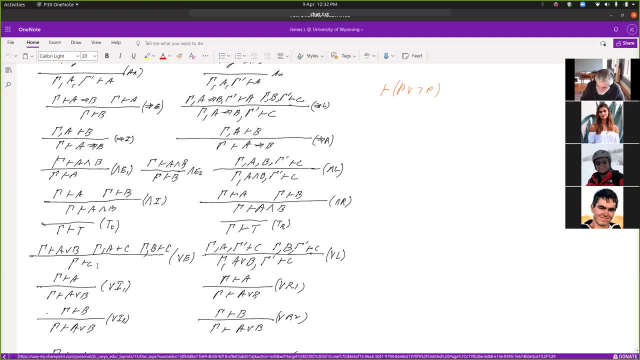 you could start off with something like this and then you can work forward from that, using the or elimination rule to get rid of that war. but it's kind of like writing down a proof that's just a truth table, because all you're doing is kind of like splitting this and splitting this. 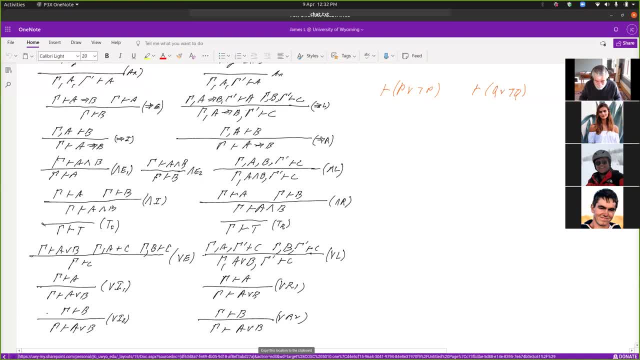 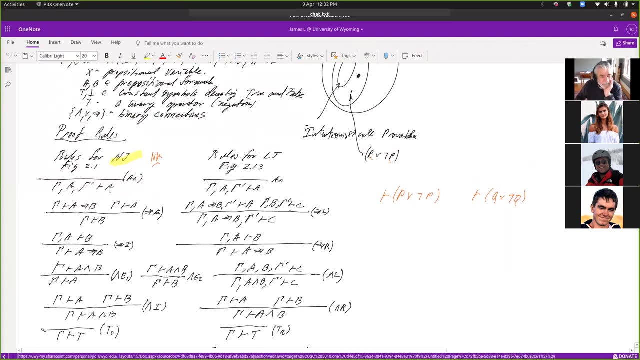 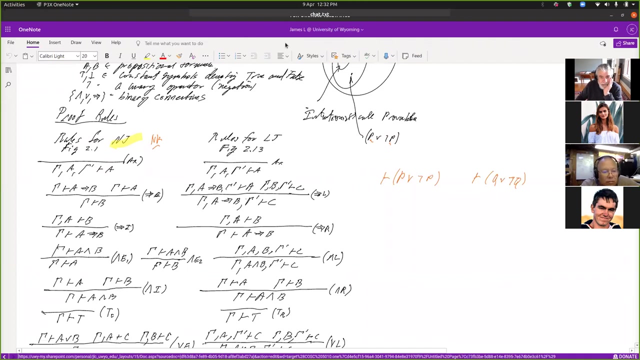 and so to me, you might almost just write down the truth table. it's shorter than trying to write down the proof. um, so let's look at these rules, how these rules work. so i mean, you've already figured them out, but, like this axiom rule is a good one. 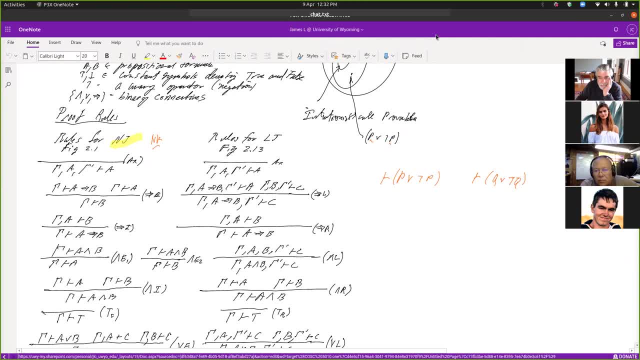 um. all right, see, i could put that up and i could come to draw here. and so the axiom rule is just saying: look, um, um, um. on the left side you've got the formula a embedded in the context. think of gamma as a list of formulas and gamma prime as a list of formulas. 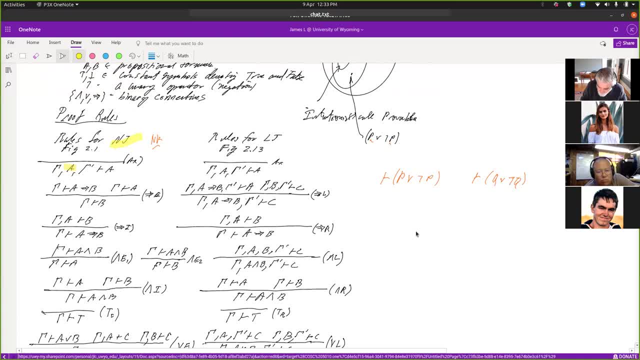 and you could sort of think of um. this form where we write down um, you know, gamma comma, a comma, dash n, is a formula where we write down a formula a with a s in the ending when we go on to the second formula. you see, here's the formula a and s with a s in its ending. where we put in the f in the previous formula, like we put in s and b and s, so to speak, and we're just making a formula as well as we do to the second formula, a and s and b and so on to the in the present formula. 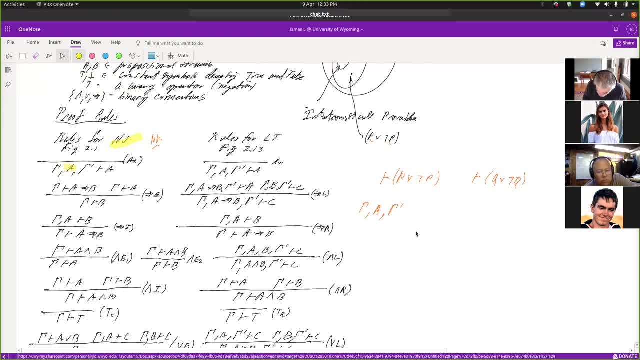 gamma prime, as, if you want to think of this as a list, you could think of this as gamma plus plus a constant to gamma prime, and what this does is you know, it allows you to specify the rule in such a way that you can make an axiom if a occurs anywhere on the, in the context, anywhere. 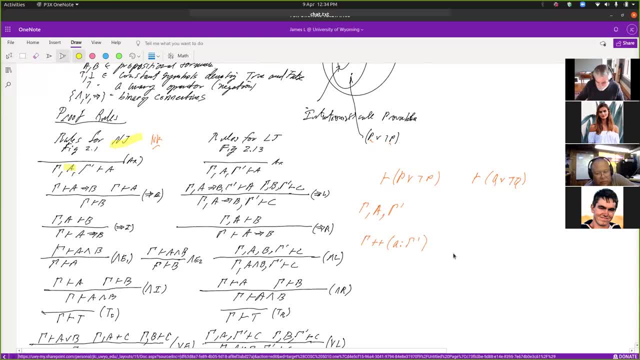 in this list. this just means a occurs somewhere in that list and you could break apart the list and figure out what the part of the lift to the left of a is. and this is the part of the list right of a. Does that make sense? So context is like a list of formulas. that's what the gammas. 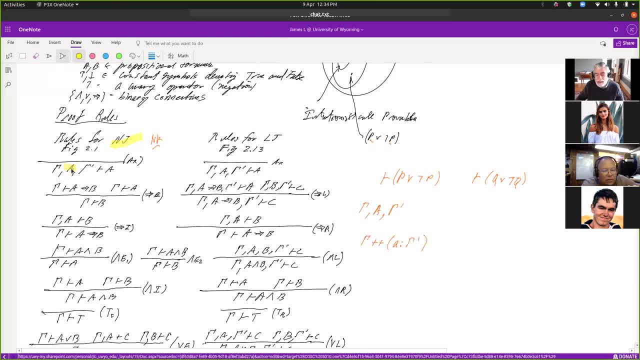 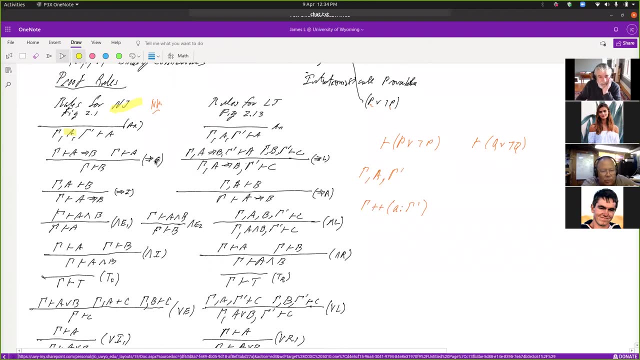 are, and this is just saying: oh, a is in gamma somewhere. Now the rule for sequent calculus is identical in this case, but it changes for the um. so we have elimination rules in natural deduction and introduction rules, and how that gets translated in the sequent calculus is that you have rules for kind of. 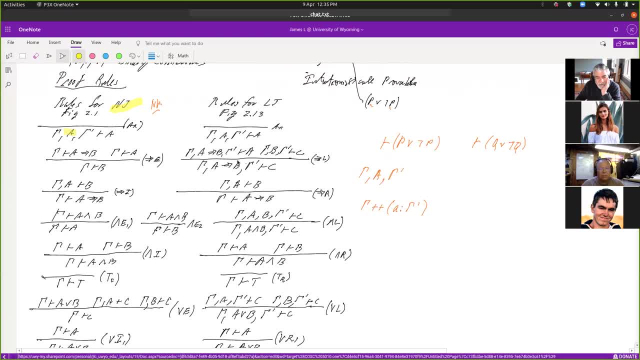 dealing with- oh, you start from the bottom up. rules for dealing with, uh, formulas, complex formulas on the left, and those correspond to the elimination rules, and you have rules for dealing with a complex a formula with a connective in it on the right, and so it turns out that the 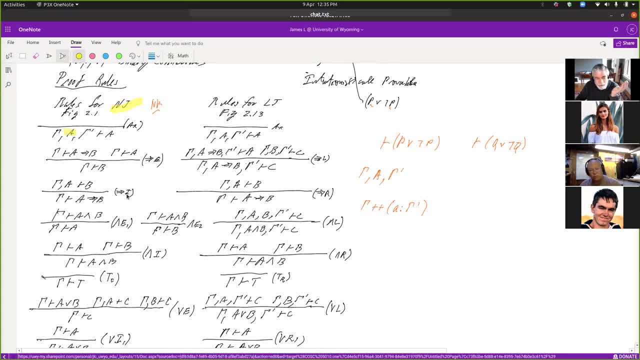 sequent rule is identical to the uh introduction, So um. so this is the uh introduction rule for for arrow, but for the left rule this just says: look, if you've previously assumed a implies b, then um, you can do, you can. how can you use? 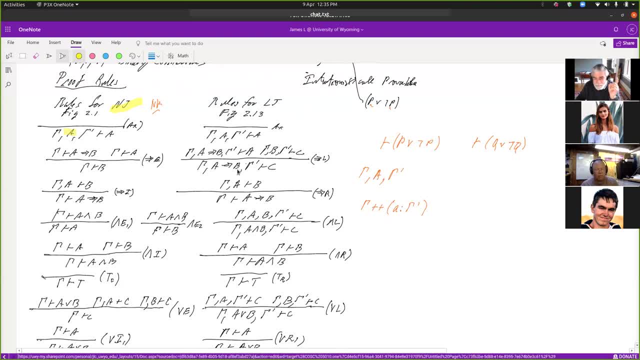 this. You might look and see. look, what I really need is I need. if I had b, I could prove c. So how could I get b? Well, we know from modus ponens: if I know a implies b, I could prove c. 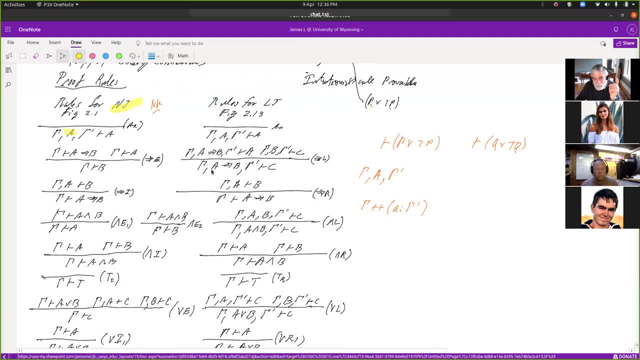 If I could prove b, if I could prove a, then I know I can use b. And so this rule is saying: if you see an, implies on the left, and you want to try to use b, what you do is you prove two things, and maybe this: um, um, I don't know. 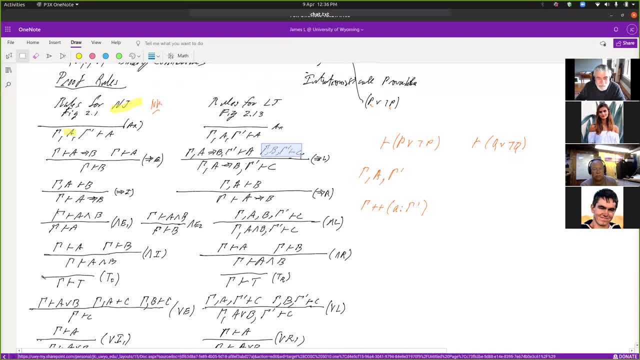 maybe I've got this a little bit like too close. the second sequence: Let's see if that will fix it. Oh God, I I really wrecked it. Okay, Undo, Where's my undo? Can I just type control z? 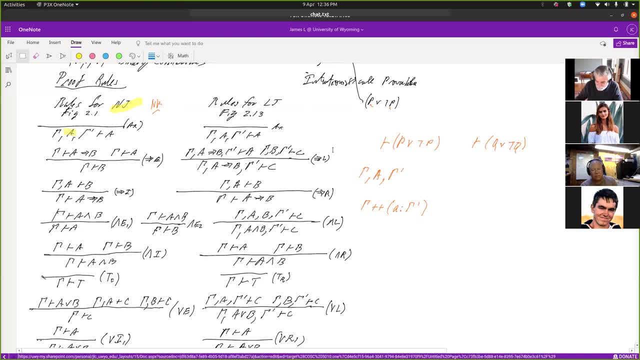 Okay, So what I'm trying to do is show you that this is one sequence over here and this is another sequence over there, right? So it has two things, just like this one has two things. Now, on this one, you're trying to get b See what we say is like: oh, what if we 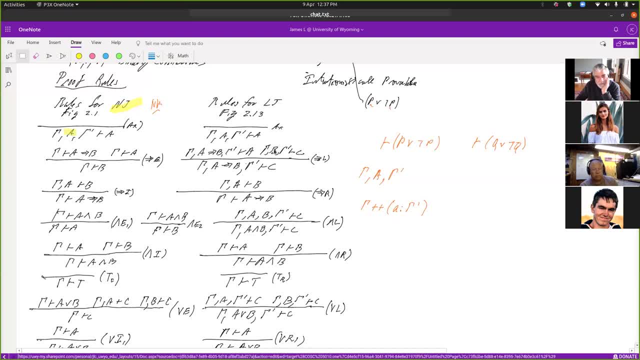 get. we want to use b in some way. So we, after we prove a, after we prove a, we get to assume b and add b to the um to the right-hand side. Now it's very subtle. Getting these rules right is very subtle. 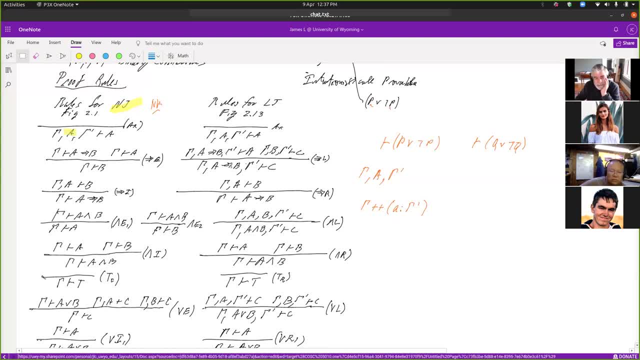 because, notice, on this branch you leave the um hypothesis a in um implies b in the sequent, and on this branch you can get rid of a implies b and just replace it with b. So that's kind of a subtle. 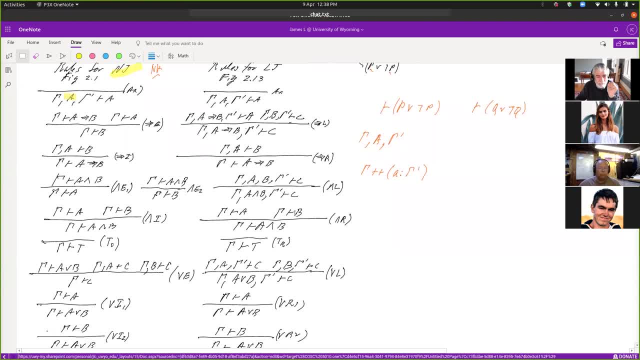 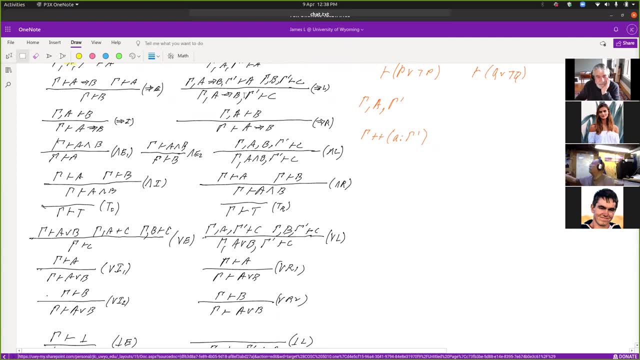 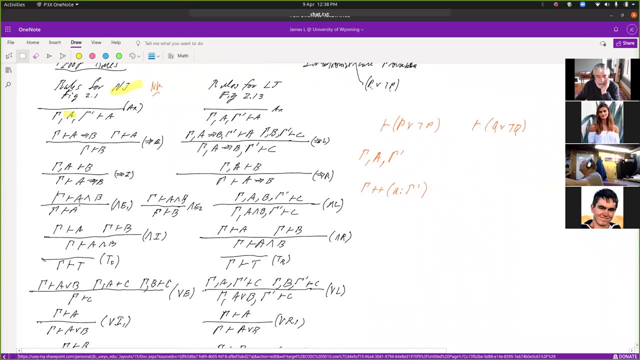 thing that's going on in that rule. Now, the advantage of doing the rules in this sequent form is- and I think the thing that makes natural deduction proofs a little bit more difficult- is that in a sequent proof you can always work backwards, You can always look and apply the rules. 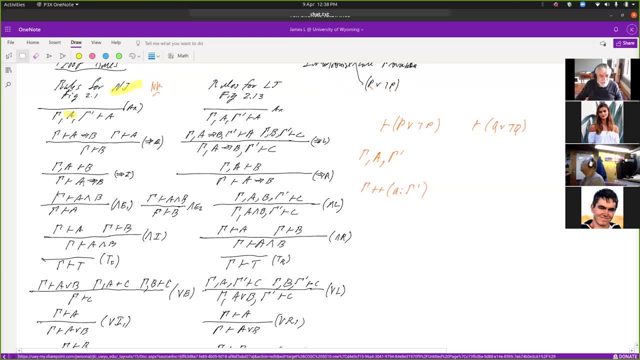 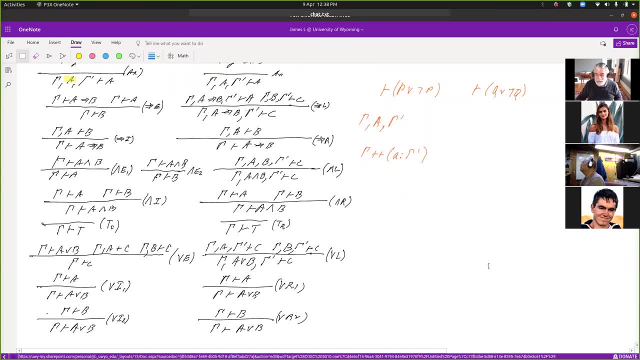 and you just keep working up, whereas in a- um, natural deduction proof, when you get something that you want in, uh, in the context that you want to use, you, you, you write that up above as an assumption, right, You, you know so well. maybe we'll look at one of MemRAM's proofs in a. 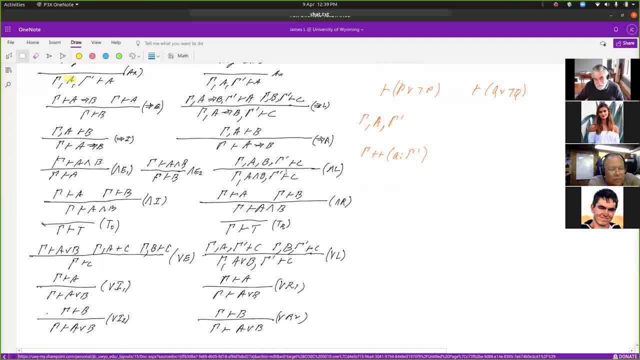 minute, but I don't know. So the AND rules, um the elimination rules, are captured by one rule that says: if you've assumed A and B in your context and you're trying to prove C, just break it apart and separately assume A and seeingbeiten. 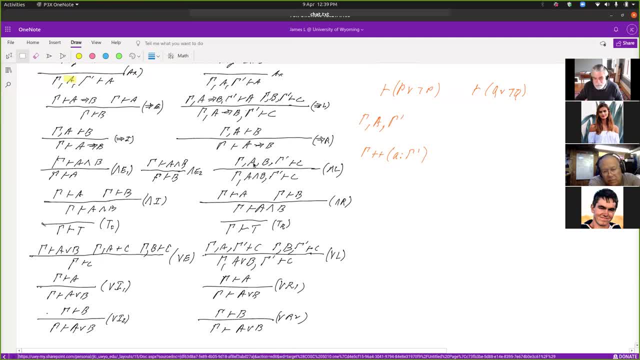 and you're trying to proves C. just break it apart and separately assume A and seeing jealousy ret primered 友. and separately assume A and seeing jealousy ret. primary statements board with the structure on creating nous. interpreter of perfect critical thinking on房s. 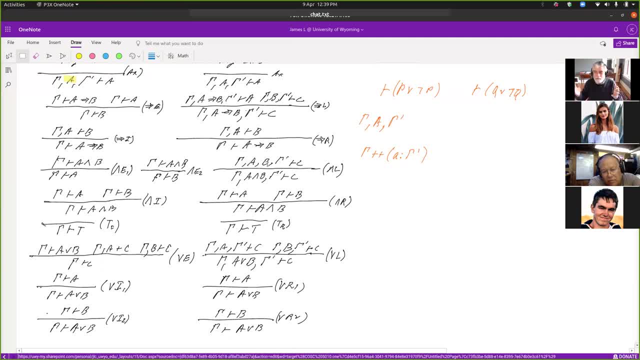 separately. assume B. If you've assumed A and B are true, you know that A is true and B is true. So the things in your context are the parts that you've assumed to be true. And if you assumed A and B, then you know A is true and you know B is true. So that's kind of the soundness of this rule. 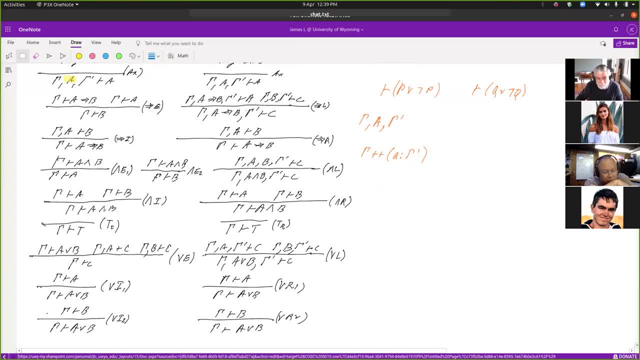 informally Any questions? I mean, that's what these rules are saying. They're saying like: okay, if you've proved A and B, then you proved A, You can get A, And on this one, if you've proved, 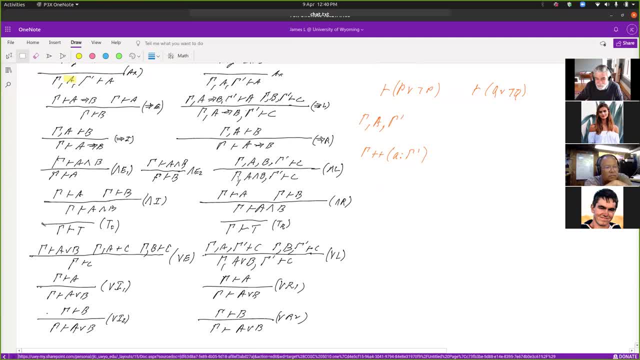 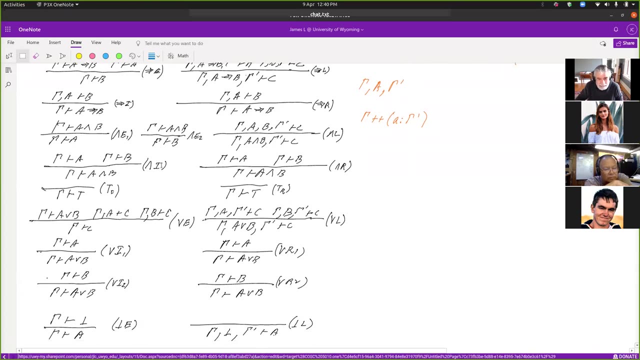 A and B, then you know B is true. And so this one's working backwards says: if you've assumed A and B, which means as if you've proved it- then you can assume A and you can assume B separately. Now the introduction rule is identical: You have to prove A and you have to prove B. 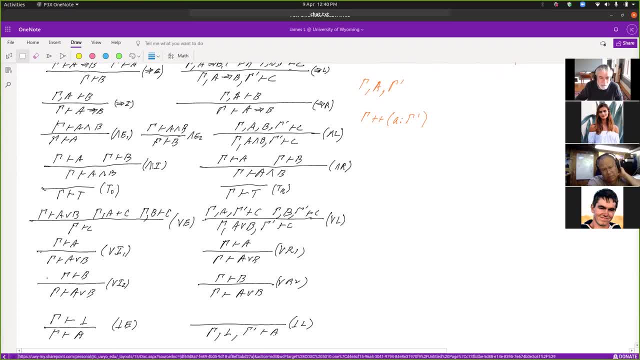 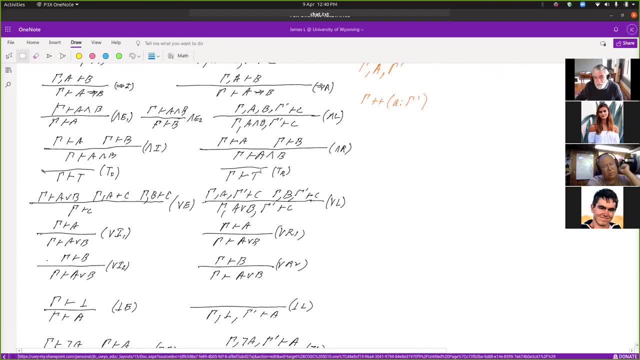 You have to prove B before you know A and B, And that's true for the introduction rule and the and on the right rule. So these rules are all meant to be used backwards. And and on the right means you're trying to prove something that looks like: this gamma turns down A and B. 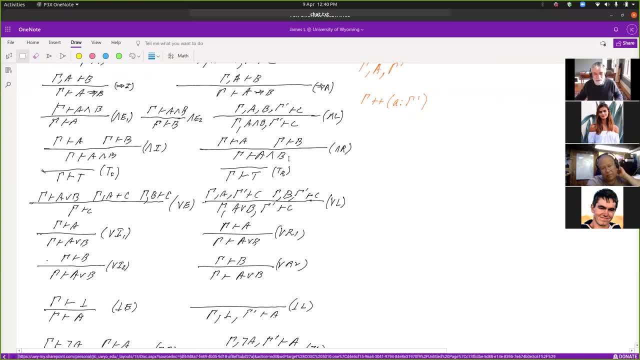 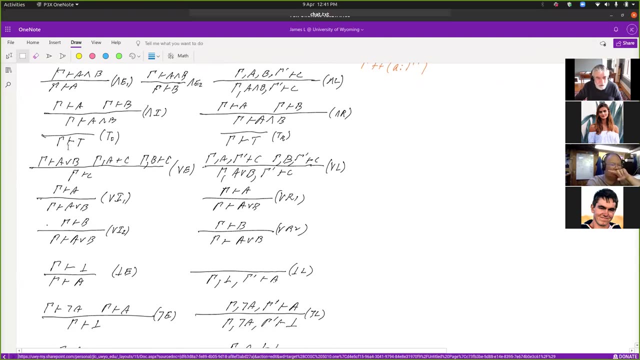 Okay, How do I complete the proof? Unless you have A and B over here, you're going to have to work on A separately and prove B separately. And that's what this says. Exactly the same thing. Now the true. what does he call this? 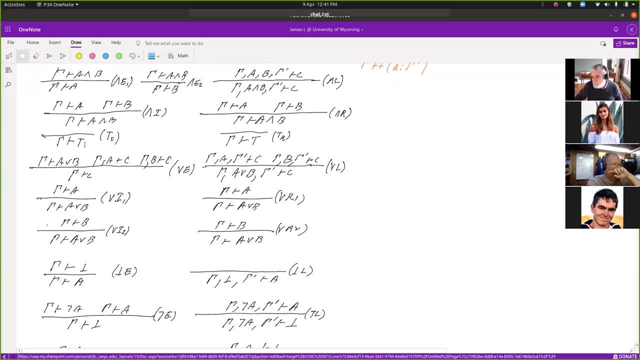 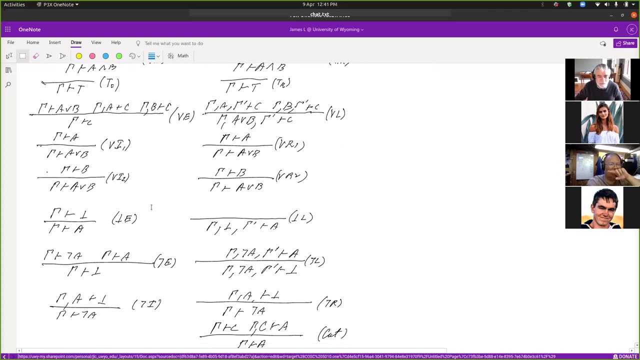 A true introduction rule. True can just be put on the right of turnstile And over here you have a true right rule. It's always okay to put true on the right. This is an axiom, And this is an axiom. So if you need true, you can just write this down. 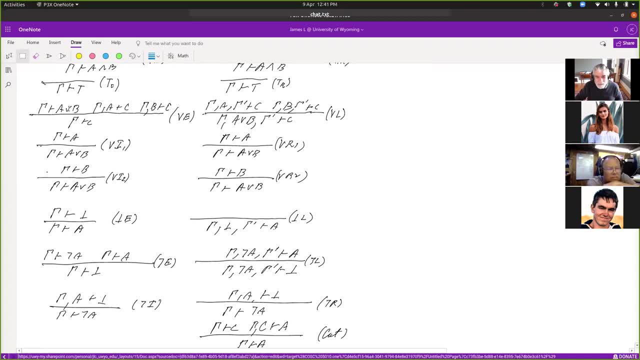 So then, on this rule, the or rule is kind of the most painful rule to use, And so this, the way they're saying it here, is if you could prove A or B, And that is the same as having assumed A or B. So I'm trying to show gamma one. 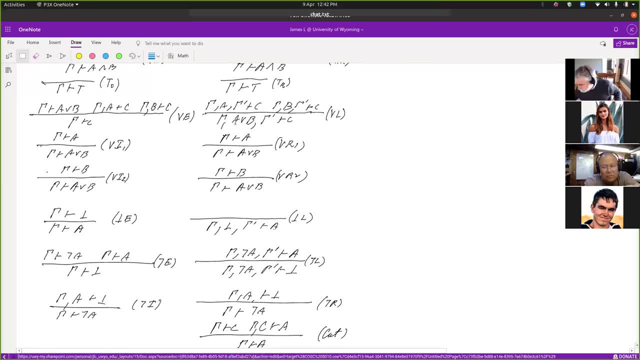 And I'll be back In a minute. And then it seems to me that when I went and solved that thing at the beginning of class, I did it by taking the implications and appending them to the end of the list. Yeah, that'd be another way to do it. 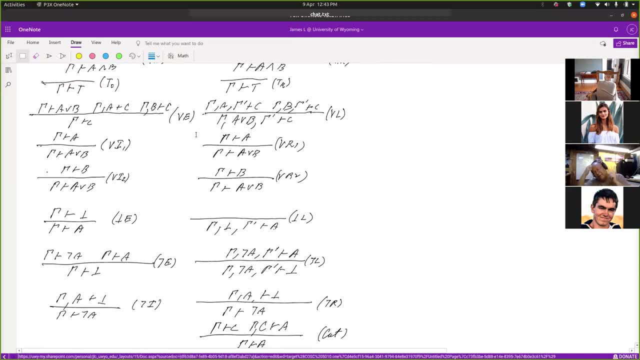 Yeah, which it looks to me like when I looked at that, that the the thing with the implications was that not only do we want to have the implications at the end when we add them to the end of the list, But the reason why we get some of these weird results is because we've, instead of proving things in no time it the process in OCaml or Haskell actually has this hidden behavior of time that we're adding to the process. 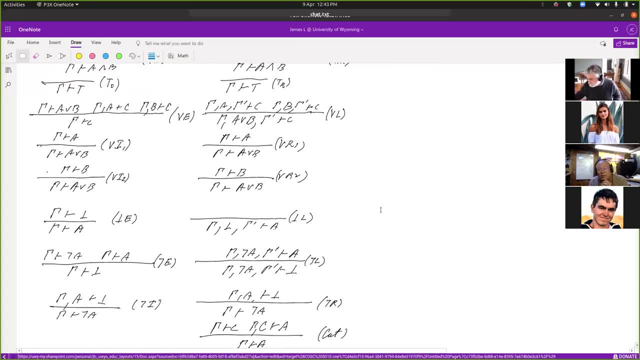 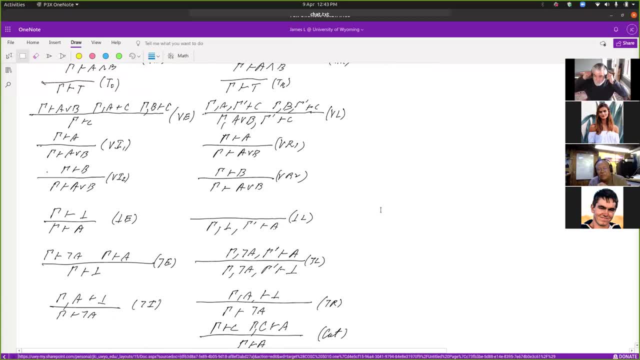 Does that make any sense to you? Things are happening sequentially instead of, you know, all in parallel. I didn't hear the question. Oh, I was talking to them about the home work, So this wasn't directly related to what you were working on. We came up with different. 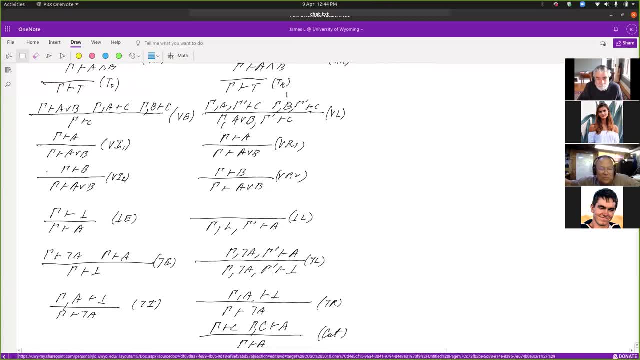 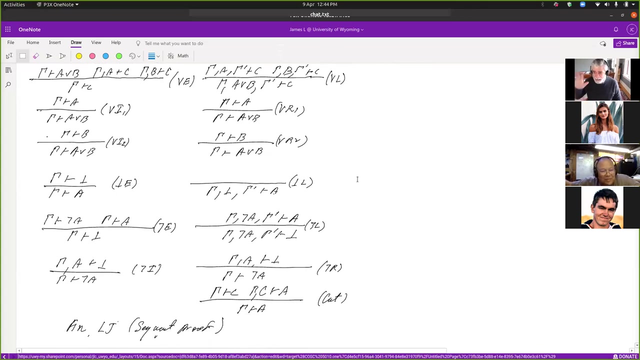 ways of solving the same problem. So here's- oh, excuse me, Maybe let's take a five-minute break. Yeah, let's take five, and we'll all be better. And maybe Finn will tell me that I'm crazy for what I'm thinking. There we go. 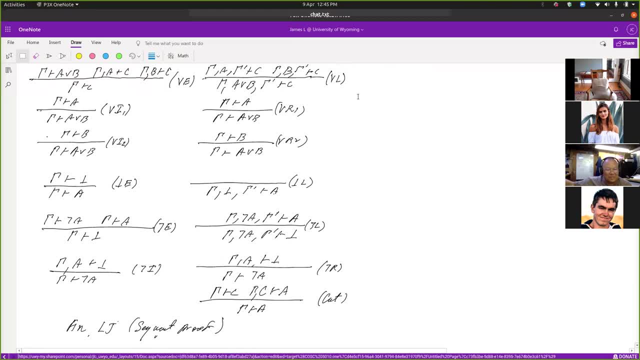 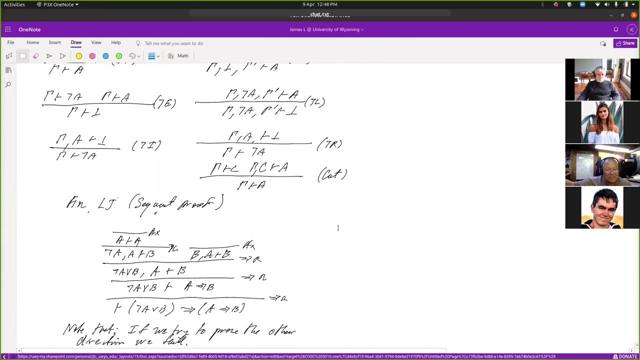 Thank you, Thank you, Thank you. 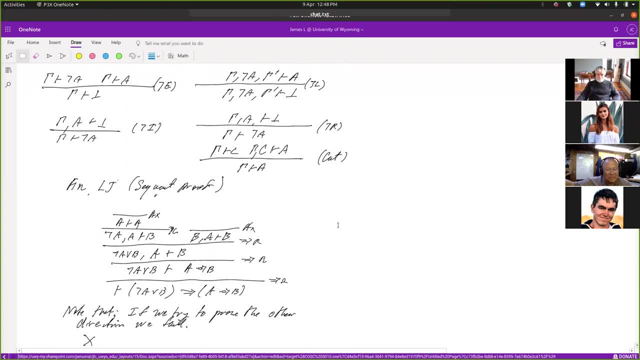 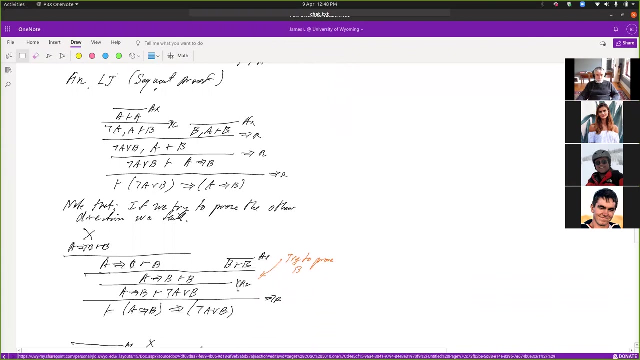 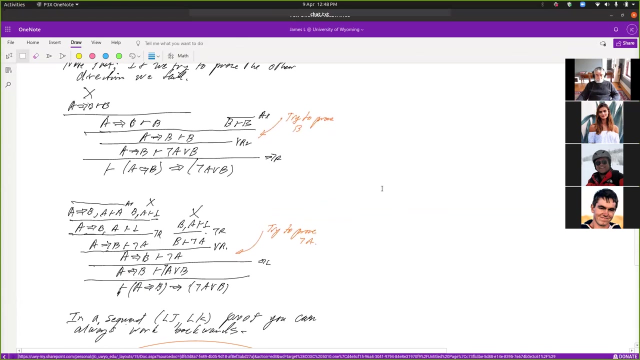 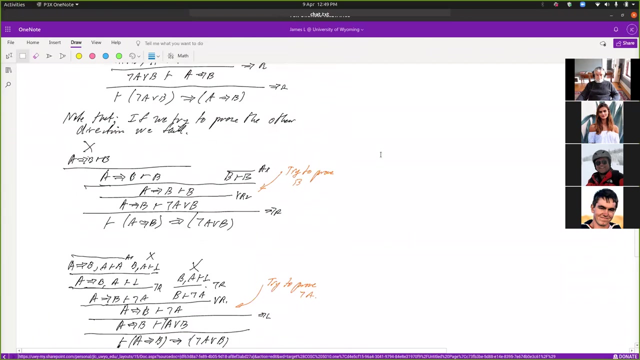 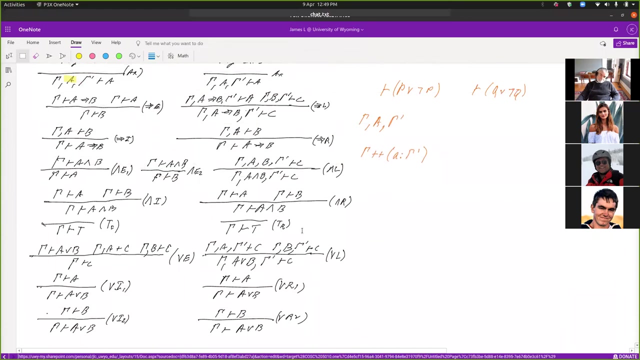 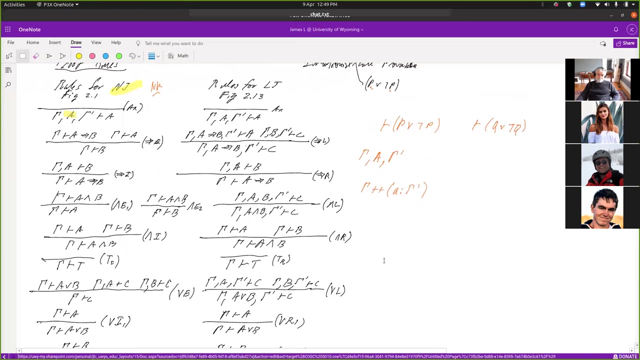 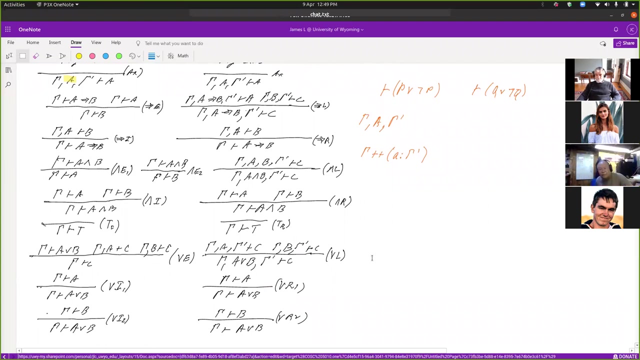 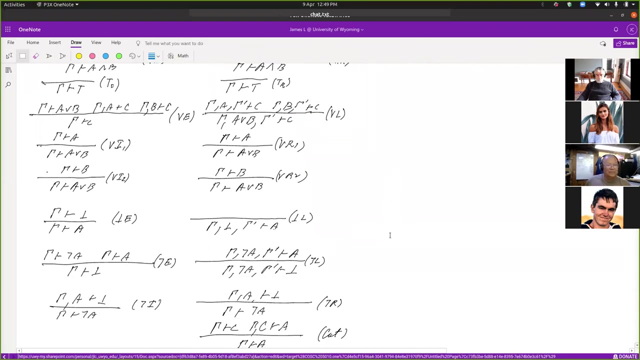 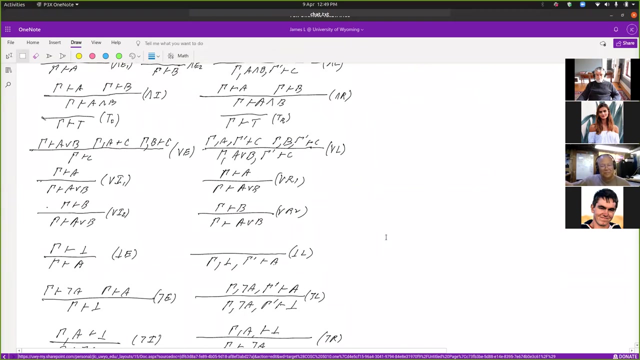 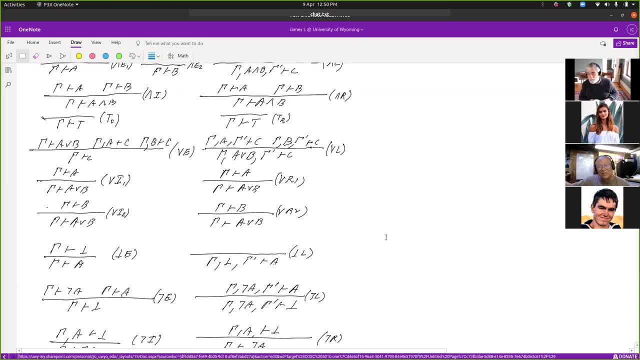 said he got me some food and it was before class and I ate it, not realizing that it was really spicy. And it was just when class was supposed to start and I got the hiccups. And then somebody else hiccuped in class. 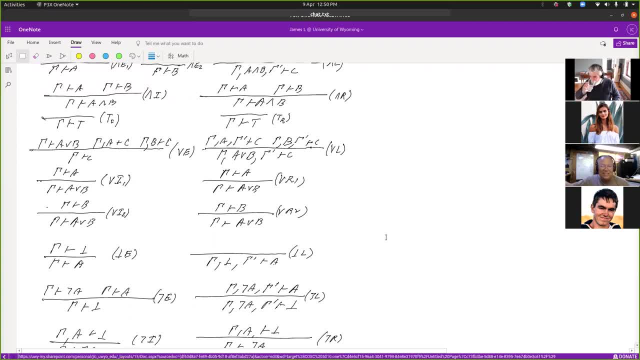 and this was before the pandemic, and I said, see, the hiccups are catching, and I had to leave the room for a couple minutes. Man, my face was red. It was so spicy. Wow Yeah, I had to leave the room. 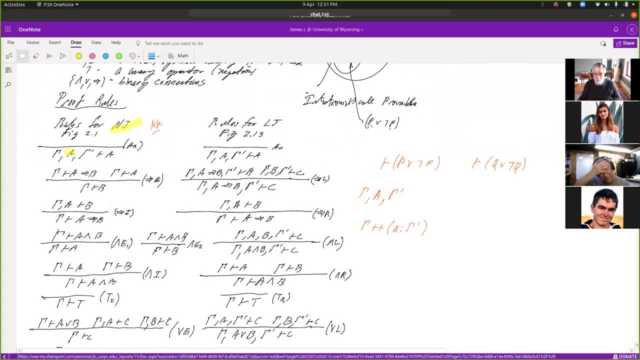 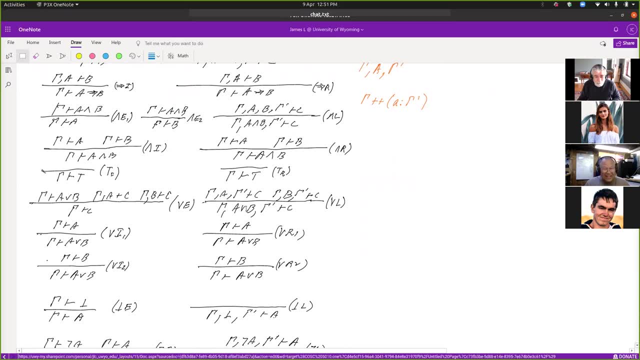 and go get some water and come back and I started class a few minutes late. But I don't think I would make that same joke today, but these things happen. Oh yeah, Yeah. it's like, ah, the world just impinged upon what I'm trying to do. 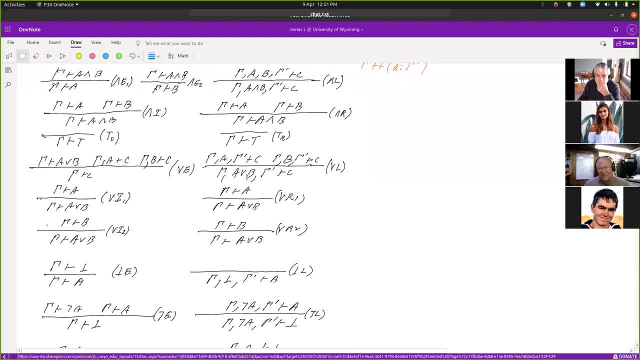 and it just is. It could have been a lot worse than just hiccups if it was really, really spicy. Oh yeah, It wouldn't go down that way. Well, this person is. I've had her food before and I usually eat spicy things without trouble. 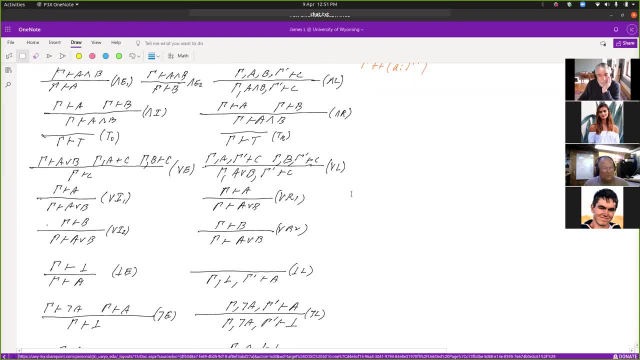 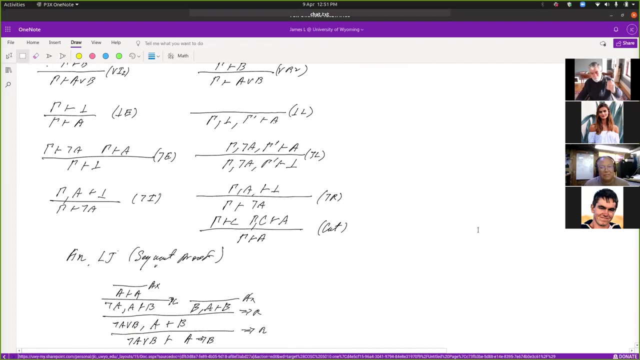 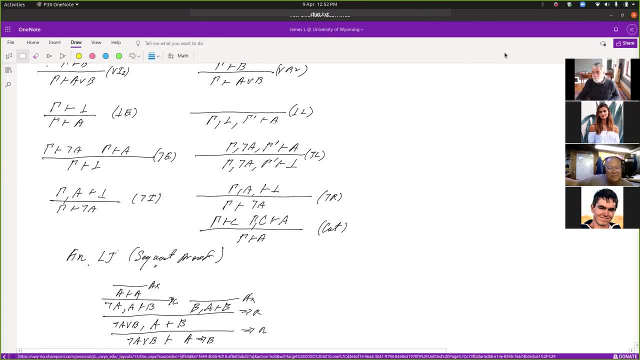 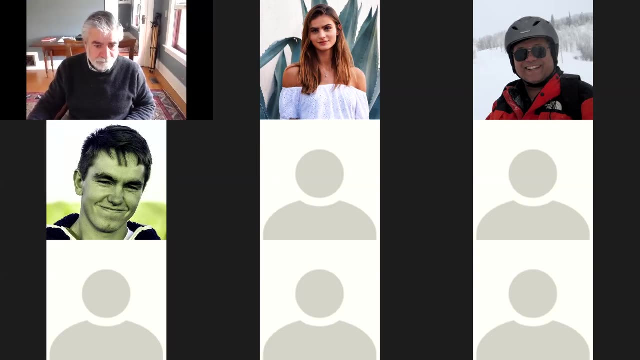 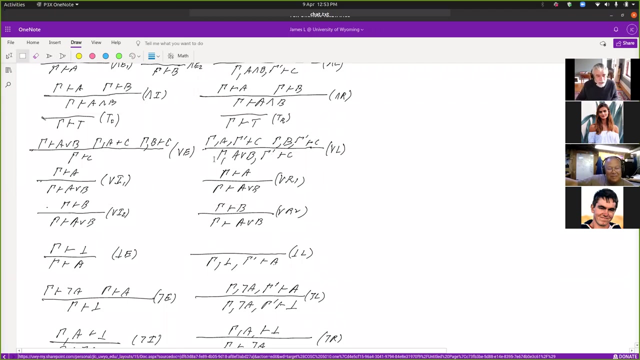 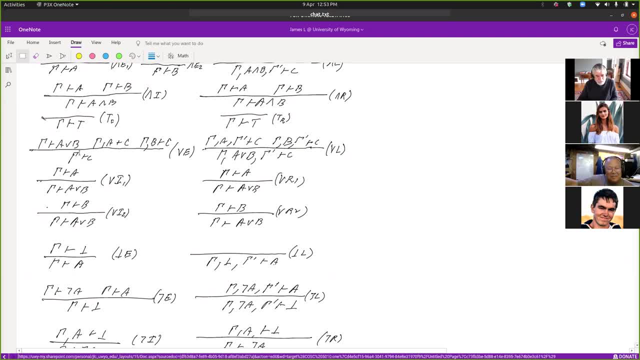 Is intuitionistically. you know you have to if you want to prove C and you know A or B. what do you know if you know A or B? You know that A is true or that B is true, or maybe they're both true. 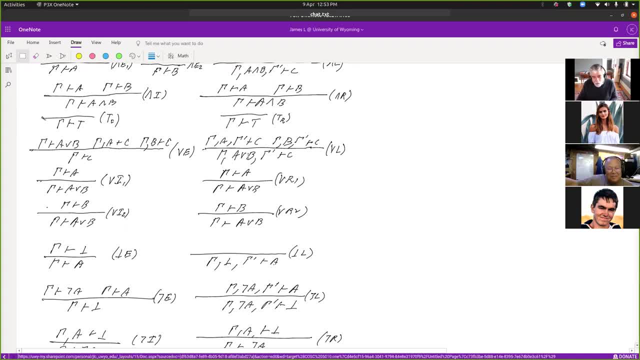 So that means you don't know whether it's A or it's B. So if you can prove C from both the assumption A and the assumption B, then you've covered both cases. Now, if you don't need to use A or B to prove C, 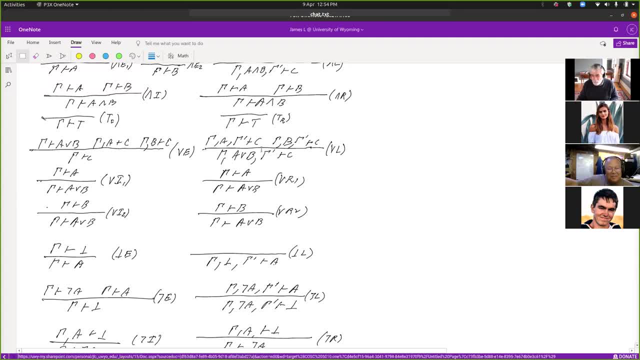 you could just skip this. You don't need to apply this rule. And if you prove A, you can prove A or B, and if you proved B, you've proved A or B. and those are the same as the rules for the right rules for the sequent calculus. 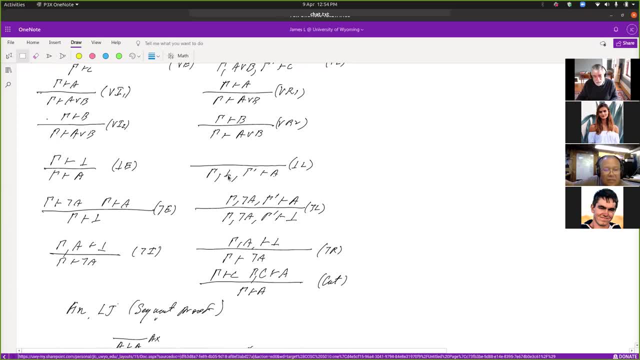 In the sequent calculus. if you've ever get bottom false on the left, you can prove anything. So this is an axiom Here: if from A you can prove, you know if from bottom, if you're going forward, you could say: 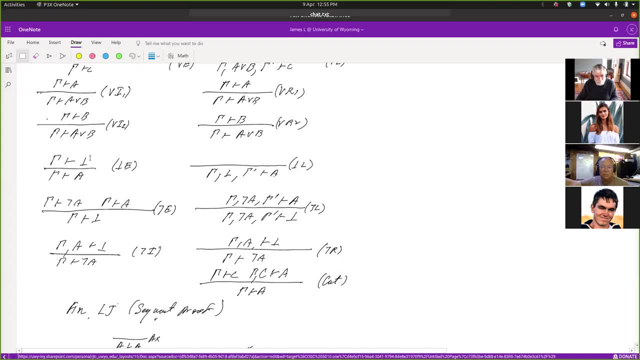 if I could prove bottom, I can prove anything. so usually you're using this one in a forward direction. you've proved bottom and now you're able to get something that you want the rule for not. it's kind of interesting now. one thing is, we don't need not because we can describe. we can define that and usually 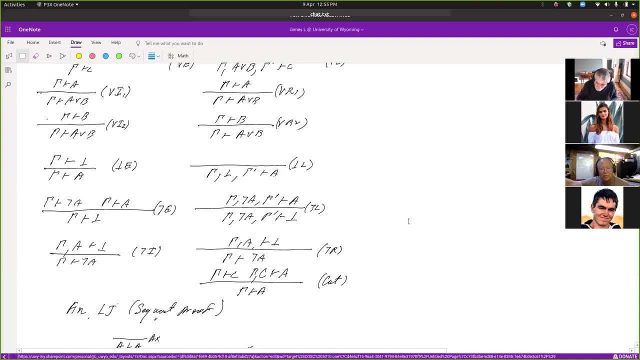 you do, you could say not. a is by definition, a implies by a implies by bottom. so if you have the bottom, if you have false, you don't need not. and if you look at these rules, you can see that these are what he called someplace else. 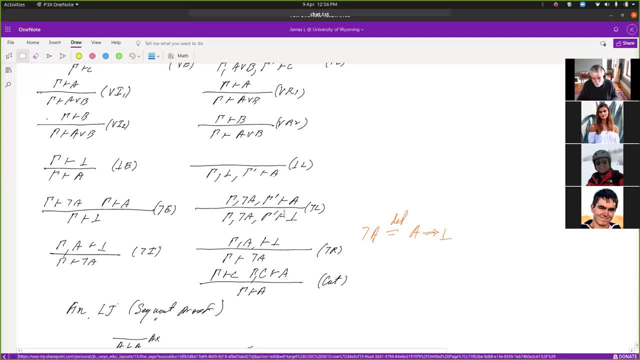 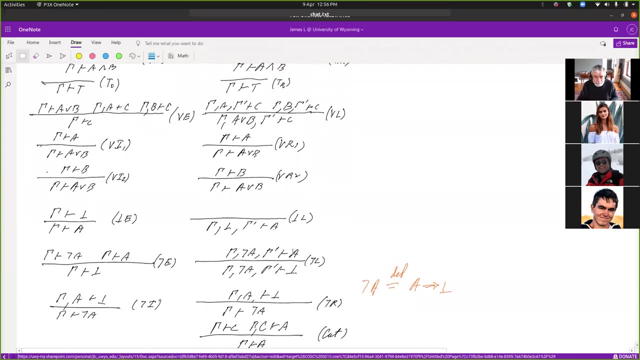 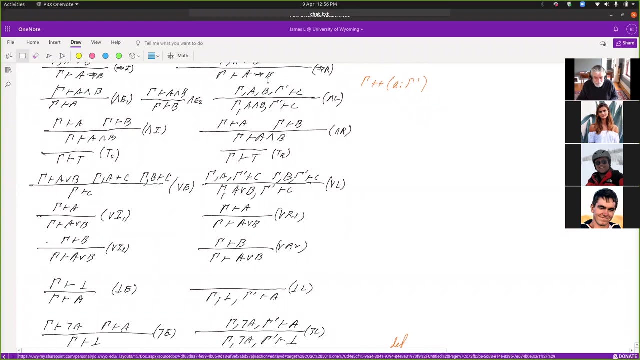 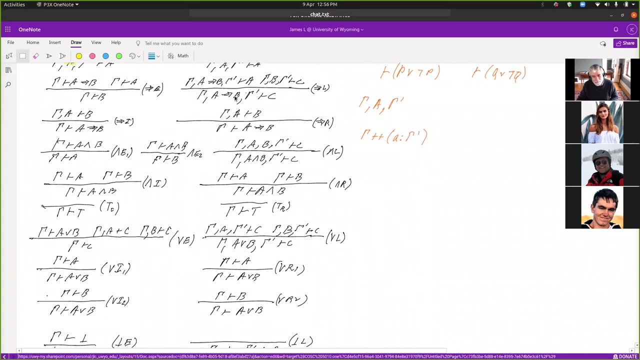 admissible rules we could derive the rules for not. if we interpret a, not a, as a implies bottom, and you can see that, like I'm gonna be able to get it, no, it's just out of the range. so here's the rule. so if you have a implies bottom on the left, then if you can prove here this: 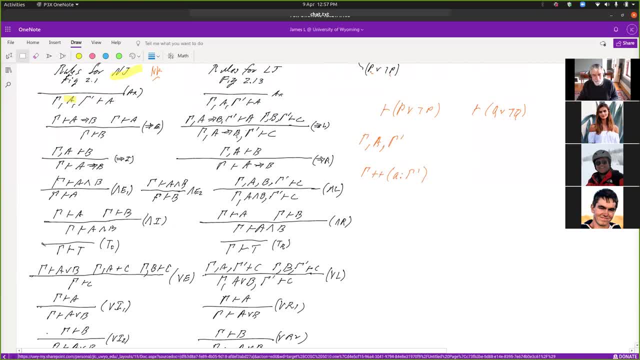 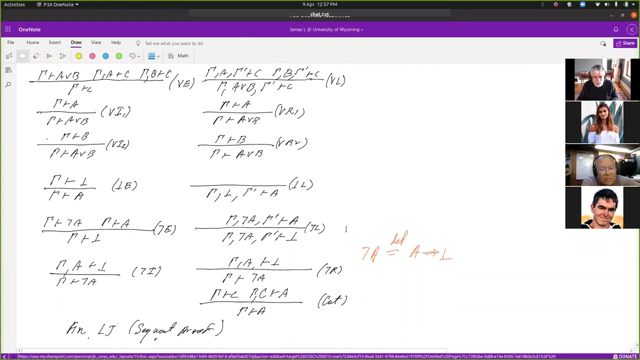 will disappear only if you can prove less to this will disappear. right, because you will assume bottom. and the bottom axiom says: if you have, if you assumed bottom, then you know you're always ok, and here you try to prove a. so if you look down here at the bottom, ruleない. a and you say, okay, if you know not a, then if you can prove a, you know. if you're not, okay you're right. but if you have no crime, then you can prove that a will be okay. and here you try to prove a that if you look down here at the bottom, roll you. okay, if you know not a in the rule that if you don't leak a rule, if you Hosanna, okay. so let's play one more argument. okay, let's try to prove a by using this to really, because of course, aa didn't prove anything in this particular quarter in the rule. 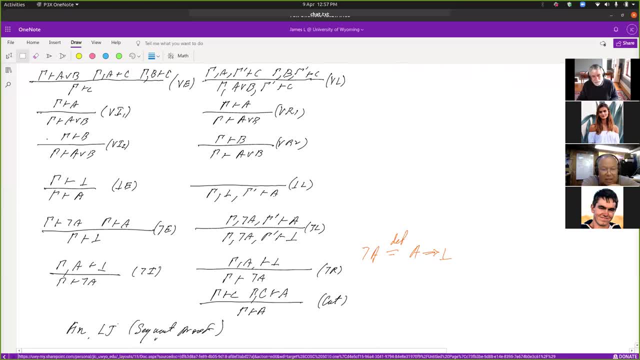 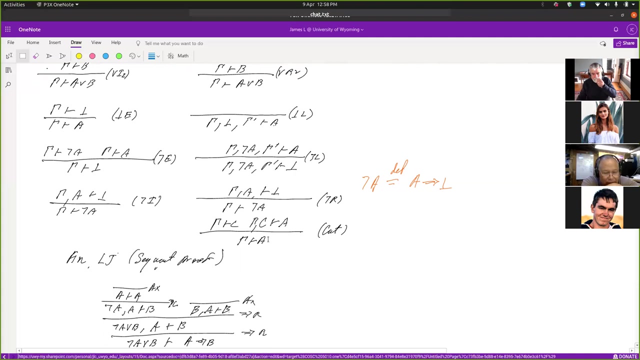 and you're trying to prove bottom. you can try to just prove a and similarly here. this is exactly the implies on the right wall rule. if this is a implies bottom, then what do you do? you assume a and you show up and here's a cut rule. 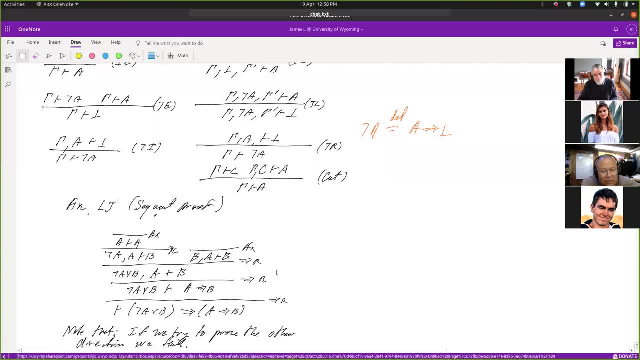 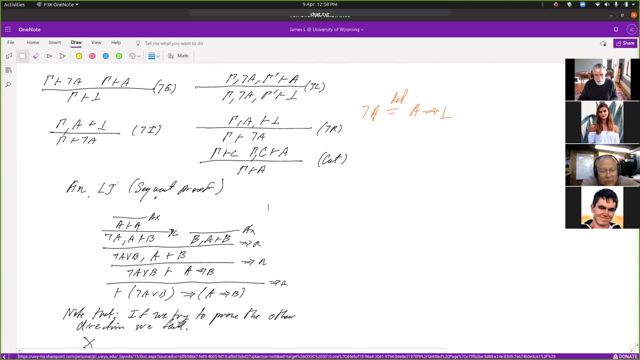 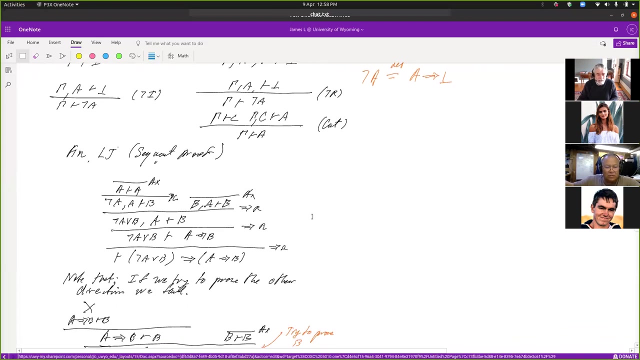 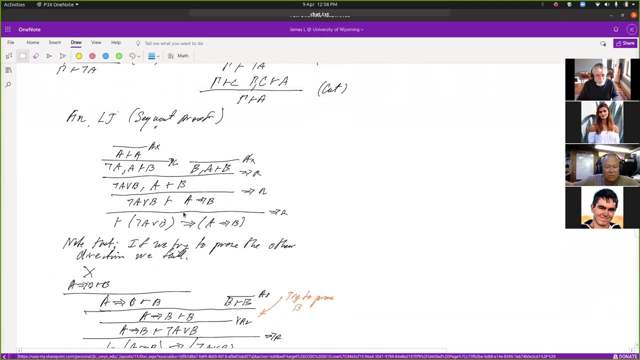 if I can prove the cut formula, see using gamma, using their current context, then I could prove a use. I can assume C. if I can prove C, I can assume it, and that might help me in the proof of a. so all right, let's look at some secret proofs, like this one's in the book he does. 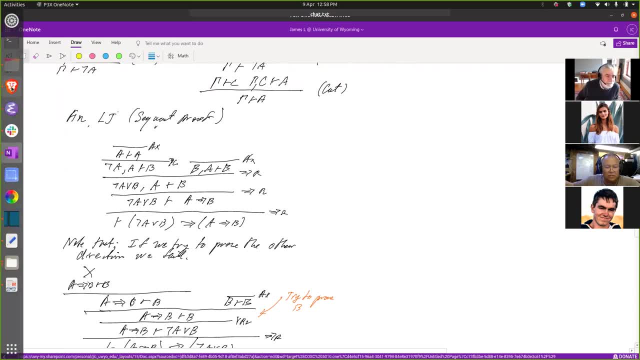 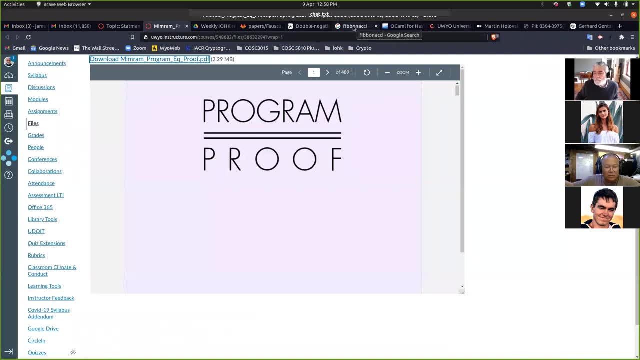 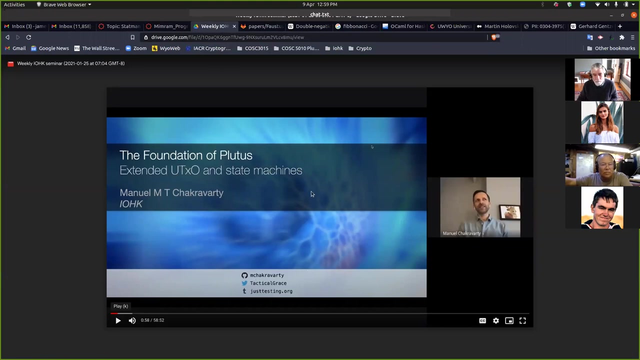 look at some secret proofs like this one's in the book. he does look at some secret proofs like this one's in the book. he does a bunch of them almost right away. I thought I brought this. well, this looks like an interesting talk. has anyone watched it? he talks about why. 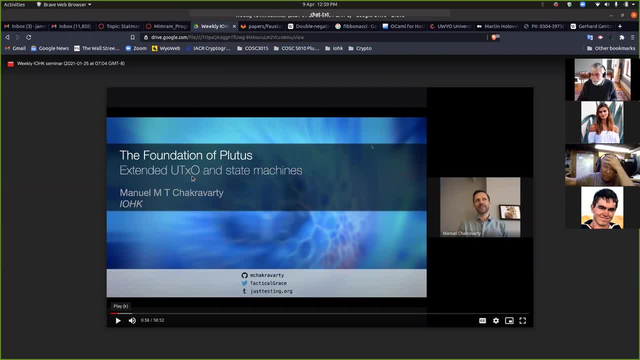 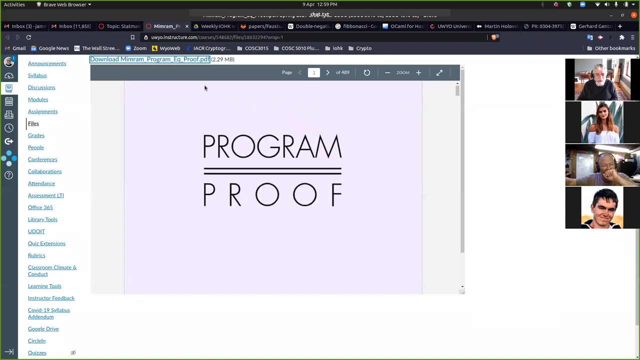 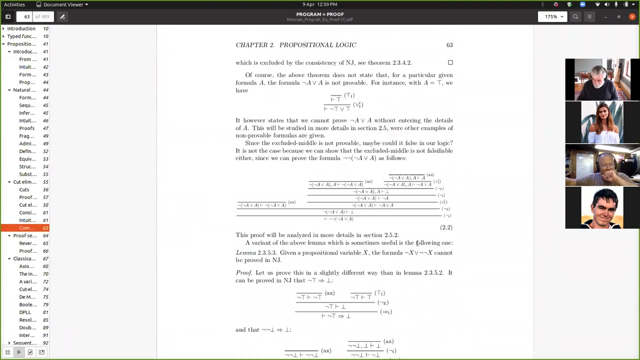 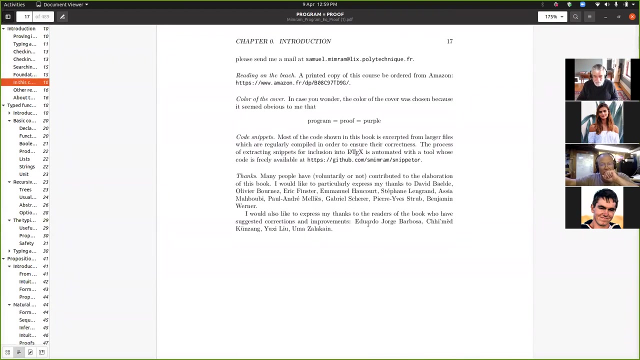 the UTXO model is actually more functional than the Ethereum separate accounts model. I don't know why I have. I need to watch that, so anyway, let's see. I somehow I did, I lost. oh, it's it over here, so let's go look after he at the point where he memram um, presents the rules. 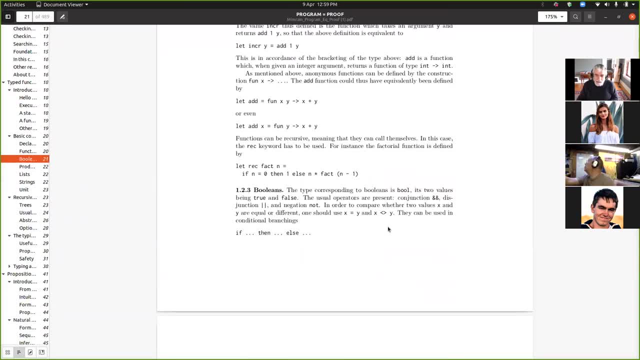 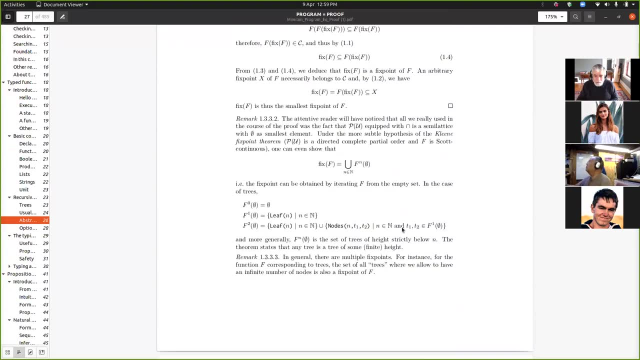 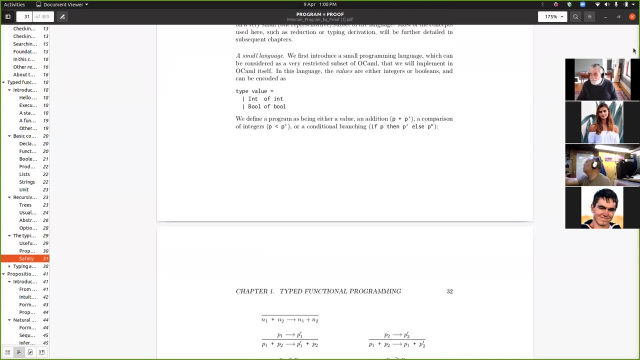 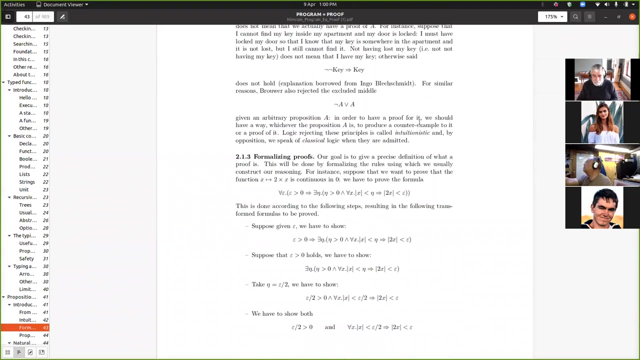 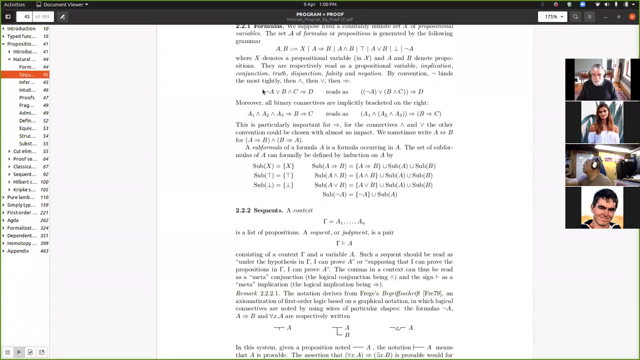 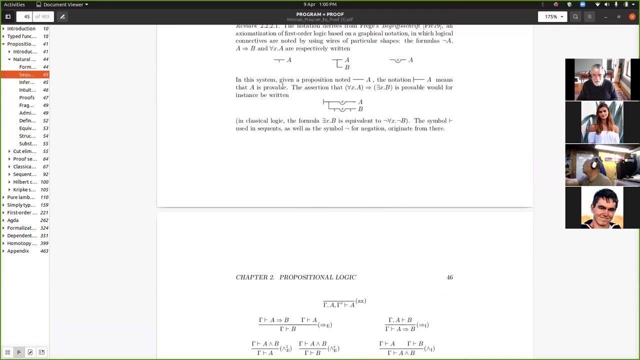 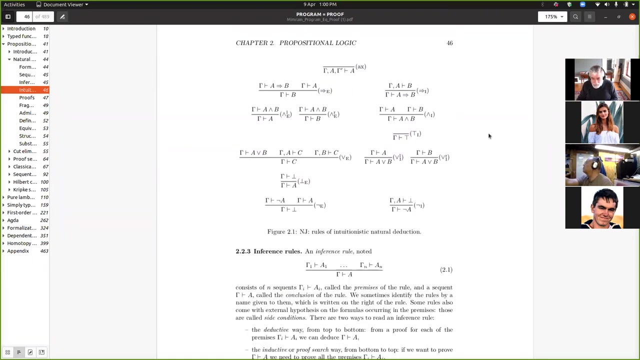 right after that, he gives you a bunch of proofs, and the thing that's interesting is that: oh, come on, where are you? okay? is that? um? okay? he gives the language. um, he talks about sequence. he talks about Frege's notation. that's amazing, um, here's his. 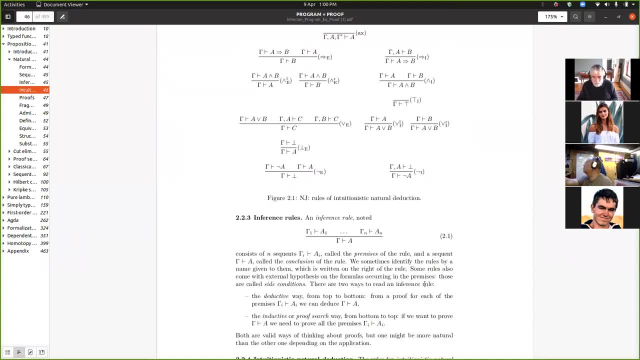 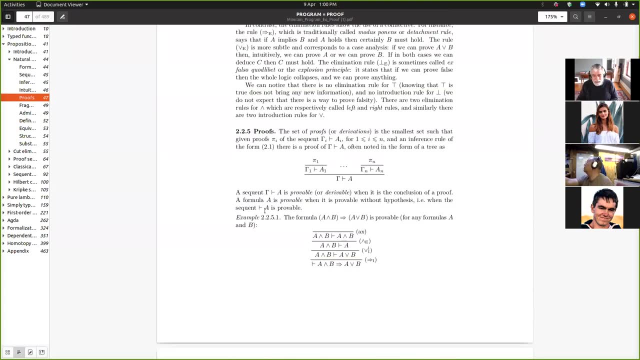 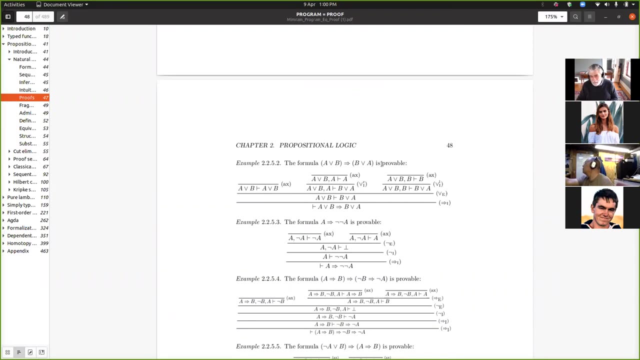 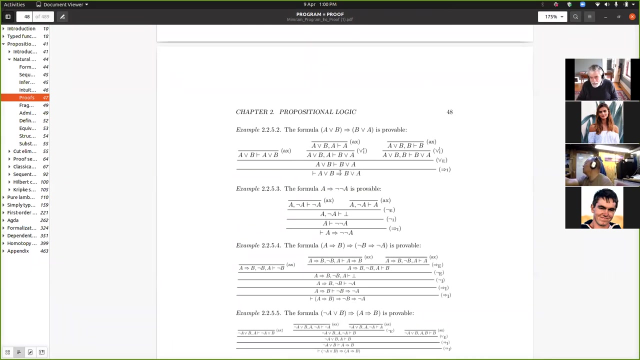 rules that we just looked at, compared to the sequent rules: um. and then he proves some facts like, okay, A or B implies B or A. all right, that one's easy and that one is um, but still um. you're kind of like um, you take this assumption and then you have to kind of like work, for now you're working kind. 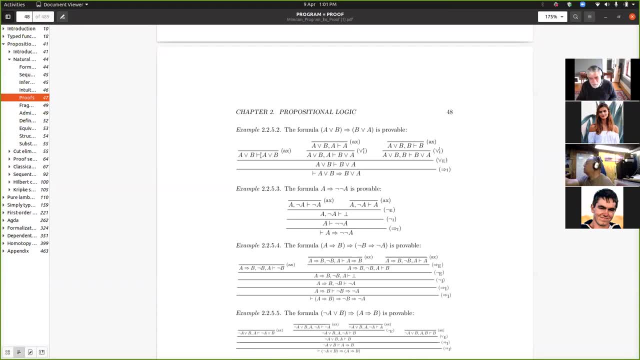 of forward. you say, oh okay, if I want to use this assumption, how do I put it on the right? well, I can put it on the right because I've assumed it. but then what do I want to prove? my C is B or A, and here I get A to prove it, and here I get B to prove it. 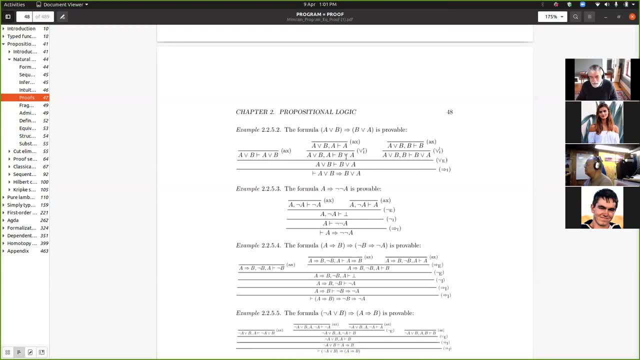 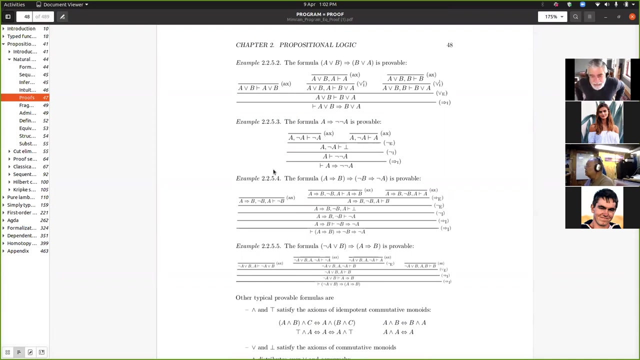 from this assumption, But I still have to then go in and work forward from the axiom that, okay, A is provable because it's been assumed on this branch and B is provable because it's been assumed on this branch. Now, this one is kind of a key thing. 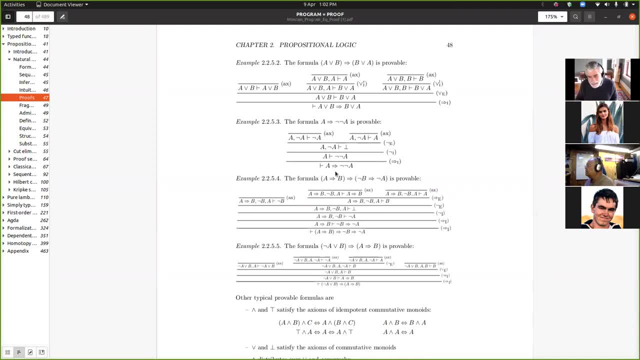 is that he's showing you a bunch of This. one is an if and only if. obviously It's just saying or commutes, But here this one is only through this direction, whereas in classical logic not not. A implies A. 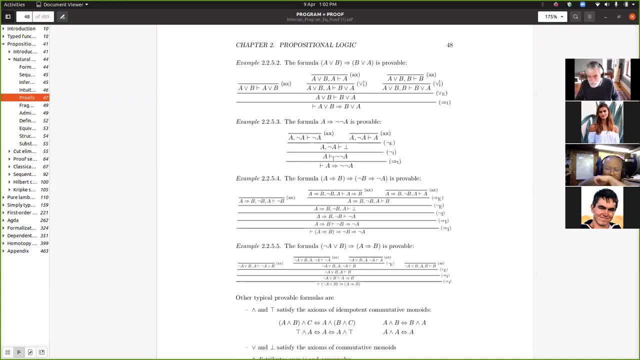 And so here's the natural deduction proof, And let's look at what a sequent proof for this might look like. Let's see, I think I can just annotate on here. Well, first I should maybe make this just a little bit smaller. 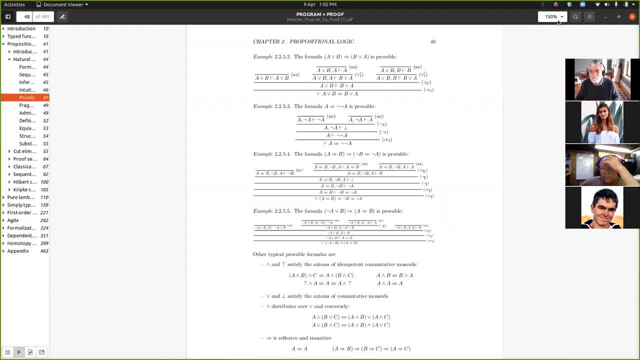 so I have more room, And so what does the sequent proof for that one look like? Well, I need my Wacom tablet to do it this way. All right, let me see. Let me go back over here. I don't want to. 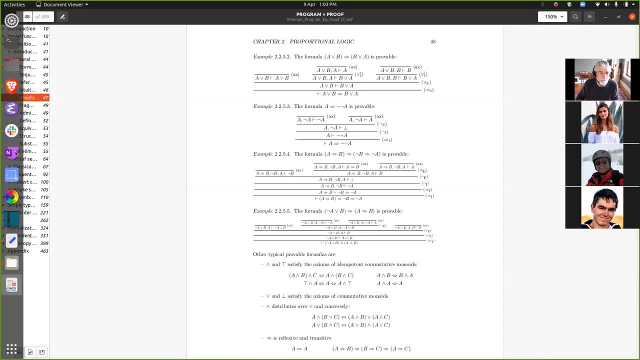 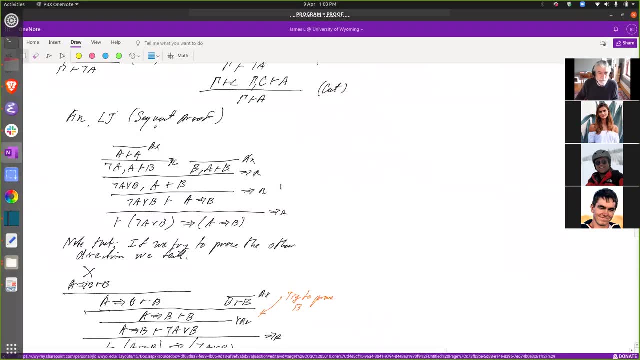 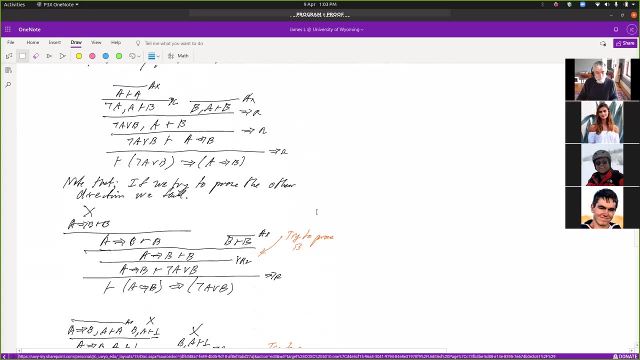 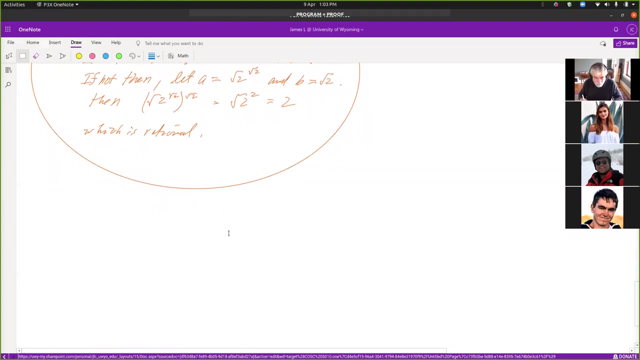 I don't want to. Oh, I guess I got to get rid of that. Okay, So let's do a different one. Let's go down, We'll do, Let's see, Don't know. Okay, Turnstile, Turnstile. 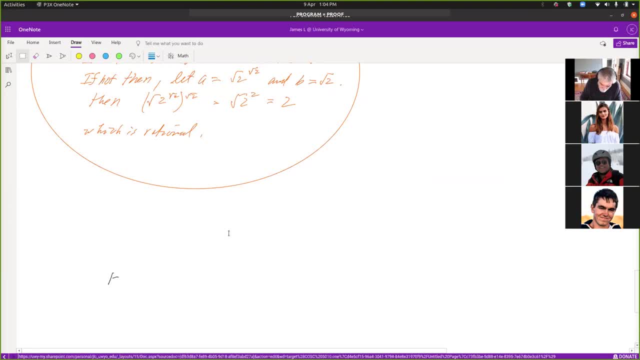 Turnstile: A implies not not A, And so the implies on the write role just says: okay, assume A and show that not not A, and then you just put the unavariable on there And so that implies saying that not, not A. can you see them? 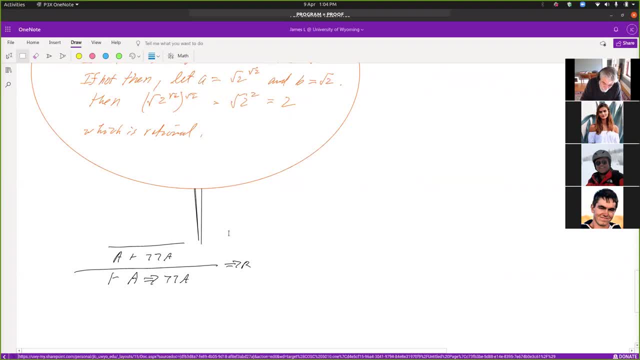 knot on the right roll. whoop, what's it doing there? The knot on the right roll says: take this formula and flip it to the other side. So I put knot A over here. Oh god, my nose is just running like a. 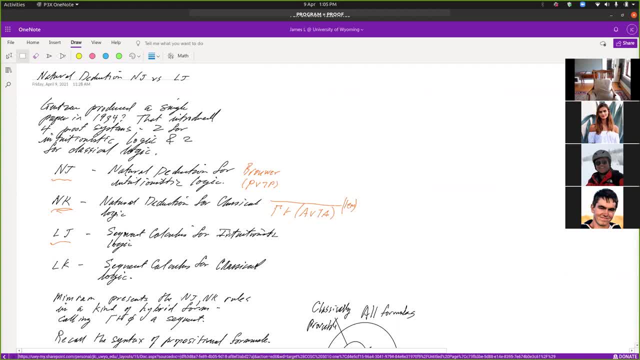 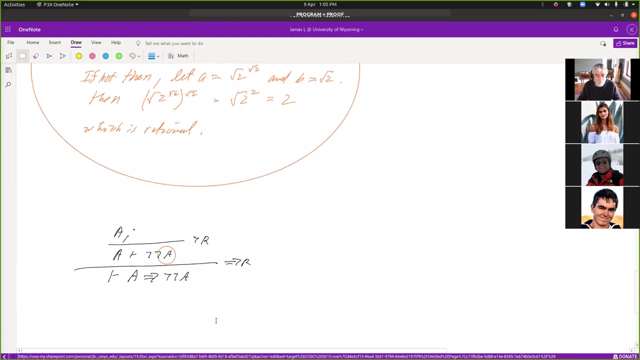 I can't open them. No, no, no, Okay, I think I'm back, Oh god. So the rule for knot A says: okay, put knot A over here, and now you got to show bottom. And now, if we go up, 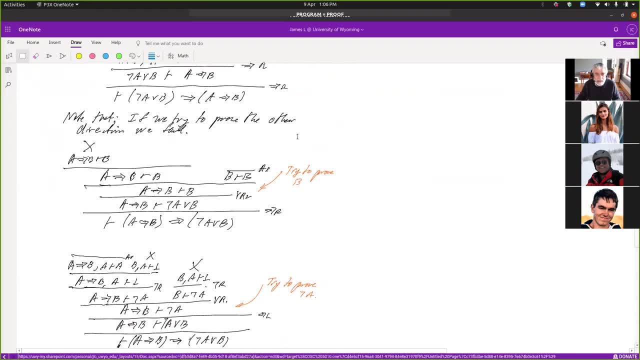 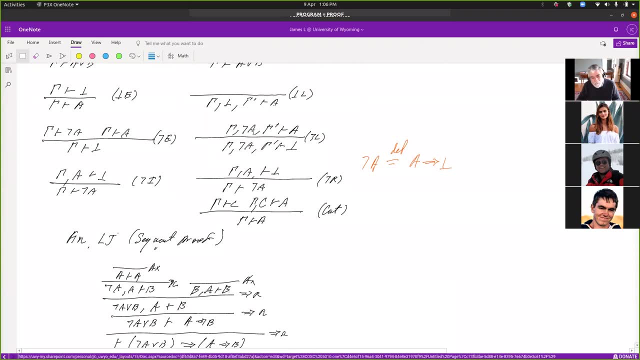 and look at the rule for knot on the right, on the left I mean this one. it says you can throw, you leave the knot A there and you throw the A over to the right. So if I'm trying to prove bottom and I have knot A in my assumptions, 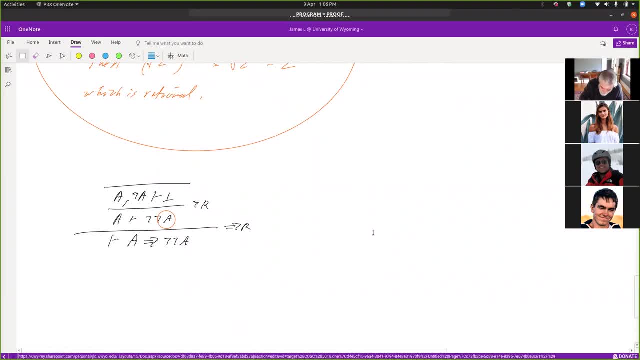 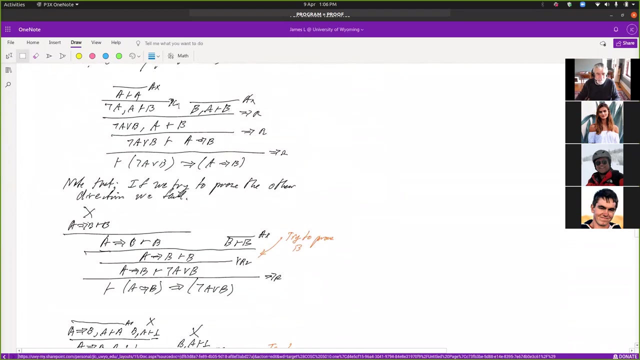 And I'm trying to prove. I'm at bottom and I have knot A in my assumptions. I can do this And then that's just an axiom. Now I think that this is so much easier to do. You just always work backwards. These are- here's a sequent proof. Now, this one's kind of I 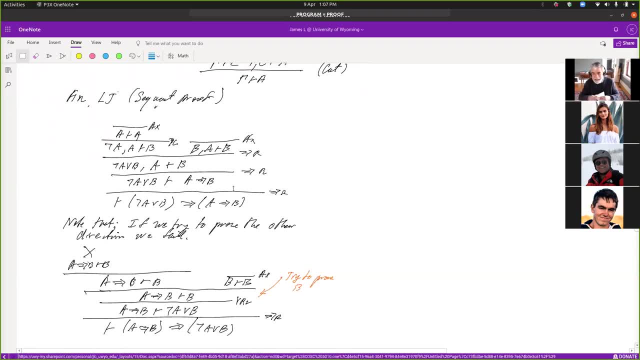 think you know. I don't know if you can see it, but this one explains something about intuitionistic logic that's very important. In classical logic, not A or B is true, if, and only if, A implies B is true. Right, We could- I mean, you know, we could- do something really. 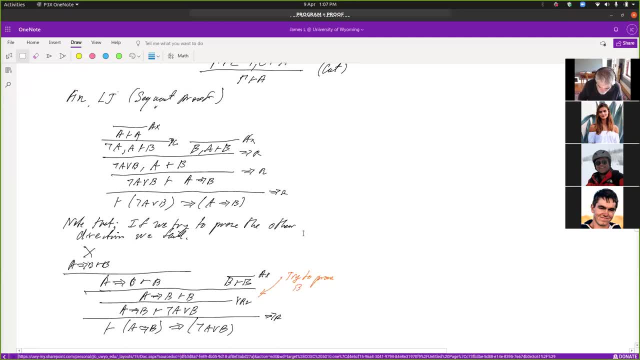 gross. We could say, okay, let's see A, B, true, true, true, false, false, true, false, false. And we could make out the proof table: knot A or B. And we want it to be if and only. 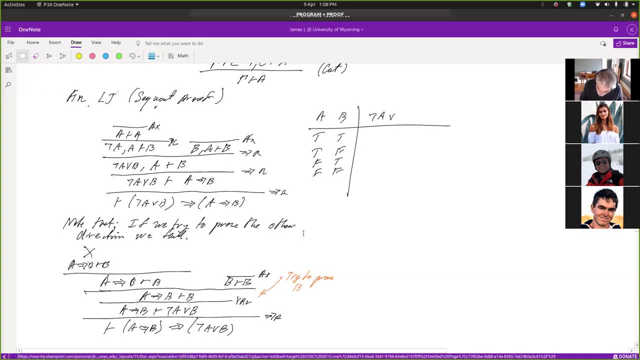 if A implies B, And so knot A, it means false and true. So that's true And this one becomes false, And this one becomes true And this one becomes true Because that's true. Knot A knot false is true, So then that's true And then that's the same as this truth table. 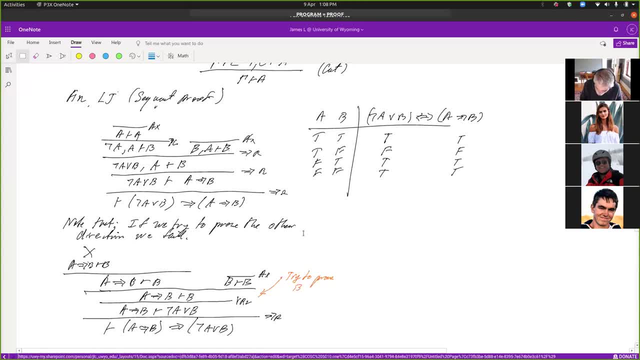 Okay, And so it's true that they're both true. They're both false. This is the main one I'm looking at. They're both true. So here's a truth table showing you that, um, this is an if and only if in um classical logic. 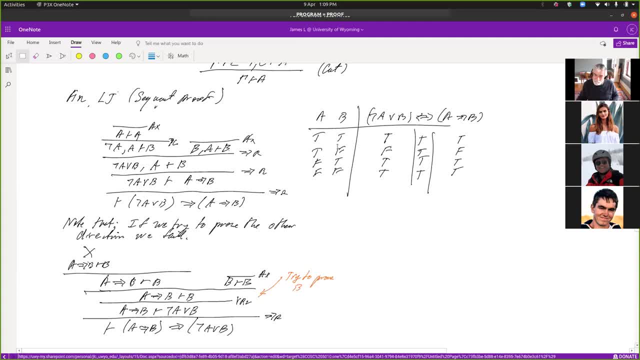 Okay, because these are models. The booleans form a model for classical logic, and here's a semantic argument that this is true if, and only if, this is true. But you can't prove it the other way. So here's the sequent proof. first of all, If you go back, if we went back to Mimram and look at his 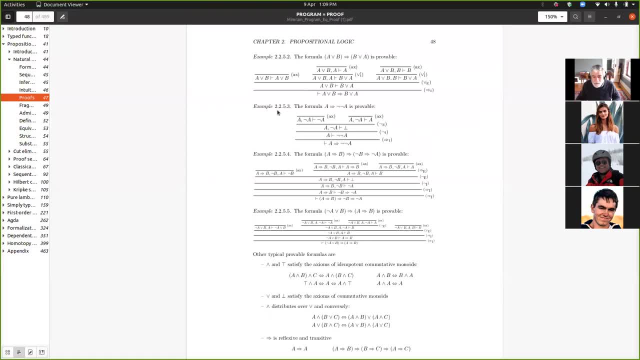 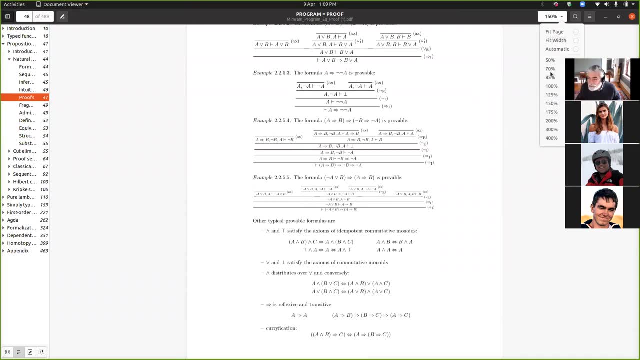 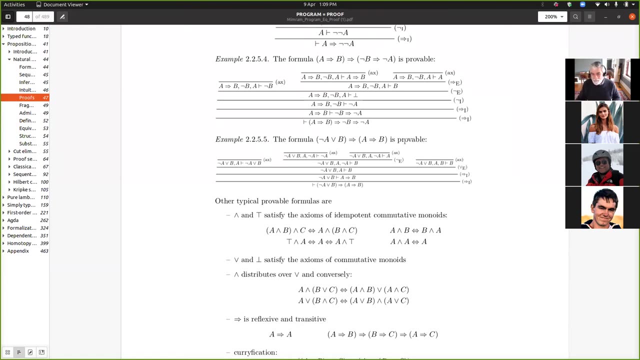 proof of this. first, maybe let's look at his proof of this. It gets kind of small, So I think I could blow this up maybe. Okay, He says this one's provable, but it's so interesting to me that he doesn't note that. 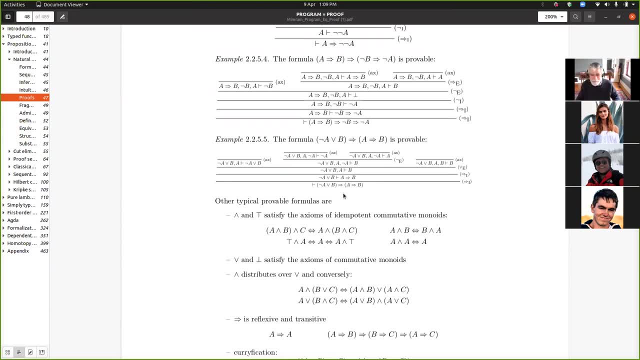 the other direction is not provable. I think it's kind of odd that he doesn't say here: but notice that the other direction is not provable And this one is also contrapositive. It goes this way but not the other way. 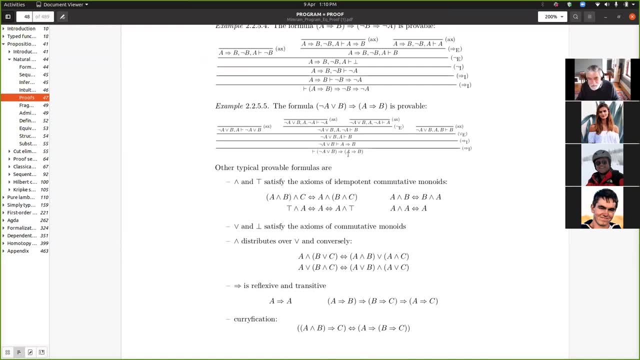 So his proof here is: okay, you know, implies introduction. that means you get assumed not A or B, and then he's got A implies B, so he does implies introduction again, and now he's got A or B and A. 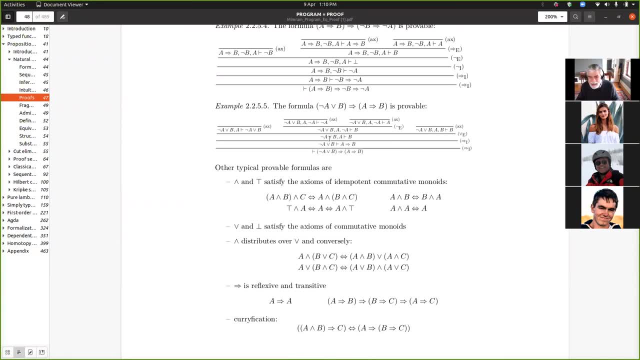 And he has to show B. And so now he assumes not A or B, He pulls that out of the assumptions and that's an axiom. And then over here, both of these branches, he's going to show B, So he's. 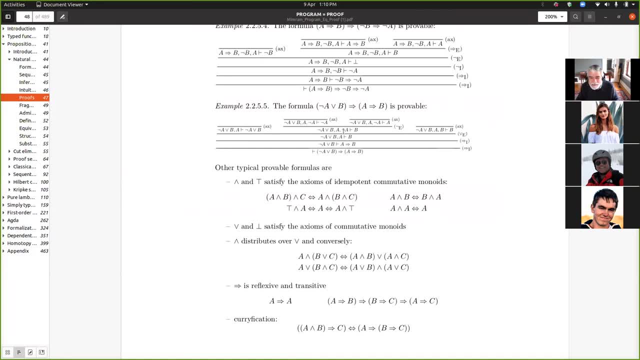 got all this stuff And so what is he doing here? So then he has to do: oh, he's, he's using, he's going to prove it, He's going to prove, not A and A, and then that lets you assume anything, Although that's funny. 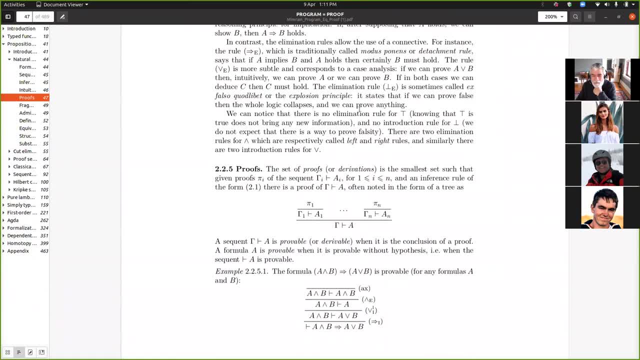 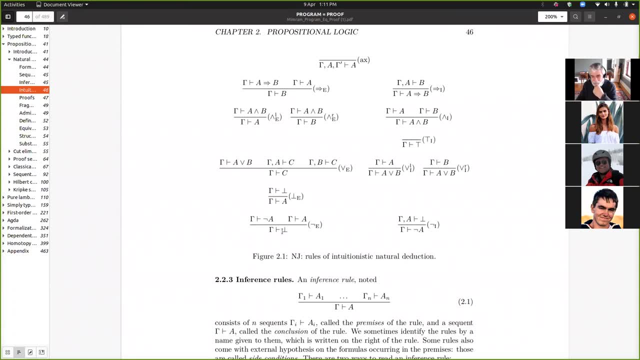 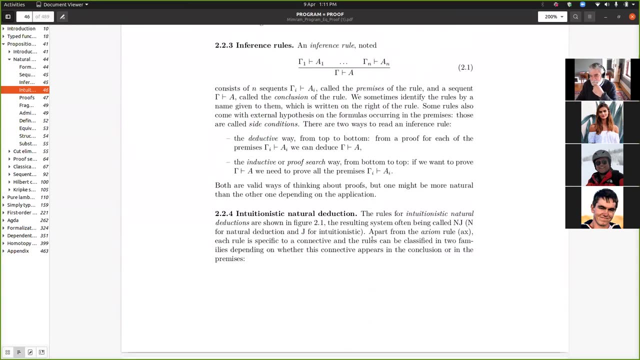 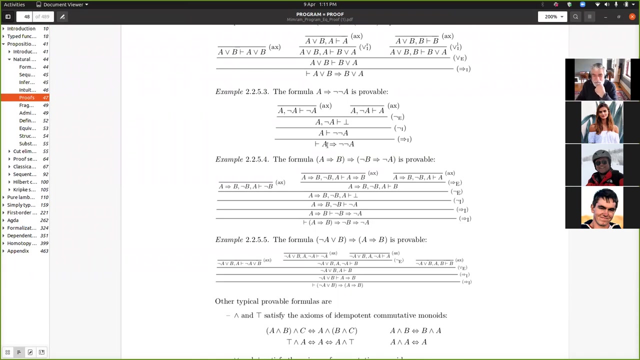 because in his rules, I think he has to prove bottom first, doesn't he? He has to prove bottom and then this rule, So he's missing a step in the proof there. Okay, Because he just goes. I mean, you can rewrite this rule to work this way, but he really needed to go. 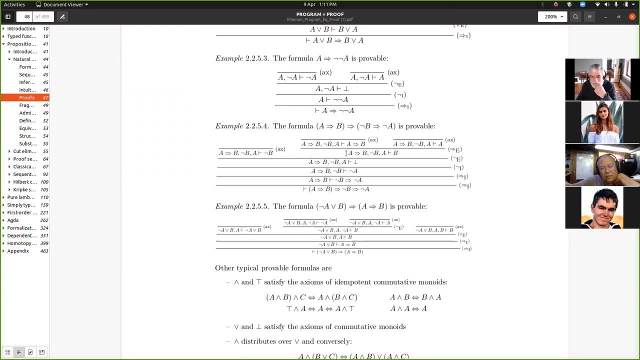 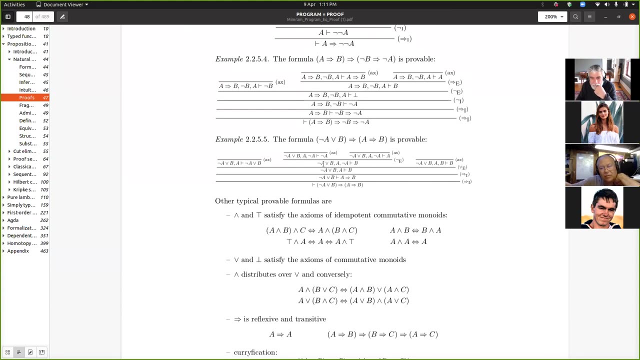 have these two things go to? oh, they do, I guess. Okay, All right, What was they thinking? Oh, it's in this proof. Okay, Here he's trying to use, not A. There should be one line inserted below this where you've got this thing bottom and then. 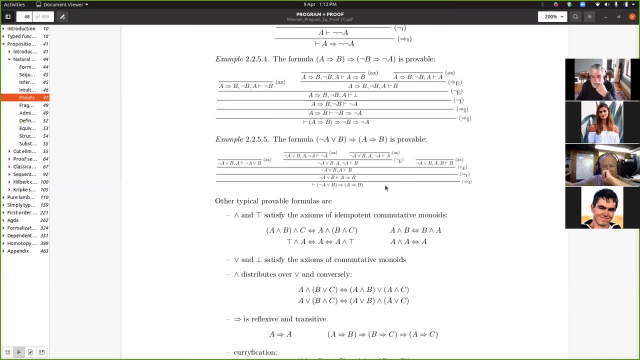 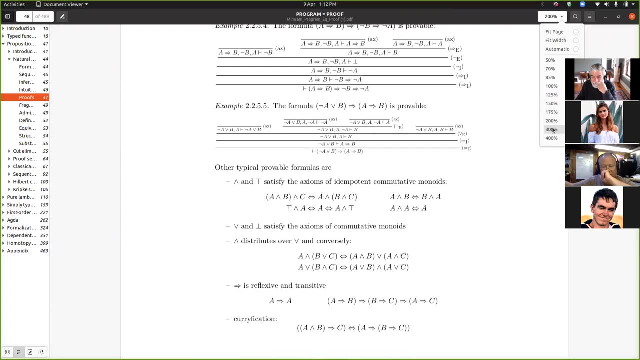 you get B. Somebody double-checked me, Am I wrong? You see what I'm saying. He had: oh, I need- I really do need- both pads. Let's see if I can get the other one working. Finley, you're pretty good at these proofs. What do you speak up? 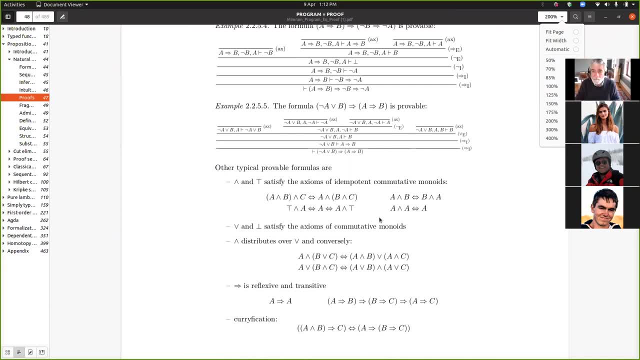 Do you see what I'm? do you see what I'm saying here? Will you repeat it? Just that he's missing a rule, because he's invented a new rule that says if he proves not A and he proves A, he directly goes to B. But his rule says not if I prove not A. 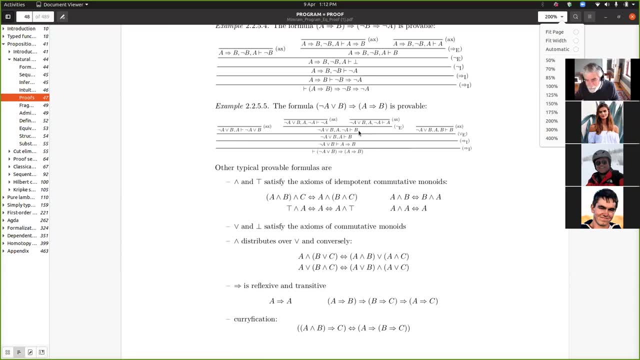 I prove A, I go to bottom, and then from bottom I can go to B. Oh yeah, He's missing it there. Yeah, Yeah, But still you have to like it's, you have to be like a little bit inventive here, right? 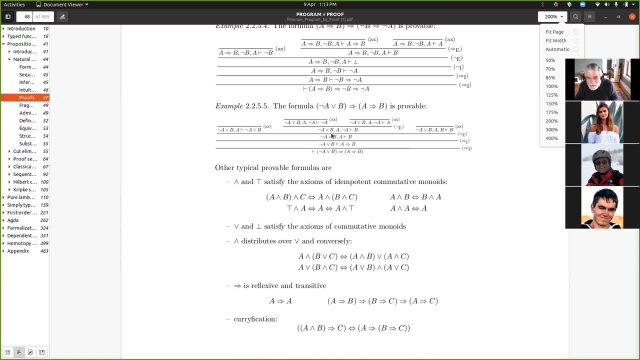 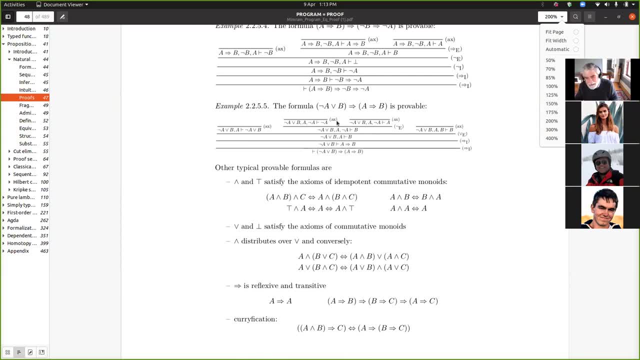 Right, Right, Right, Right, Right, Right, And then I prove A, and then I prove not A, and that gives me bottom, and bottom gives me B. So this is another letter to MemRAM. And then what's on this one And that one's? 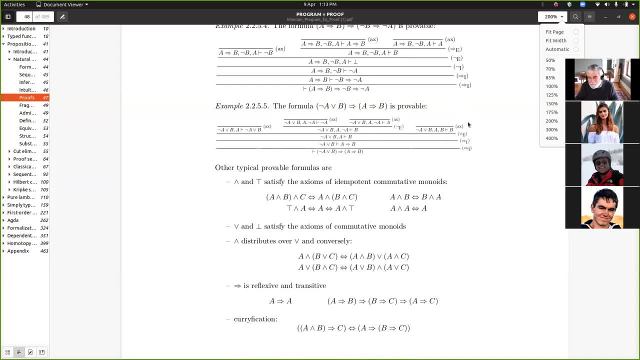 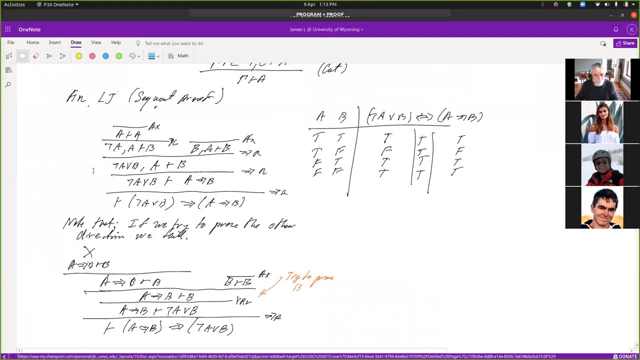 easy because you get to assume B and you got to prove B. So anyway, I think that this proof is much harder to do Then this proof here, because in this proof you only work backwards, You never have to kind of like do the forward style of thinking. 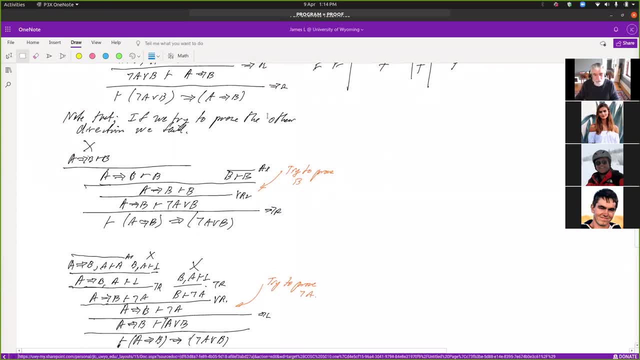 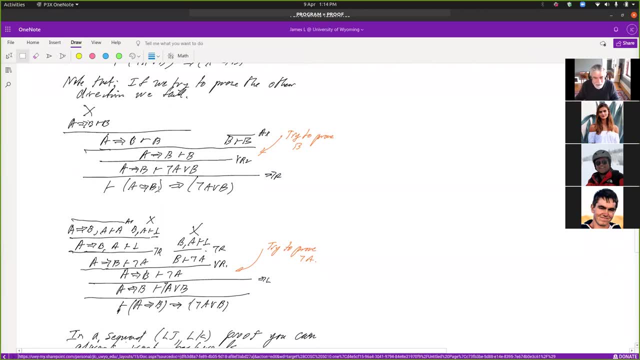 Now, if you try to prove the other direction, here's what happens. Like, okay, you apply implies on the right, because there's the principal connective. So that means pull this over here and put that there, And then you could say, all right, well, I'm going to either have to prove, to prove, or 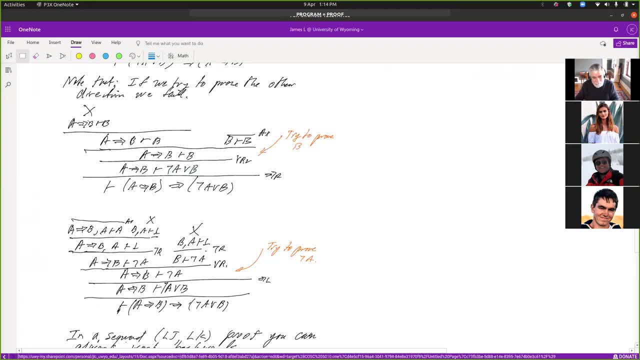 I either have to prove not A or I have to prove B. So let's try to prove B. So we have A implies B and we're trying to prove B, And so then you say the only connective left is implies. 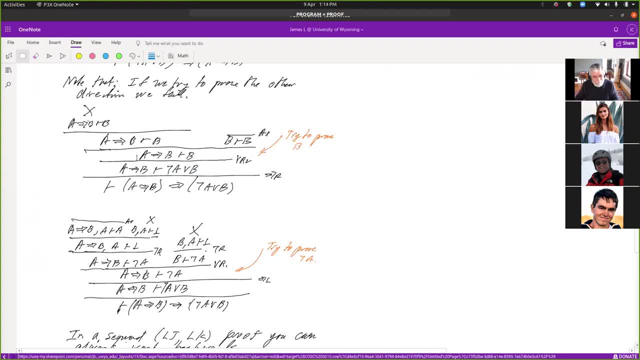 And from that says: okay, I could use this, helps right over here. right, If I could get B, Oh, but this should say A over there. That's a typo, There's mine, Okay, Okay, Okay. So this one should be A Cause. that's. what I have to prove is the antecedent. 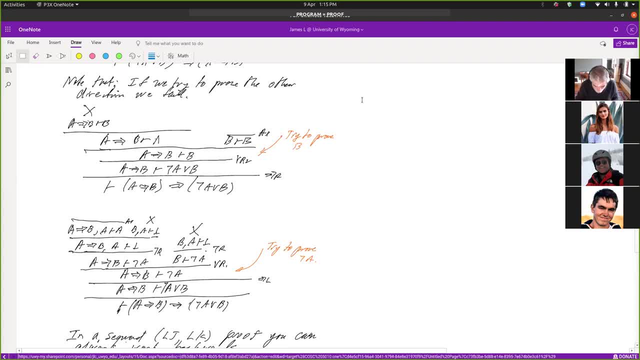 But now I get stuck kind of in an infinite loop. I go like, oh okay, I got to prove A implies B implies A. Oh okay, Okay, and I mean the only connective is implication. so the only thing I could do is do the implies. 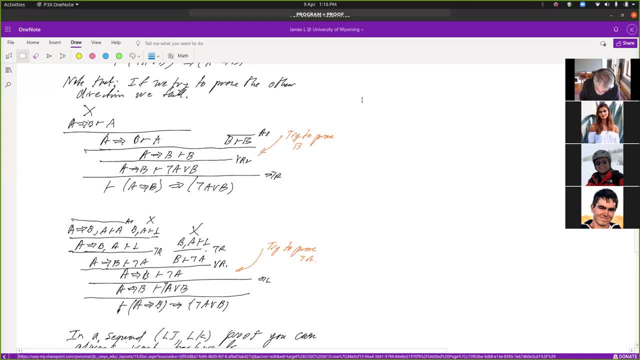 on the left rule. So this one here was implies on the left and this one is implies on the left. and now I gotta prove from: A implies B, I gotta prove A. so oh, I get to assume B over here. I gotta prove B turns to A. I can't prove that. that's unproved. 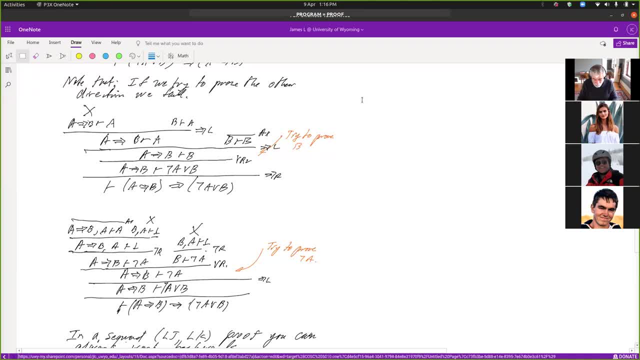 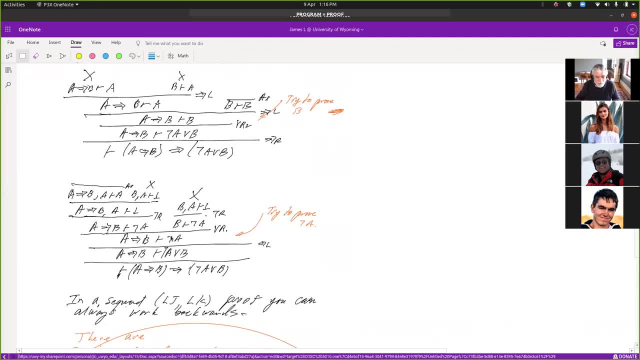 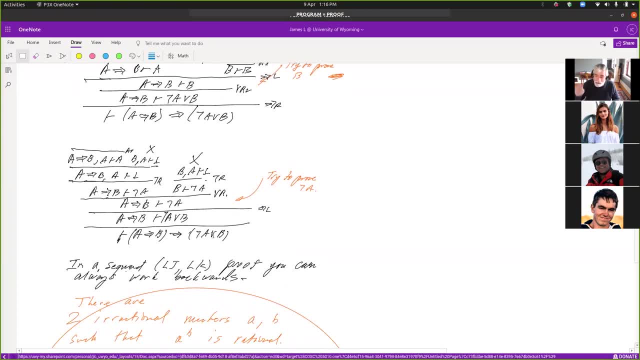 Now we haven't really tried every possible permutation of proofs like we we had. the only rule that applied here at this first step is: implies on the right, And then we do the. oh, this is, I'm sorry, this is the. or write one rule. 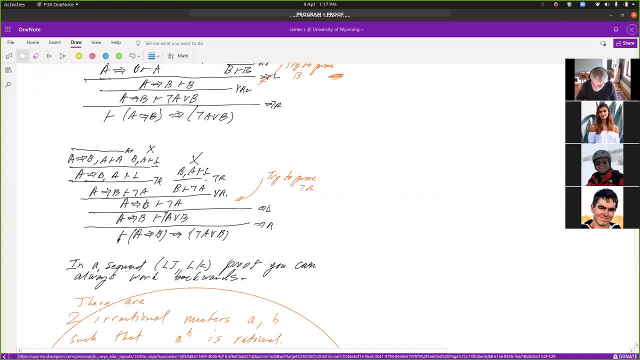 I mislabeled this thing. So from here I got or write one and I'm going to prove not A. And then what did I do here? Here I did the implies On the right, But again you can't get to. 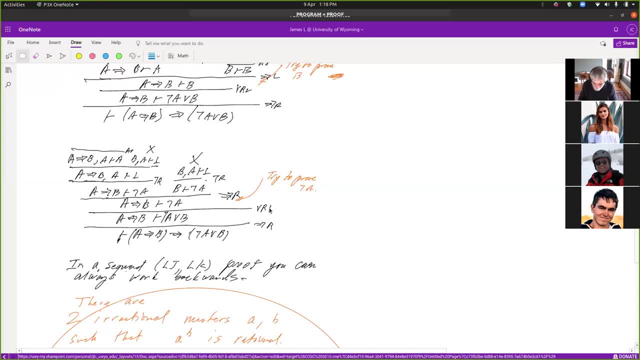 you can't get to a proof Like this one, for example. here you can never prove false. So this is completely blocked. This one's blocked because you end up getting stuck in a loop where you're trying to prove the same thing over and over. 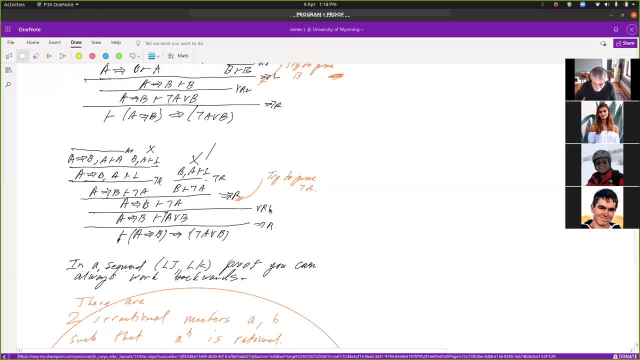 and over again. Now it turns out that this is pretty weird. It's in MemRAMP. There are no. so like for classical logic or classical propositional logic, a two-valued set can can serve as a model. 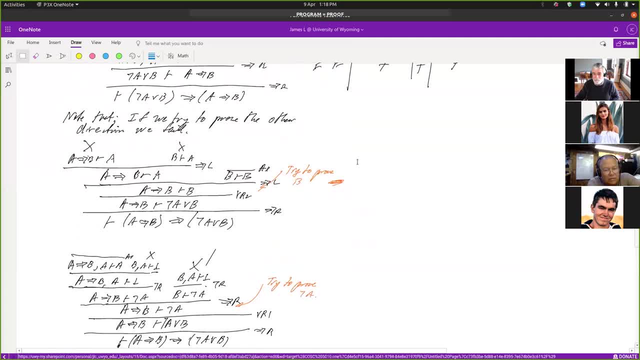 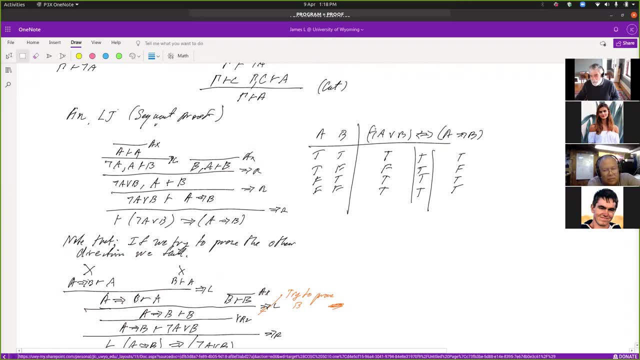 And that's what we do when we draw truth tables. We define the meaning of you know true or well, this we define the meaning. I didn't write down the separate columns, right. I just wrote, not A or B. 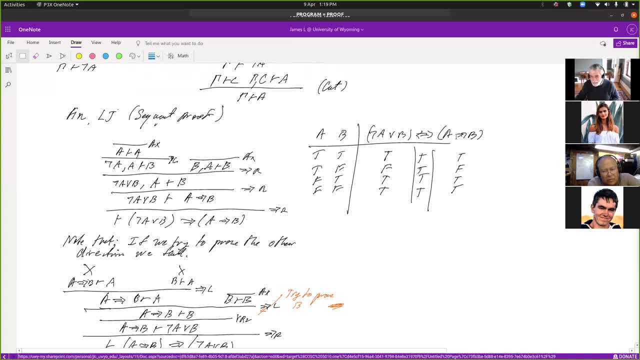 So we define the meaning of, or we define the meaning of implies, We define all these meanings using a two-value set, and it captures perfectly the meaning of these formulas. And so we can find the semantics using a two-valued set For intuitionistic logic. 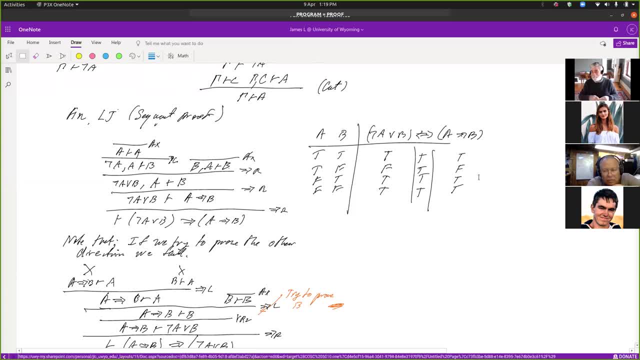 it's can. it can be shown that no, there is no finite K for which a K-valued model will work, So there's no finite valued models. And then, amazingly, Saul Kripke was a is a philosopher at Princeton still, I think. 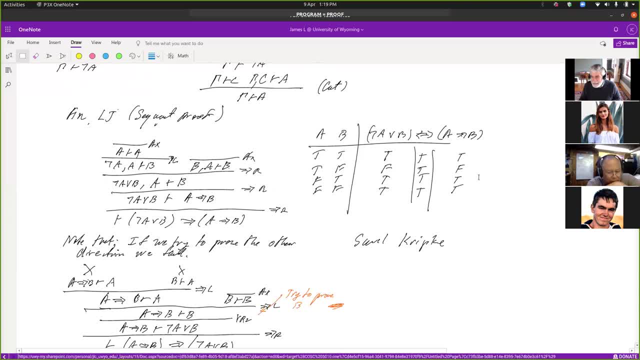 And he was a kid, like he was like 16, and he figured out semantics for intuitionistic logic And it turns out they're Kripke's doctors. they're called- I don't think he called them that at Princeton. I don't think he called them that at Princeton. 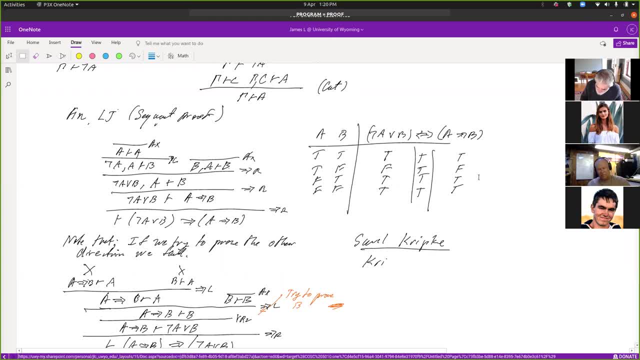 I think he called them that at Princeton. I don't think he called them that at Princeton. But and they're kind of, they're tree structures where at each node you label the things that are true. at that node you label the things that are true at that node. 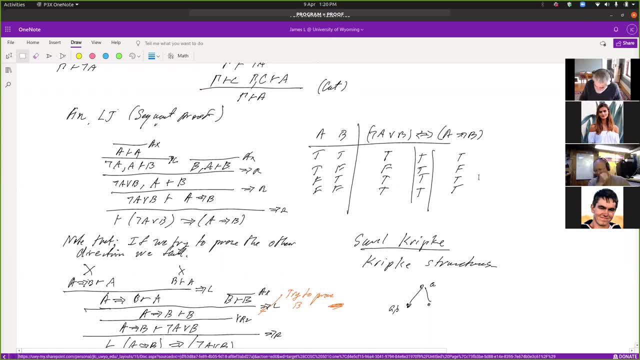 And the atomic formula that are true, and then a Kripke structure can model a formula in the same way that, like a row, an assignment, which is: you know, oh, a is true and b is true. so you know in in here that that's one assignment and another. 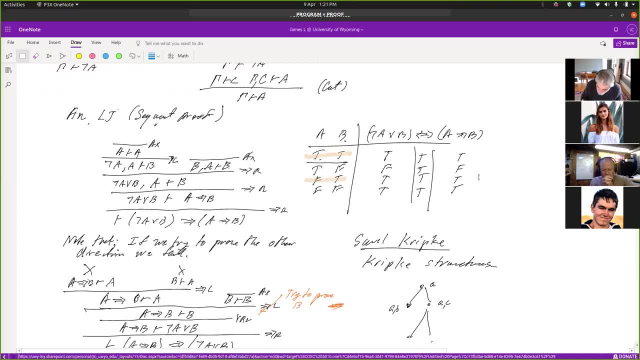 assignment is. you know, a is false, b is true. so each of these crypti structures corresponds to essentially a row of like an assignment, and then you can say there's a way of defining whether or not a formula is true in a particular crypti structure and then, if it's true, 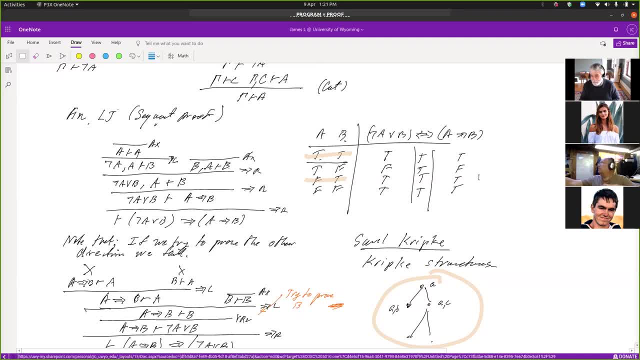 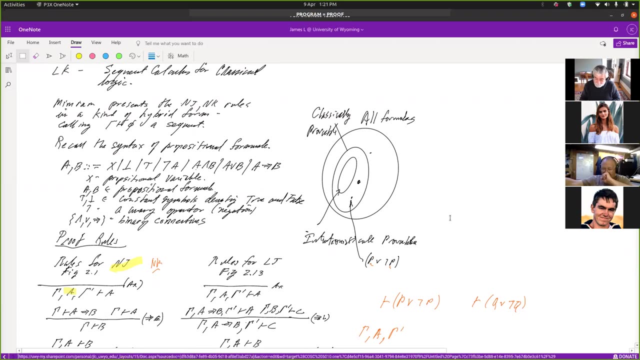 in all of them, then it's provable or valid. so now let's go back up here, because i think this picture leaves you with completely the wrong idea, because it turns out that um for for propositional logic, you know. so this is by a russian mathematician. 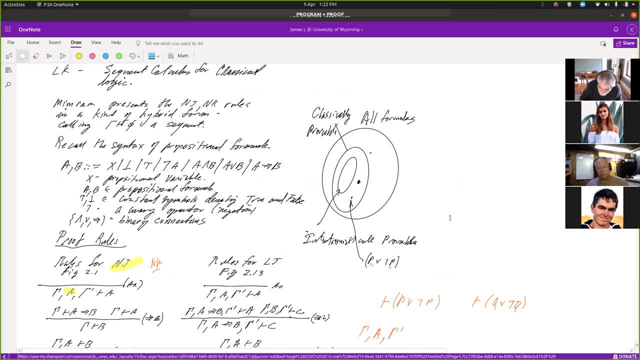 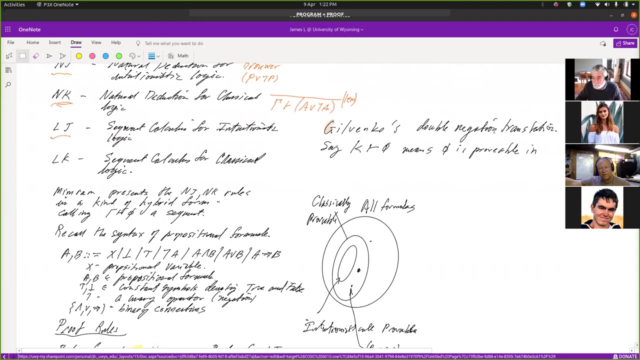 givenko, uh, double negation, translation, translation and basically, if, um, you know, say k turnstile, phi means phi is provable, a provable formula in: uh, i don't know, we pick your favorite. uh, oh, you need to scroll up a little bit. you're up above us, okay. yeah, there you go, i know and i don't. 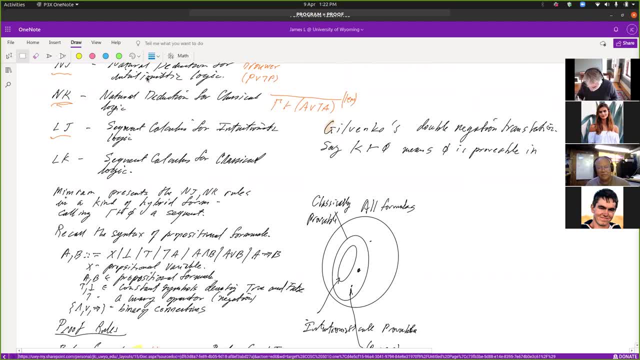 know, these little side things come in on this and i never know how to get rid of them except by leaving the app and then coming back. okay, so anyway, you could say in class one is probably the most appropriate theme in twentieth century. so anyway, you could say in class one is probably the most appropriate theme in twentieth century. 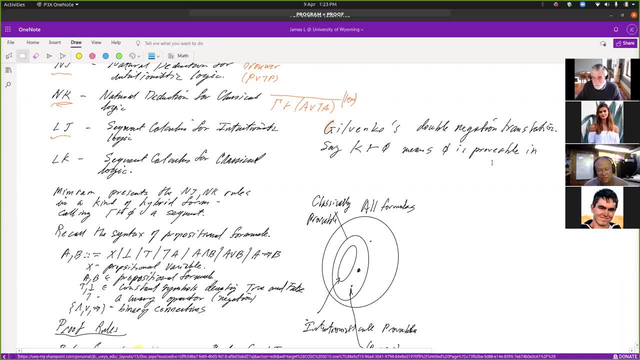 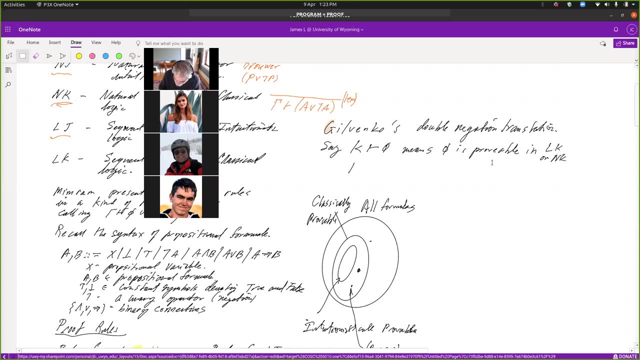 logical logic the formula phi is provable. So we could say like in L, LK or NK, and then we can write int turnstile phi means phi is provable in LJ or NJ, So intuitionistically provable. So this is classically provable. 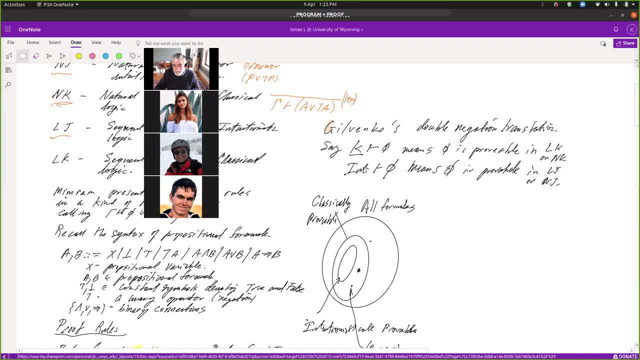 K is classically provable, Int is intuitionistically provable And Gilvenko's theorem says that if K proves phi- and it's actually an if and only if, K proves phi, if and only if int proves not, not phi. 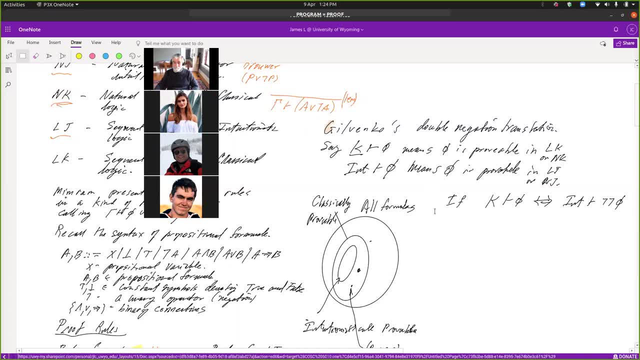 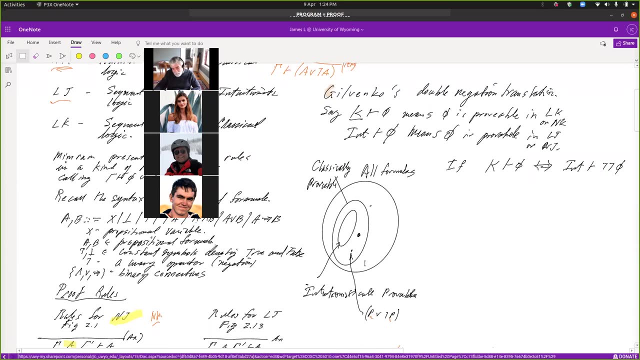 Come on, there you go. So this is crazy. So that means that- and Memram showed you one of those- like, for example, in this thing here I'm saying, okay, P or not, P is one of these formulas that you can't prove that formula intuitionistically. 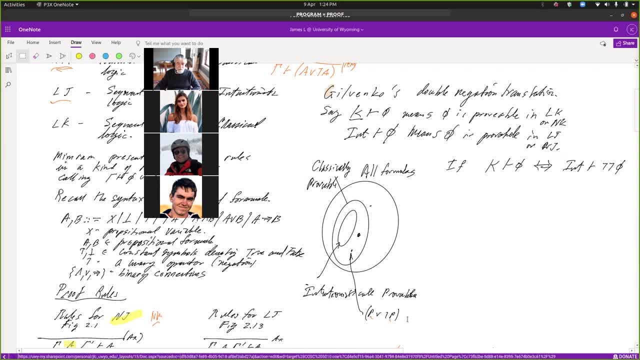 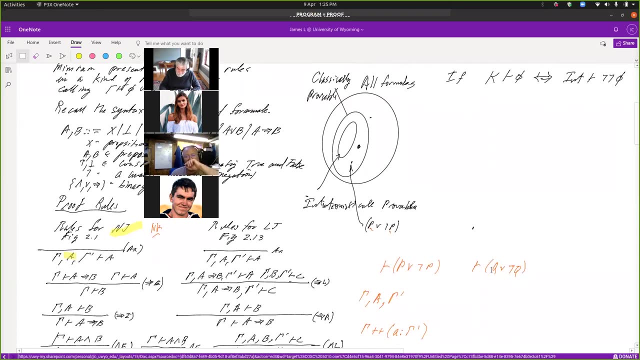 you can't do it And you can use Kripke models to show that it's never true. But you can prove. let's see, let me scroll up so I have some room. You can prove not, not P or not P. 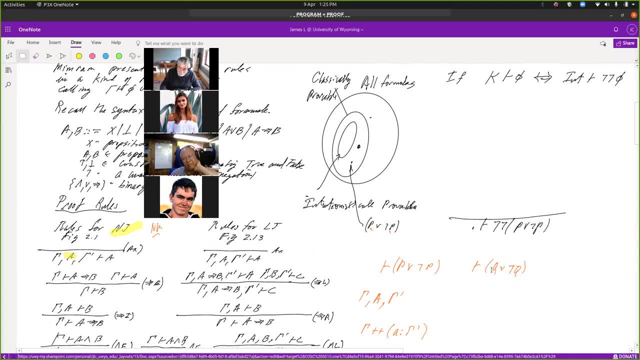 And the rule for not on the right whoops says you gotta prove not P or not P, turnstile bottom. And then we have a not on the left whoops, not on the left row. the left says keep this over here, P or not P. 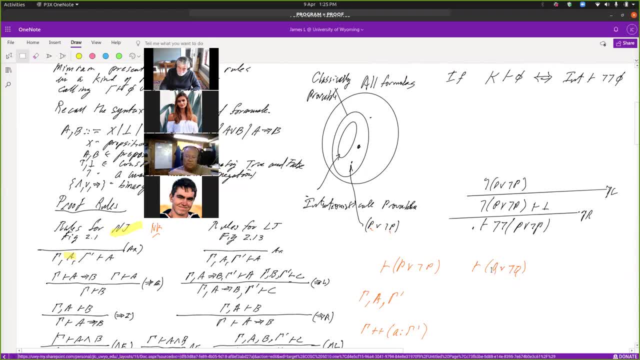 And says you gotta show P or not P. And so which one do I wanna try to prove? Probably not P, yeah. So I think I'll say, okay, prove not P, because the or on the right role says you gotta pick one of these. 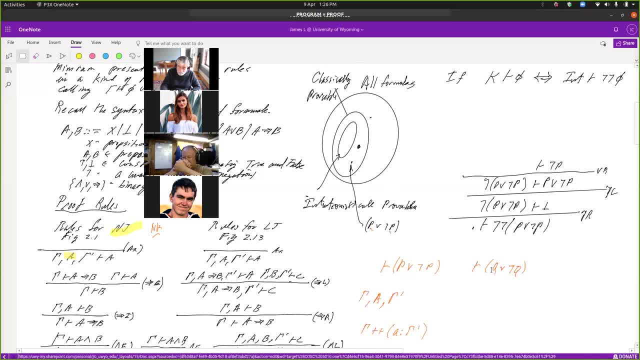 So I'll pick the second one, And I still have not P or not P. And now I could do not on the right, and I get not P or not P and P. Ah, come on, what are you doing? My thing went. oh, I must be in some kind of trouble. 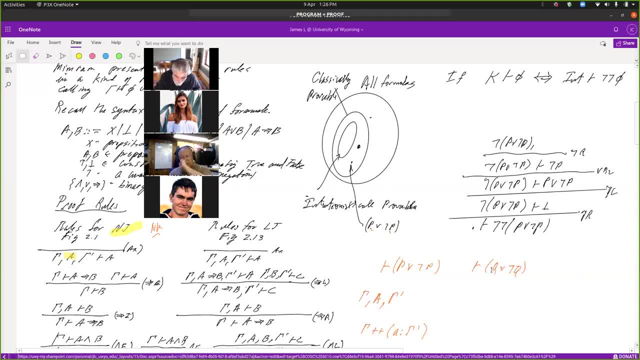 I'm in some kind of mode- I don't wanna be like that- Turn that off. I was trying to draw boxes and figures And so P comes over and now I have to show bottom. but now I can do the not on the left rule. 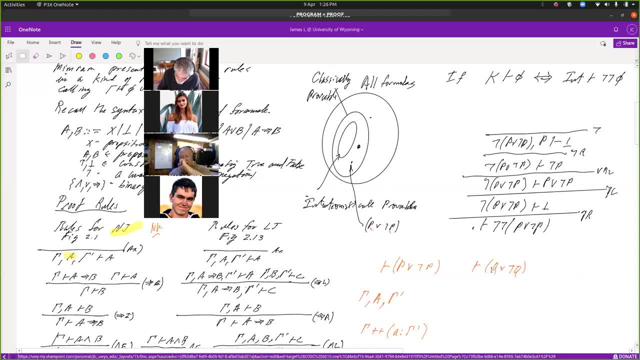 and I know P and I have to show P or not P, And so I could do. or on the right again and say, okay, P, turnstile P, And that's an accurate, That's an accurate, That's an accurate. Now, to me this is a pretty first of all. 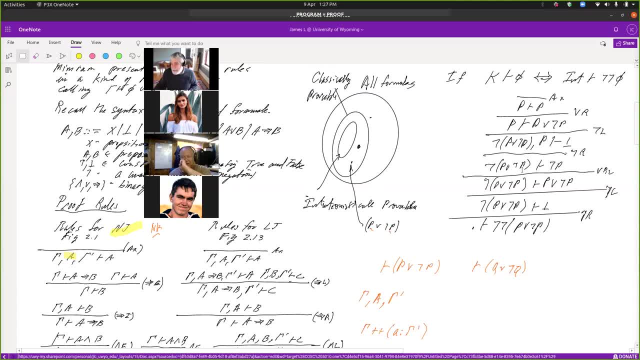 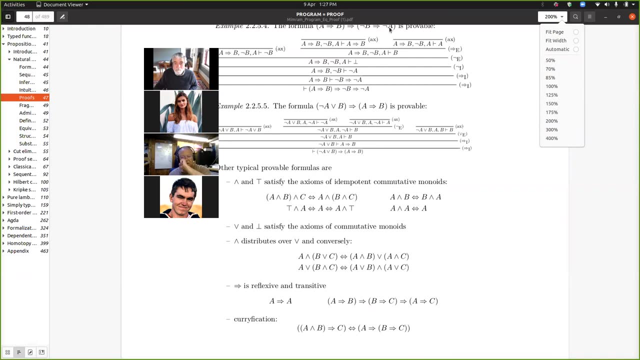 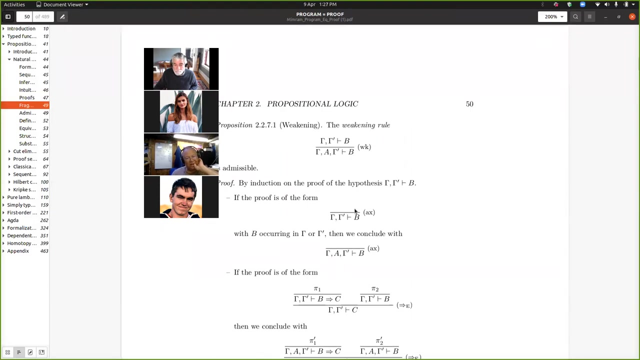 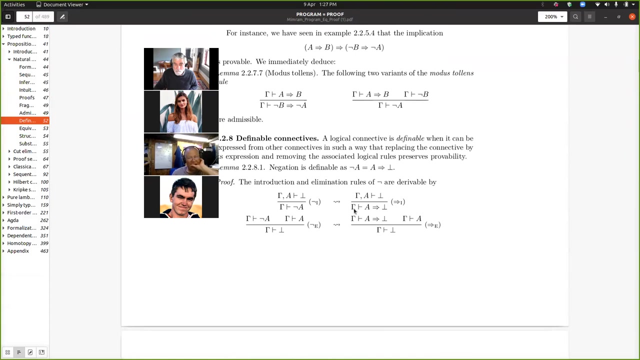 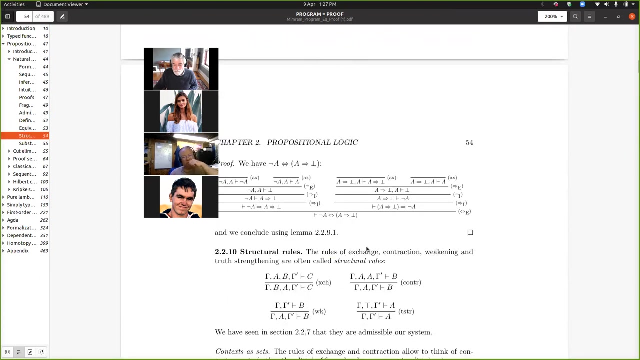 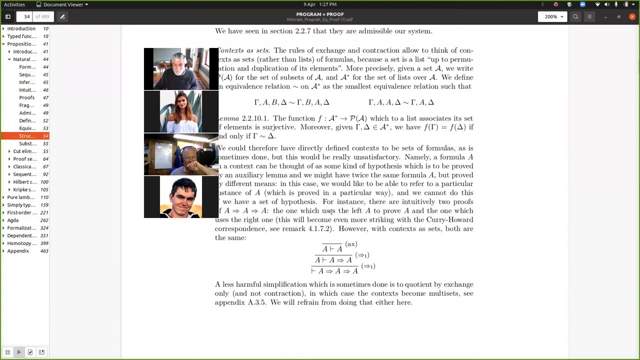 I mean I can just write this proof down by following the rule. There's no thinking. If you look, he has a proof of this somewhere in here. I thought I don't see it up. Anyway, he does. somewhere in here is a proof of not not peer. 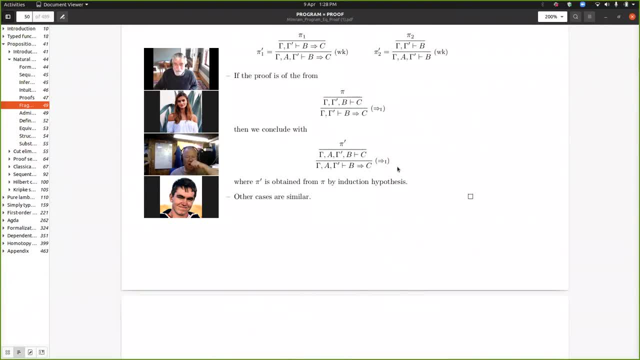 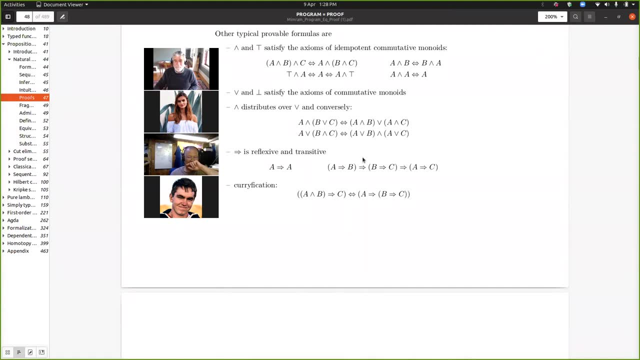 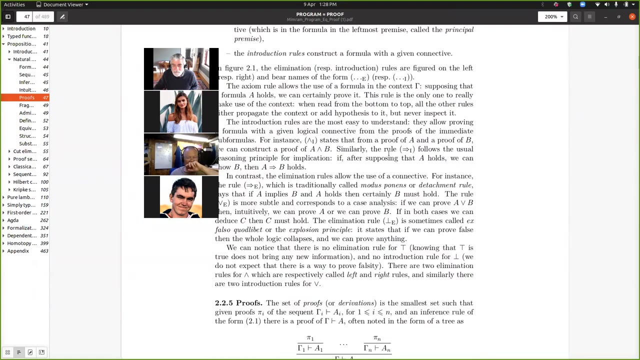 not not. It's not a proof. p or not. p not not excluded middle or LEM. law of excluded middle stands for LEM. Does anyone remember? did he prove it here, or maybe not? I thought I saw a proof of it here. 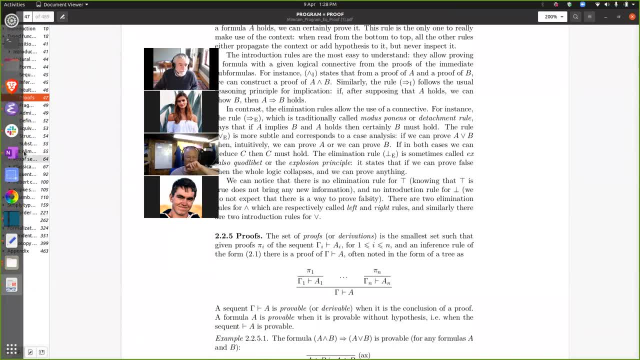 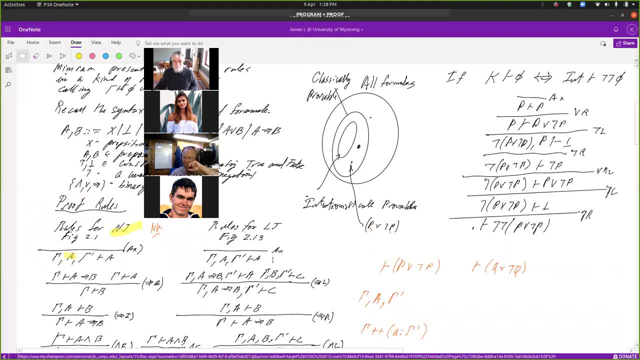 somewhere. Okay, well, so if not, what we just did was a new proof for you, except I did it in this LJ calculus. So the thing is: is that this is a little bit subtle, but it's, and it's, a little bit? 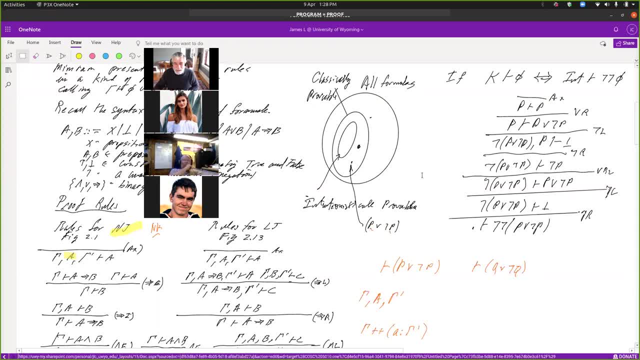 weird is that if you are a classical logician, if you believe that, if, if, like your own epistemology, how, how you know something is based on classical logic, then to you, then to you the formula not not p- is true, if, and only if, p is true, You take it as exactly the. 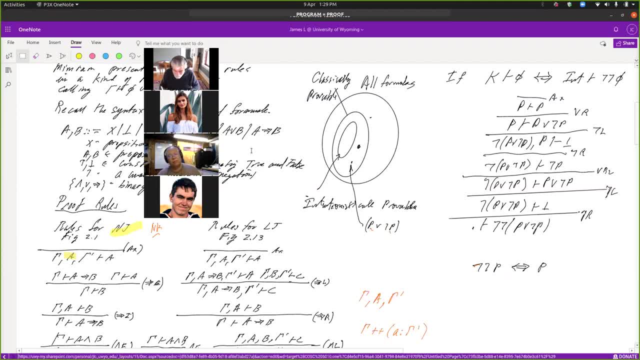 same thing. It means the same thing to you. So since I proved not not p, you could take this and then do the same thing. So, since I proved not not p, you could take this and then do the same thing. So, since I proved not not p, you could take this and then do the. 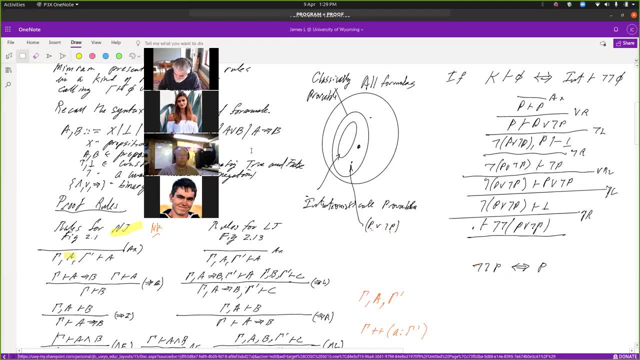 mind. and then you could do some kind of classical a derived rule- not not mind. and then you could take this and then do the some kind of classical a derived rule- not not elimination, and you would get p or not p. but this last thing, but this last thing I should have made. 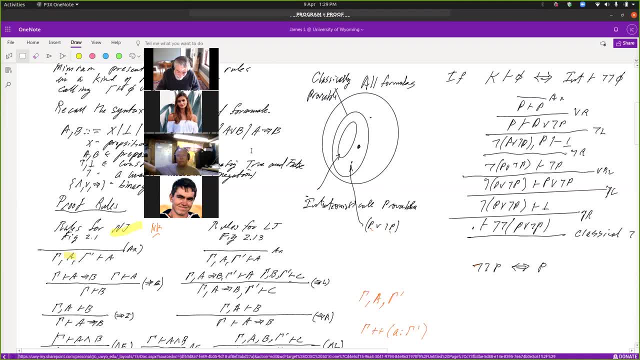 elimination and you would get p or not p. but this last thing- I should have made it read um- is not acceptable to an intuitionist who doesn't believe that our に, knot, knot is the same, because you can't approval as to what that might be, or if rock doesn't belongs. 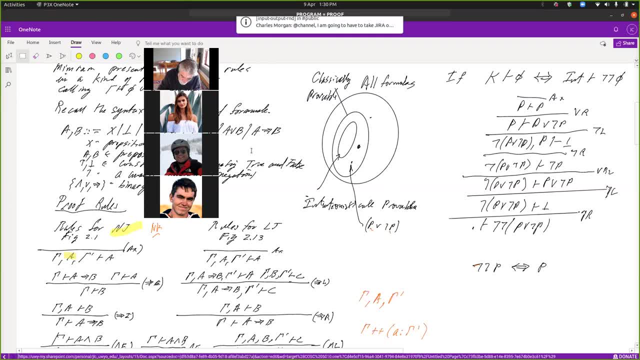 knit, knot. knot is the same because you can't shape it if it wasn't in the clothing socket, or this is left out, or like are there serve by exciting example where it's just a vague mungkin cause they way that give us. So this is, this is classical, not not elimination. 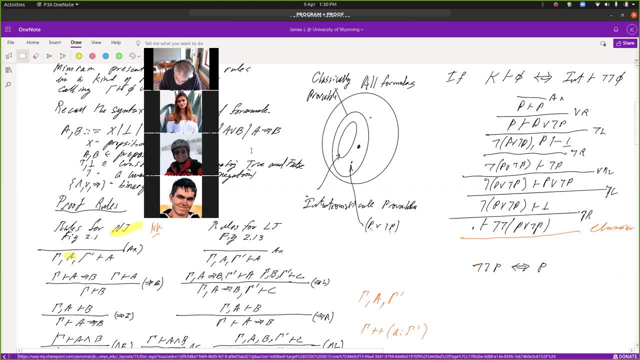 And that's perfectly valid as a derived rule. And so you get P or not P, But the intuitionist says no, that's not a valid step. So what's going on with this? not not thing. Why is that not a valid step? 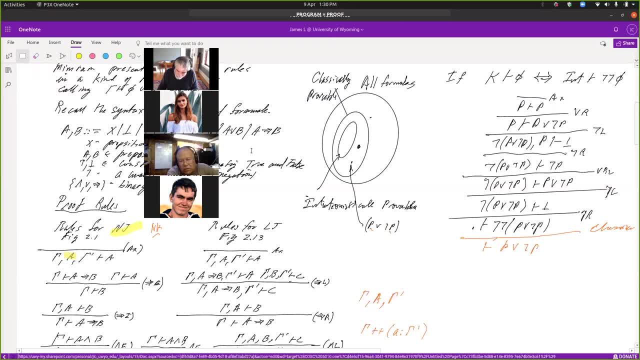 Because, in the end of this, if you apply this step, you don't know which one of P or not P is true, So, So, which of the two of? uh-oh, I got to move over a little bit, Hmm. 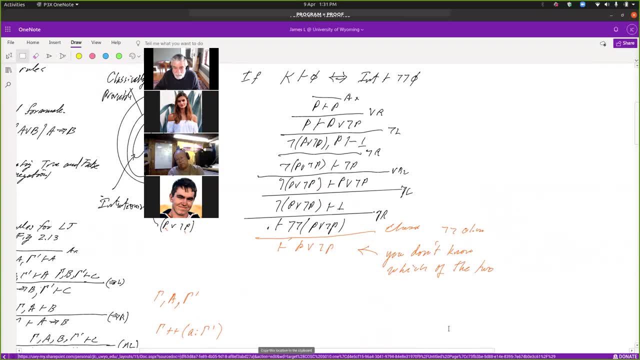 Well, it's not letting me. Oh, there I go. So at this point you don't know which of the two, of P or not. P is true, But it doesn't bother. a classical logician. They say: we don't, who cares? 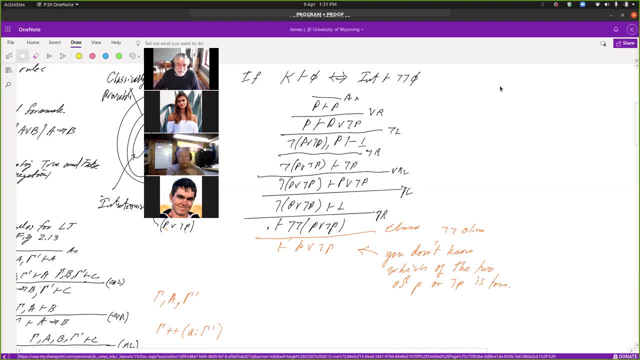 But this kind of means that this Venn diagram is not really quite correct. If you accept classical logic, then these two things are exactly the same circle, because you can always do a not not in front of it, And it's the same formula. 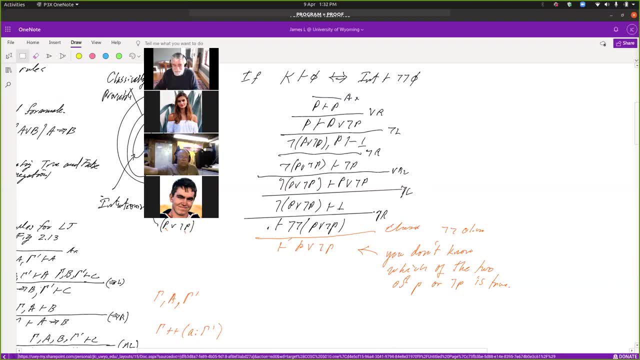 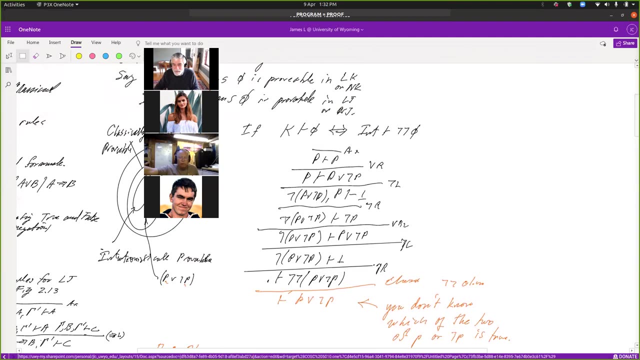 As the one without the not not to the classical logician, And so these two circles completely coincide. If you take a not not and add it to all these that are in this place here, So any class. that's what Gilvenko's theorem says. 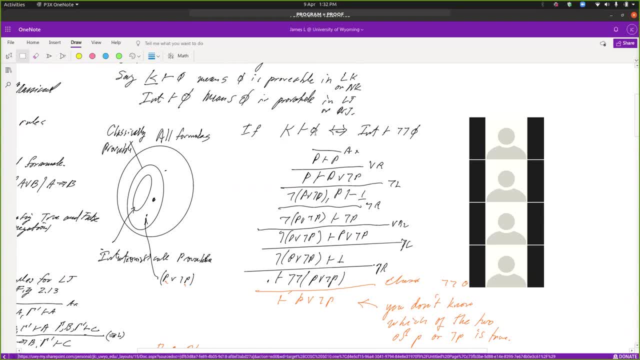 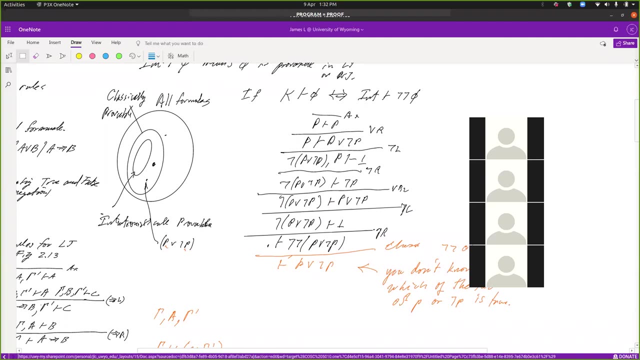 It says If K is or if phi is provable formula is provable classically if, and only if, the not not version, you know the disprovable intuitionist equate. And then it turns out that there's um. let's see. 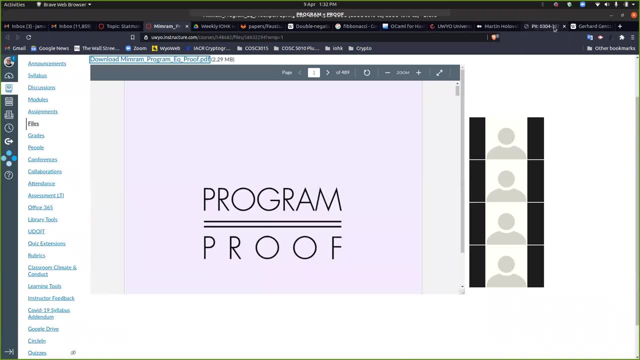 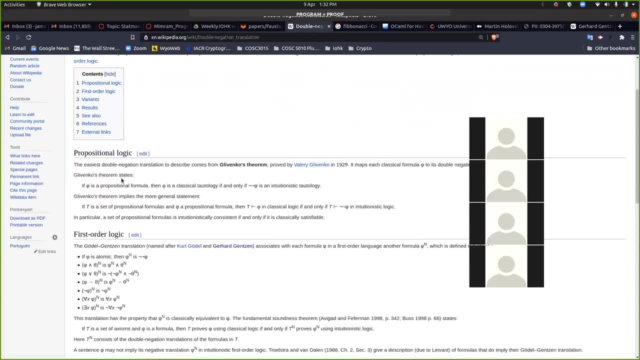 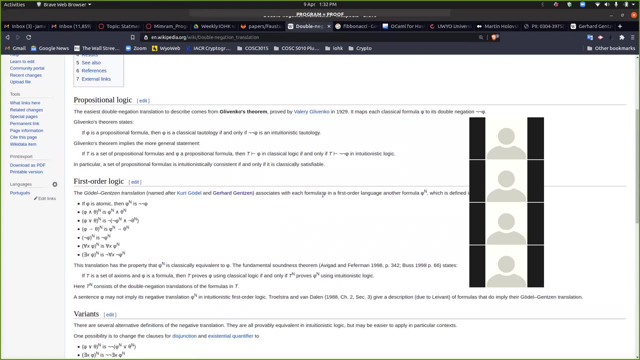 I think I might have an article about it. No, Oh, here it is. It turns out that, okay, this is Gilvenko's theorem, proved in 1929.. Oh, I should mention that. Uh, does anyone know? 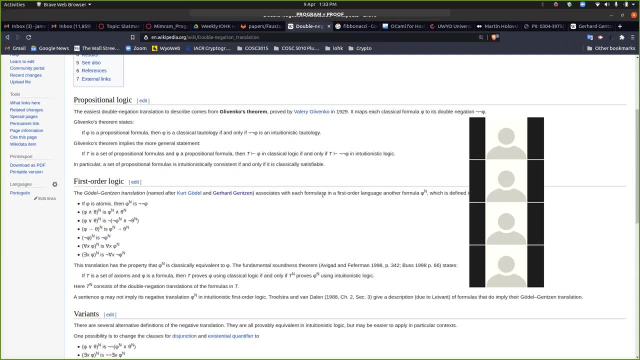 Do you know who Kolmogorov was? Has anyone ever heard of him? I have, Yeah, What do you? do you remember what he did? Um, what I learned about was Kolmogorov complexity, Ah right. 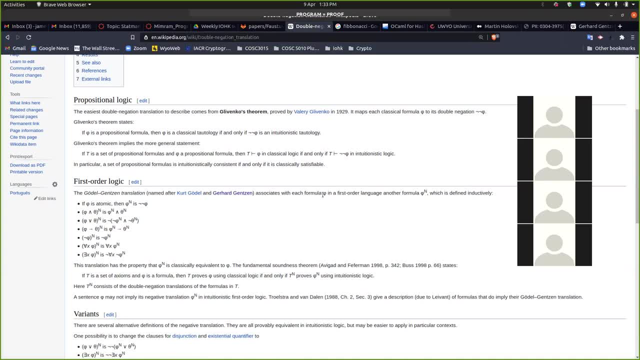 Right, They named a whole complexity theory after him because he worked. he worked with that as well, but he he invented. like the modern axioms that we use for probability were Kolmogorov's invention, And he was a a constructivist himself. 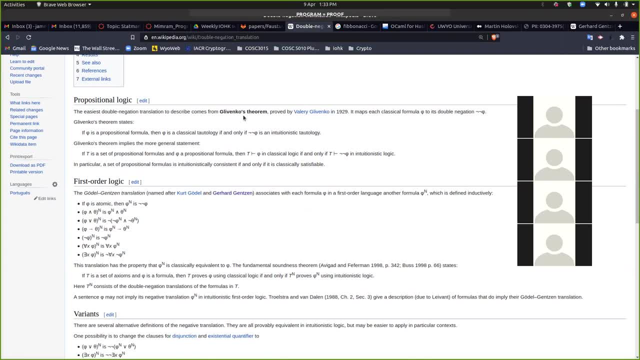 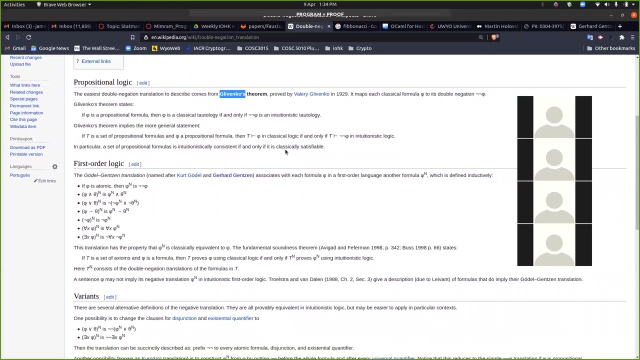 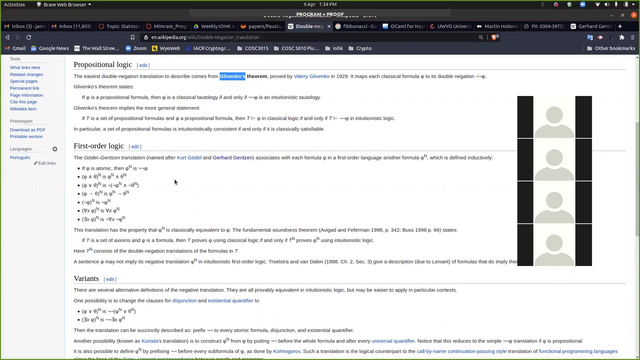 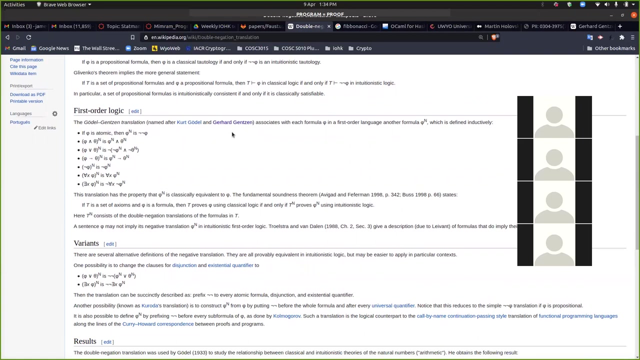 And then there were students in Russia. I wouldn't be surprised to find out that Gilvenko probably was a student of Kolmogorov Um, but they were working for him. I suppose You know what we, what we learned from him. 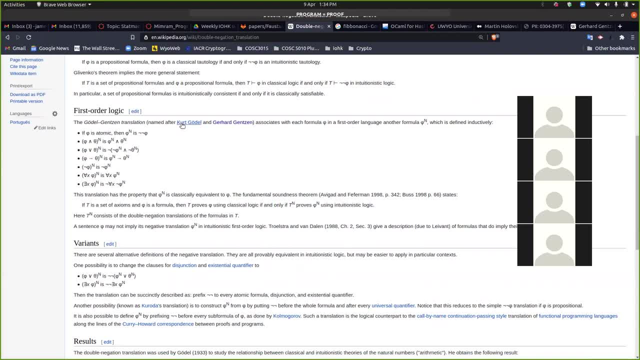 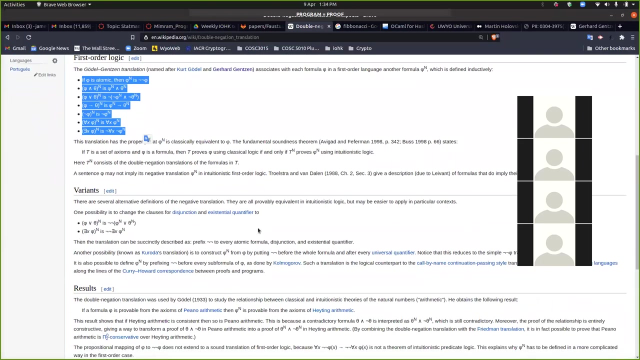 The two of them discovered this translation, which works for formulas with quantifiers, to translate formulas to essentially do exactly what Govenko's theorem does, except now it does it for first-order logic. And then there's other interesting ones, And then, God, there's. 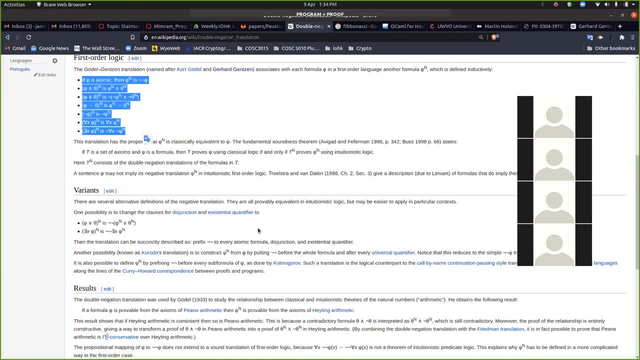 So a lot of it's been worked out, but there's something called oh, Friedman's A translation, And It's a different thing, And it turns out like, if you try to look at these, if you want to say like, okay, well, what is the meaning? 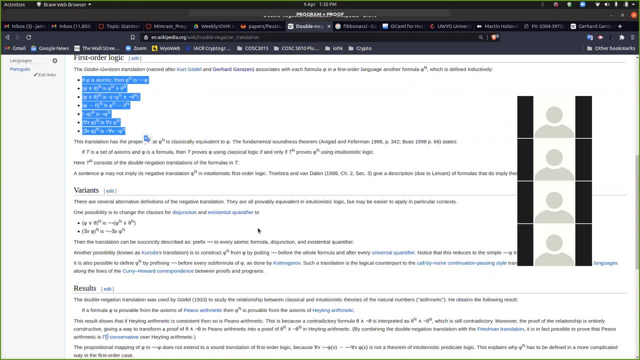 Like we We can do through the Curry-Howard interpretation. we know that, okay, constructive logic corresponds identically to type theory, to simple theory of types, And so we can use lambda terms as evidence that for that a type is inhabited. 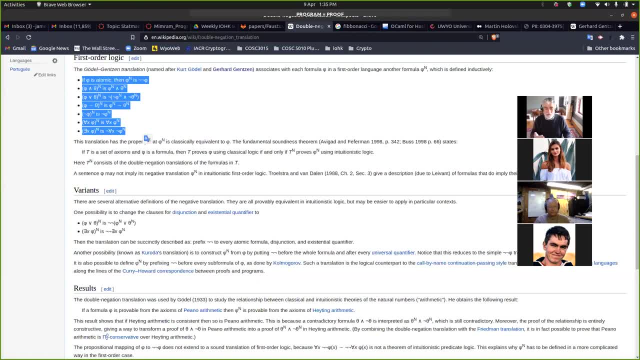 And so those lambda terms in some way are evidence also that a proof exists, because the trees are the same structure, The rules are identical, So can you use, like what happens if you try to do like a Curry-Howard thing to these translated things. 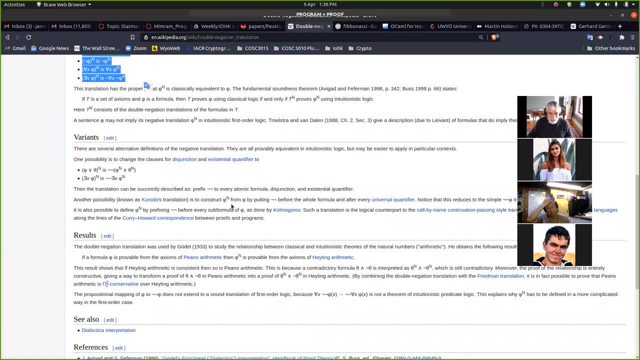 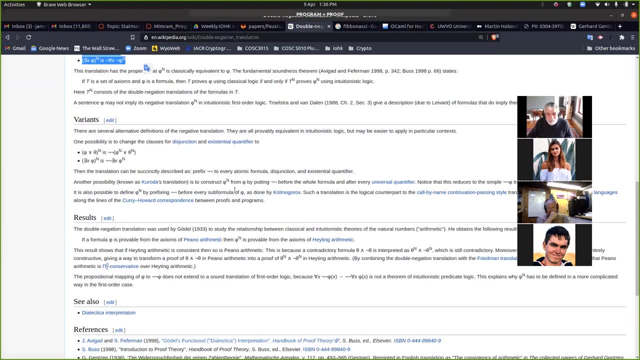 And I don't know. There's a lot of really interesting results. Um, Oh right, There's the Kuroda translation. There's the Komogorov translation. He was just just an astounding, astounding mathematician. 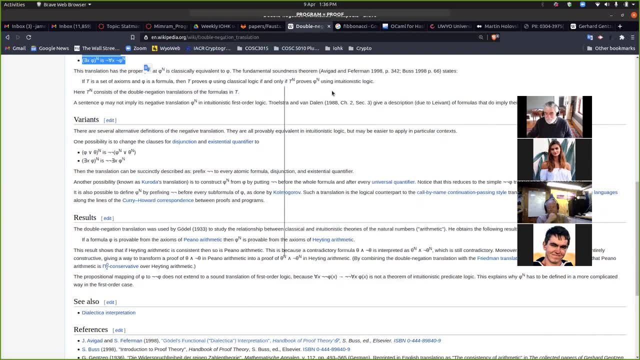 But we just don't know as much about him because he's Russian. Um He, I think he also made one of the early definitions of what tried to define randomness. Um Oh, and here's the Friedman translation. So anyway, Um, people have worked with these translations. 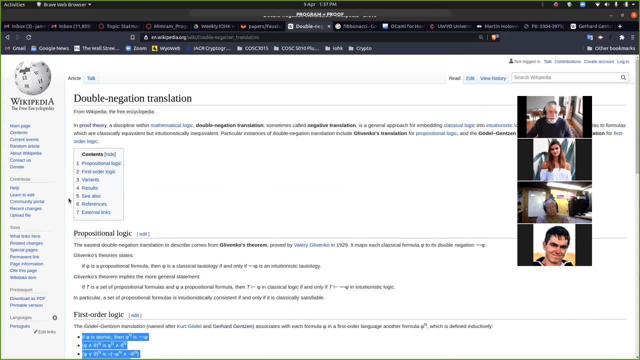 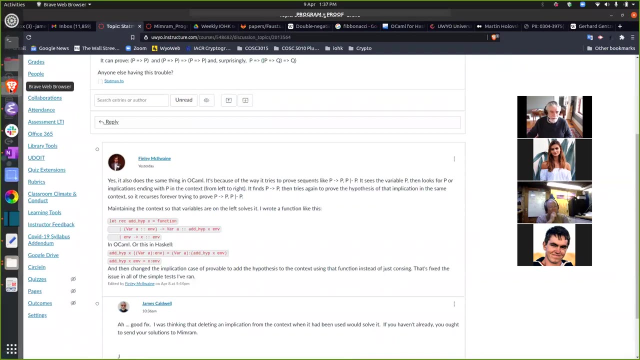 to try to figure out, like, okay, can we add computational content to classical logic? Can we figure out what? Can we extract programs from classical logic? All right, we have about a half hour, a little bit less. Um, first of all, any questions comments. 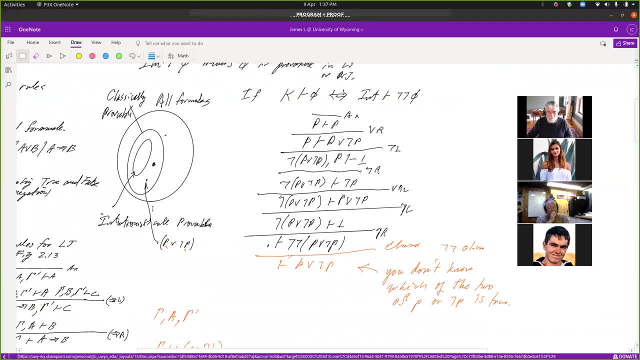 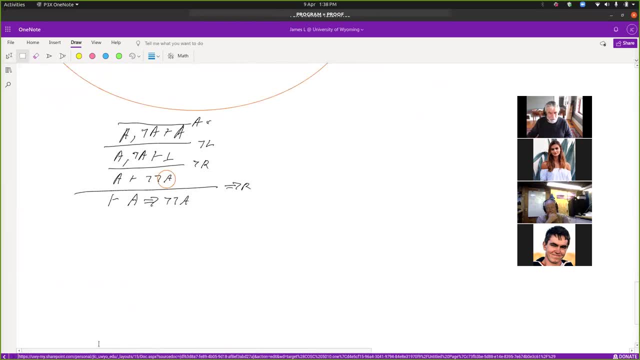 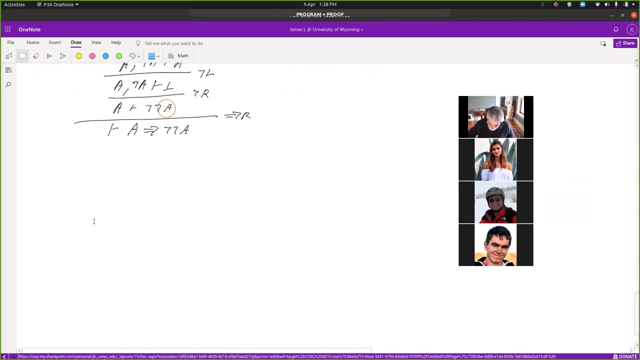 Is there anything you want to share to everybody? And then I'm ready to jump right into my discussion. No, No, All right, so what I want to do is I want to show you, um, um, the idea which you can track here. 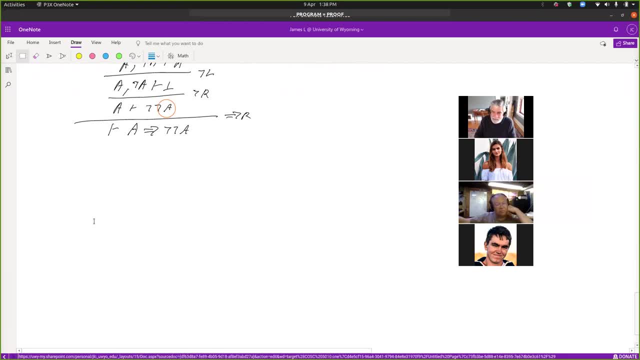 the idea which you can track um, which is quite similar. Kleene did this right, You remember, like the Kleene star operator which defines that he's maybe most well-known in computer science for Kleene star, you know, sigma star. 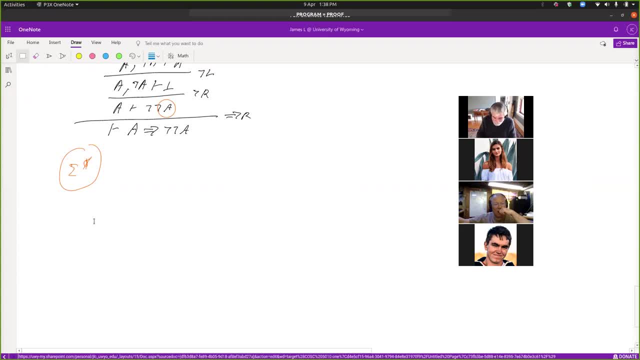 It's a star operator that we use in regular expression, so it means you know all strings, including the empty string. So this is, you know, the set of epsilon, and then you know whatever. if this is you know. 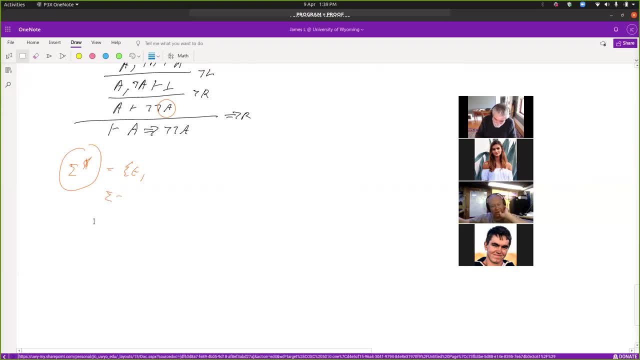 A, B, C, D, So all finite strings include. so it's an infinite set of strings, but all the strings in the set are finite, All those finite strings over the in the alphabet. it's kind of well-known for that in computer science, but he did also. 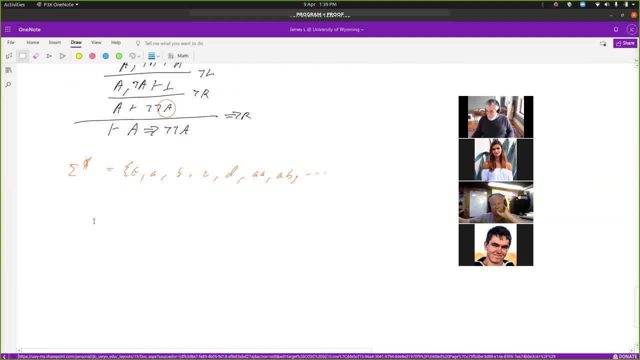 he worked with. well, he was the one that figured out a big stumbling block with Church. He was a student of Church, a big stumbling block with Church- working on lambda calculus and trying to show that you could actually do arithmetic and it was subtractions really hard to define as a pure 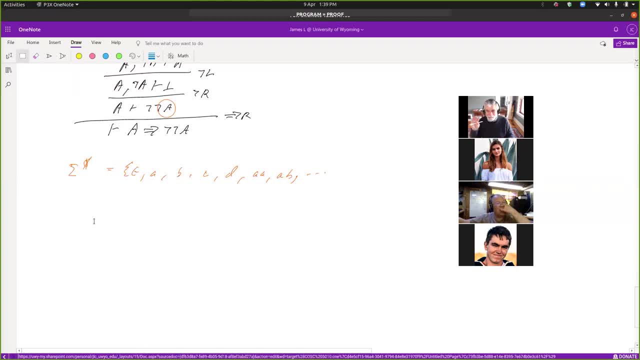 lambda term, and there was Church and Barclay-Rosser who were. so we have the Church-Rosser theorem that we talked about. Rosser was a student of Church- and then we have Kleene, who was a student of Church. 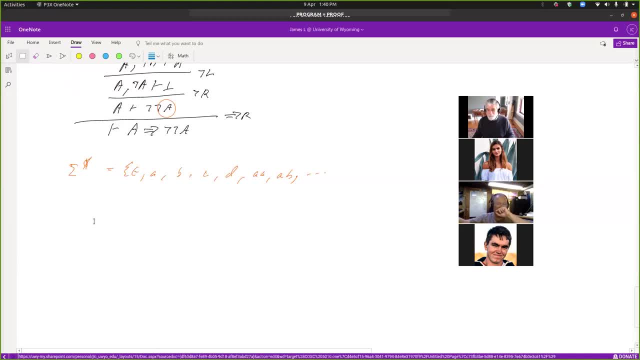 and the three of them were working like mad on this. but I mean, what a great thing like to be a PhD student of Church when he, after he'd just come up with this thing and just trying to work it out. Anyway, what I wanna try and show you is how. 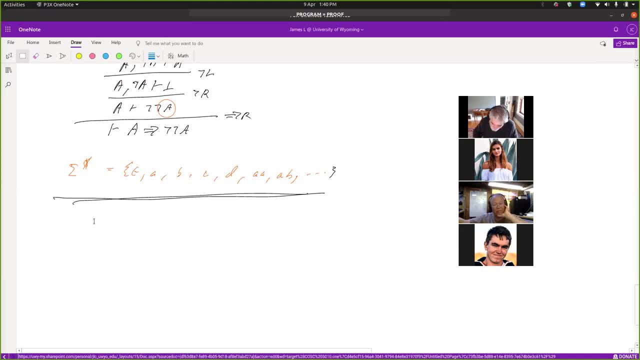 maybe I should just try to do it up here, but I don't know if I have room. Okay, I don't have room up there on those, but let's look at the axiom rule Now in our new contexts are of the form. 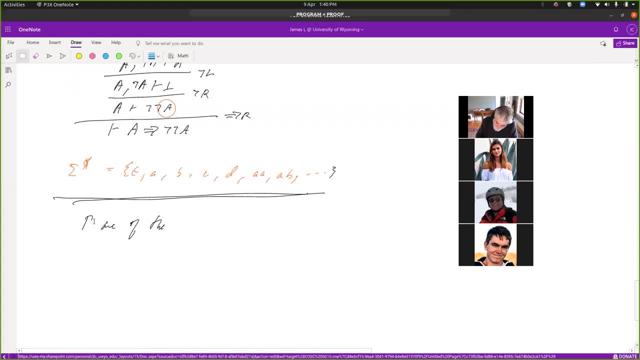 x sub i, colon, phi sub i, where phi is a formula and x sub i is a variable. Okay, So we're not just gonna throw the formula to the left Every time we put a formula over. we're gonna add a variable, a name. 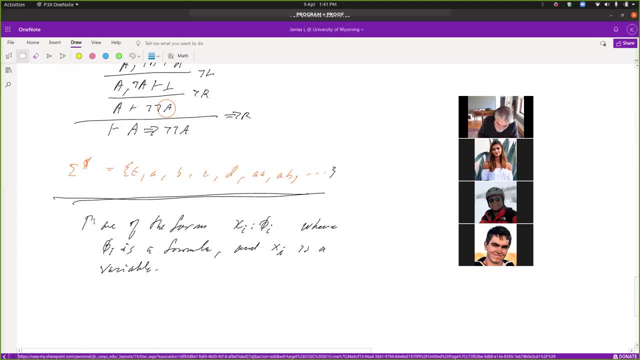 so that we can refer to it. So then that means that you know your axiom rule looks something like this: x, colon, a, comma, gamma, prime term, style a. You're trying to prove a and a realizer for this. 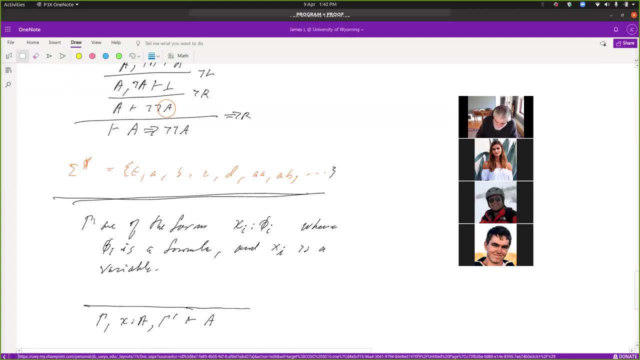 or a term that shows this is. we can say, the extract term that proves this is x. So we're kind of like pointing back to the name of the thing. So this is the axiom rule And then we can say what's the implies on the right, let's do. 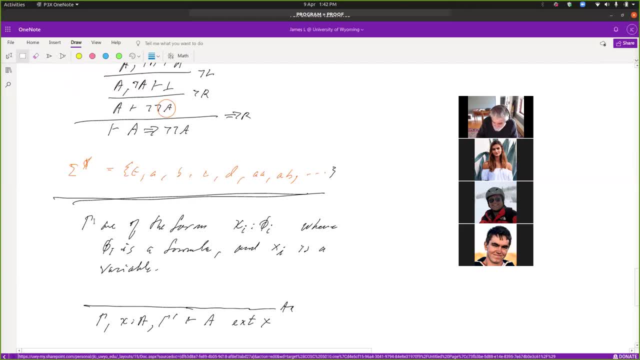 So if I have some gamma term style I've got a implies b. I take gamma, I add x colon a to it where a, x is new, And prove b. So what we need to prove again is the new term. 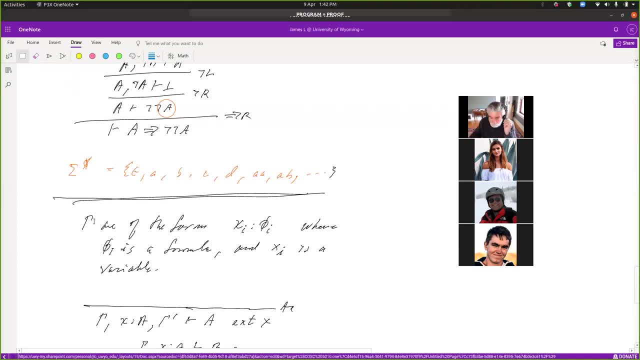 So if I give to this guy a new int, it will give us some new value because we're gonna use it another time. So I'll just show it here. So if I give it a new int, I'll call this script. 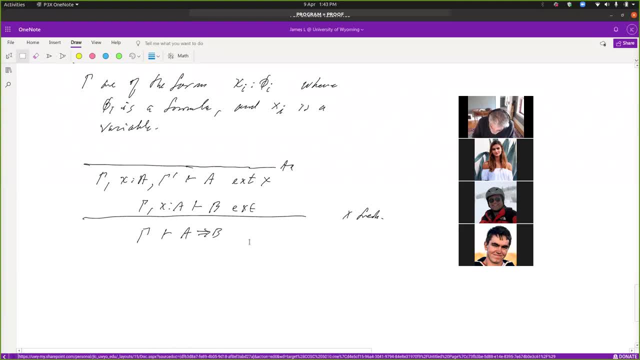 so it will say, if this is a new term, it's gonna give us some new value. And then I'll add a new null which is gonna give us a new What about? so that's implies on the right suppose, and oftentimes people will label: 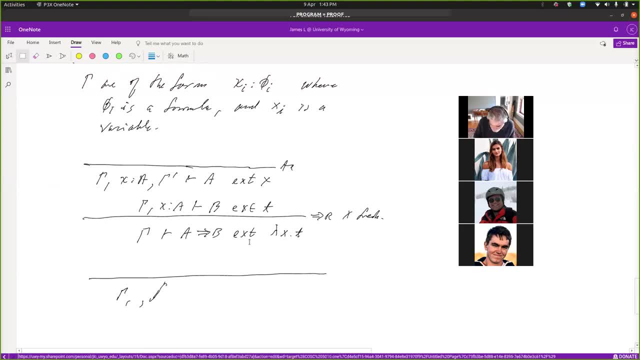 something like this: like F is the label on A, I wrote B because it's going to be a function, And so what was the this? hopefully this rule will actually kind of like help explain also the rule for implies. So in one case I need to say, okay, gamma, one comma F, colon, A arrow, B comma, gamma. 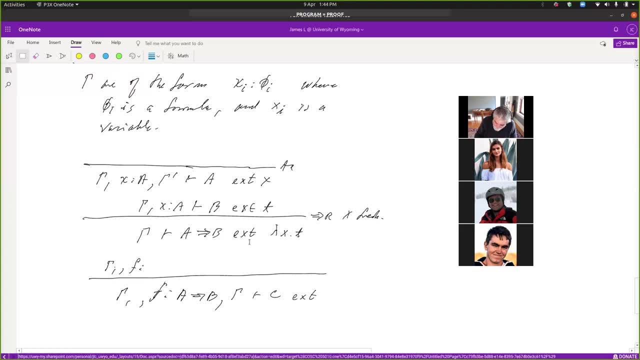 prime. I'm going to have to show you this. So if the extract of this is, let's say, T one, and then on the other branch I get to assume B, right, So I show this, and now I can assume B, And so I'll call B, you know Y. 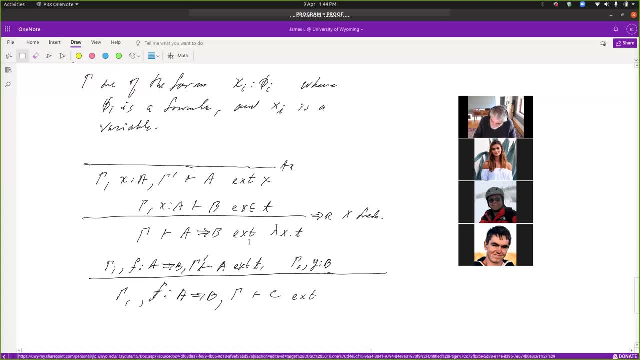 And I prove over here C. So what's the extract of this? Well, call it T two. So I've got a T one and a T two And now. so what's the extract of this? Well, it's F. 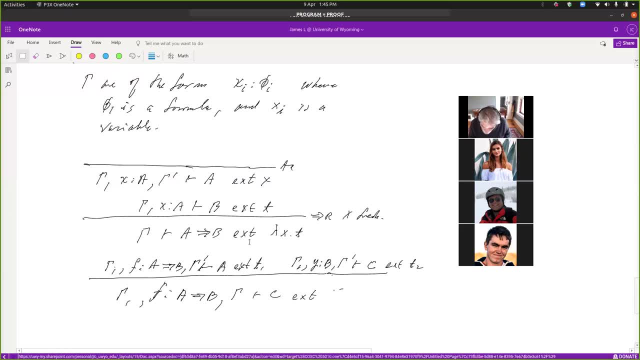 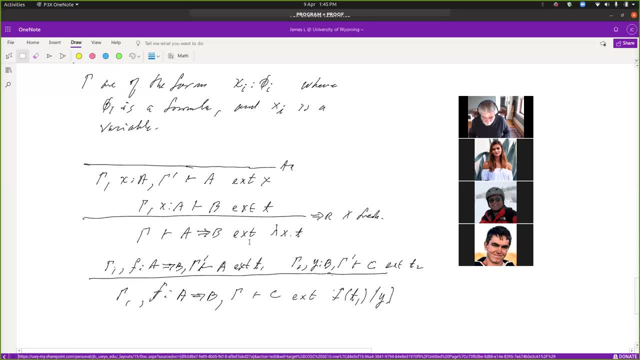 in t2.. Because y is b and if I apply a function from a to b to something of type a, I get back something of type b. So this thing here, you know, this thing here is f of t1 has type b and y. we can clearly see here y has type b. 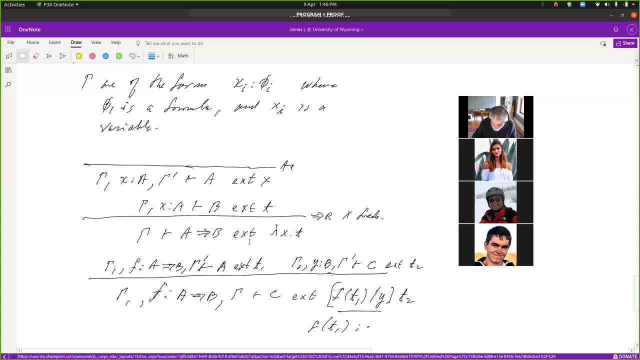 And so how did we? how did we? what was the evidence for b? The evidence for b came from proving a and then applying f to whatever the evidence for a was. Does that make sense? So I mean, this is probably enough to prove something. If we can think of somebody, help me. 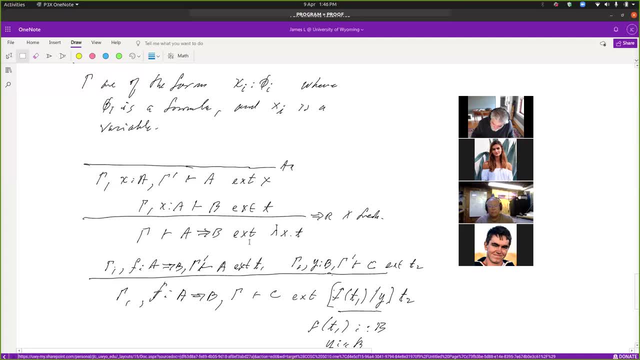 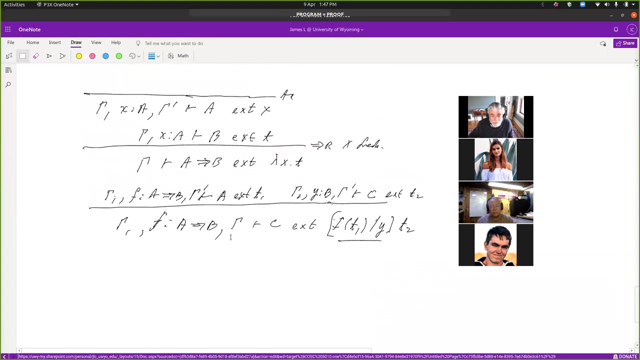 think of something interesting that will require us to use the left and the right implication rule. What's a formula? So I want to. I mean it certainly has to have all right. so those are our rules. I wish I could figure out how to zoom on this. Maybe does anyone know. 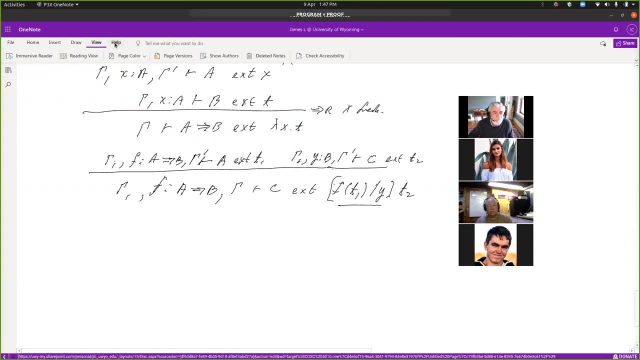 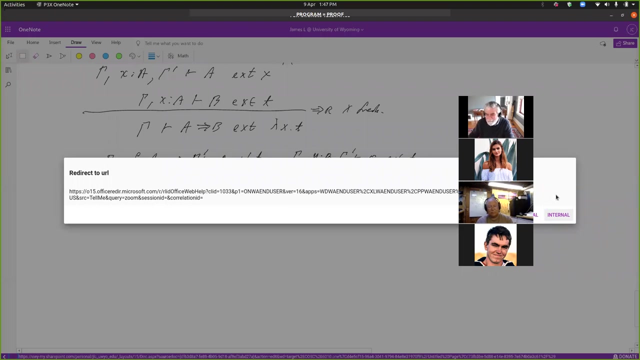 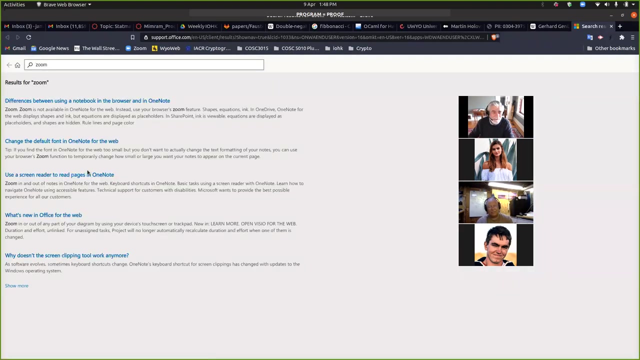 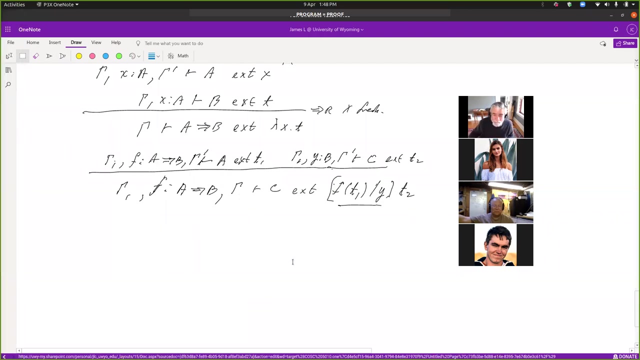 You? no, Tell me what you want to do. Okay, zoom, Okay. now, how do I get rid of that? Okay, Oh no. what's happening now? Oh, okay, Okay, All right. whatever, That's not going to help. All right, let's try to prove something using 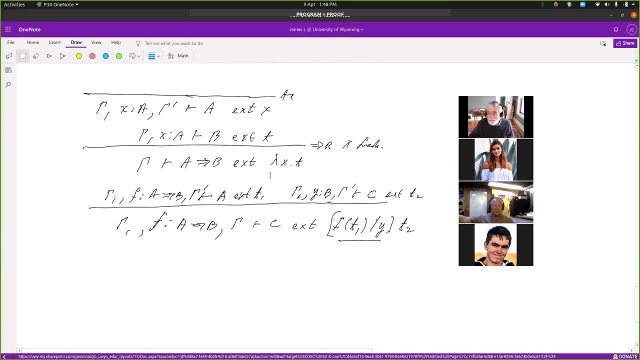 these rules. I'll have to. I don't know how to make them smaller so that we could continue to look at them, But anyway, what would be a formula where I'm going to have to use both those rules? I would say, like: p implies, p implies, q implies q. 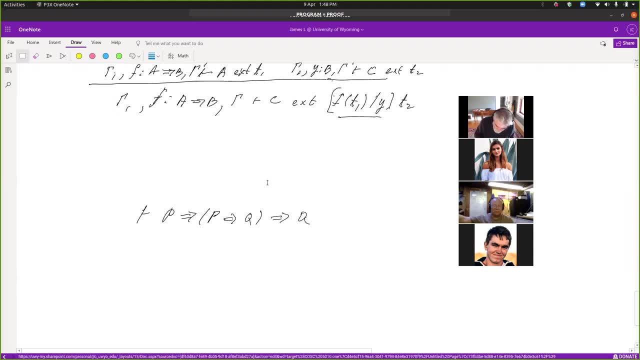 And what's this program going to look like? What's the extract of this? Well, I'm going to say p is x, And then I got p implies q implies q, And I'm going to have some kind of extract there. So the proof rules you work up and then the extract. 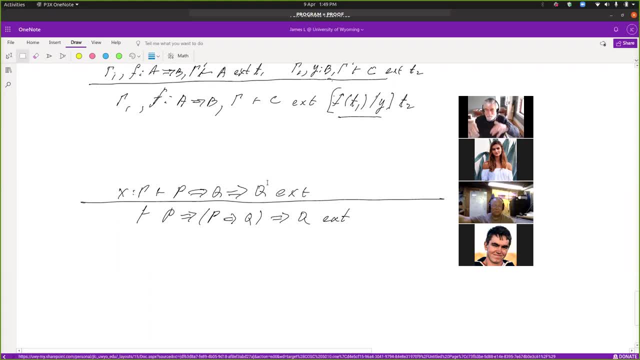 or sometimes what we call synthesized attributes. if you've ever heard about an attribute tree or that an attribute grammar, this is like an attribute tree, because the proof rules help you work up to build the extract terms from the smaller proofs with the axioms. Okay, so that was. 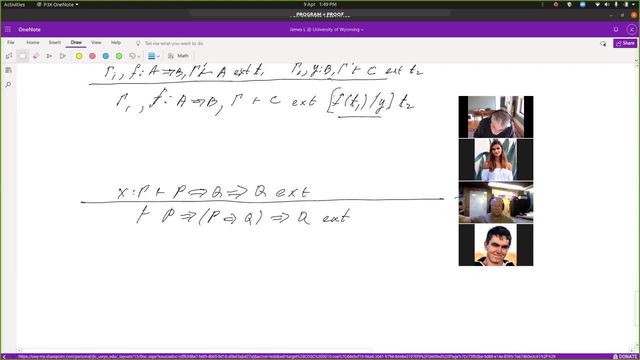 implies right, And then I got to do implies right again, And now I get x colon p and I'll call this one. oops, this is p. I need my parentheses there, And so I'll call that one f. it's a p, arrow q and I got to show q. 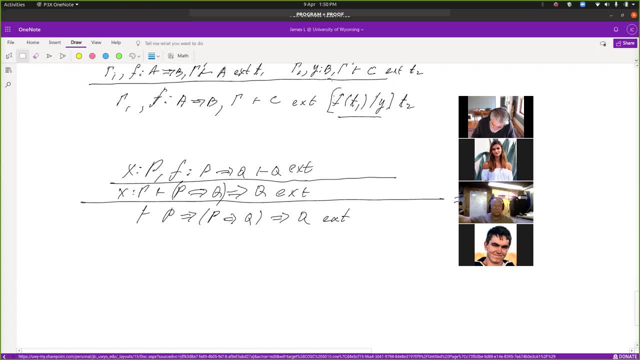 And need more room. so that was another implies on the right, and so now I have to do: implies on the left and that's the. that rule is just visible right here. so I have an F P, arrow Q. so what do I have to do? I have to say X, colon P, that's my. 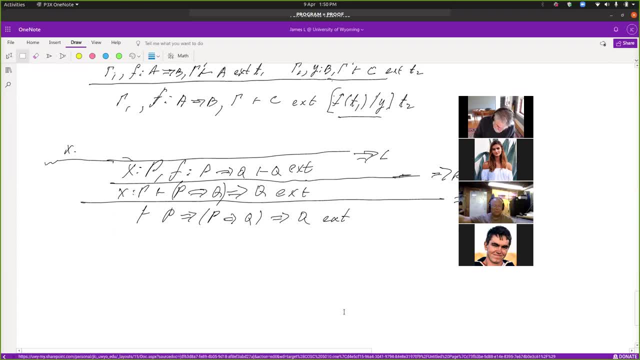 gamma. and then I've got F, colon P, arrow Q, and then I've got gamma. prime is empty. and so then I got to show P. you over here I've got X, colon P. I don't have that, and I have a Y, a new thing of. 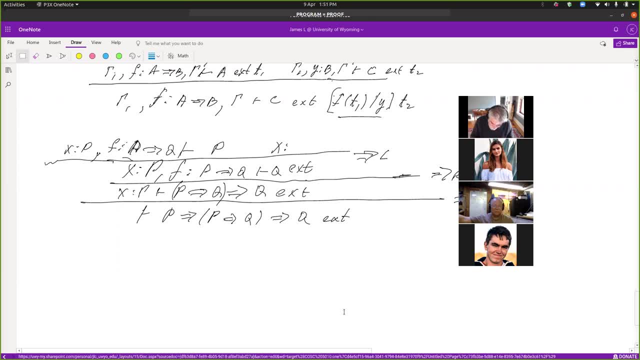 type Q and I have to prove Q, and so the extract of this is Y and the extract of this is X, and so the extract down here is F, so the extract down here is: apply f. I moved the player here and I pulled out my joints and I'm a surprised item that. 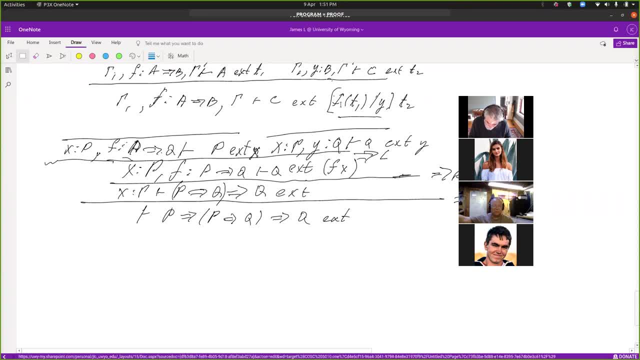 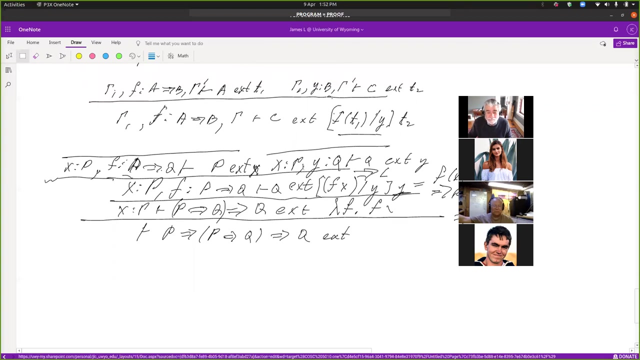 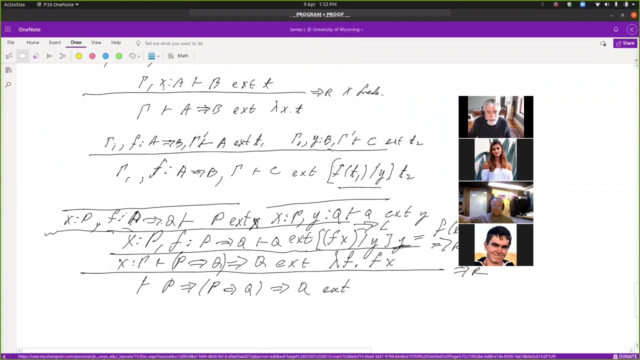 well, a ball, or I, I. you see, I and I too, all the ways in the your Gabriel, You ci you. the extract on it implies right role. this one would be lambda f dot f of X, because the rule says: pick a new variable to name a, and in this case I picked a new. 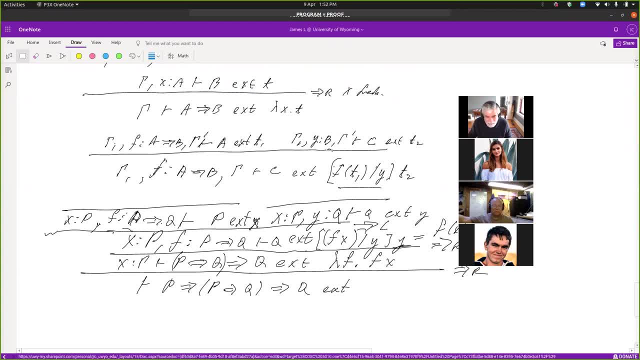 variable to name f, and so I get lambda f and then you just write down whatever the extract is up, there is the body of the lambda, so f of X is the body of this lambda. and then we go down here and now we have lambda x, dot, lambda f, dot. f of x. 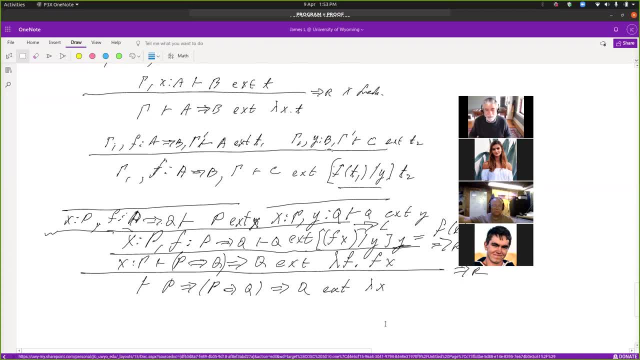 is the term that you can build out of this proof using these augmented extract rules. so I haven't read in the book about this curry style, but this is curry style because these terms are not annotated. they're well typed. this term definitely has this type because it came out of the. oh, I didn't mean to move that. 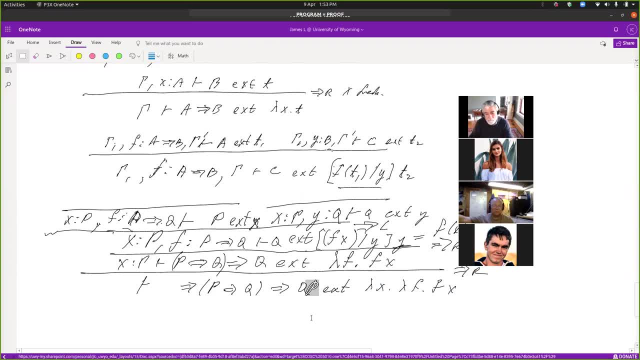 out of the. oh, I didn't mean to move that out of the. oh, I didn't mean to move that. come on, go back. what is it doing? okay for something, and grab it and put it over there- and I think I can fix it on here and and remember our associates to the. 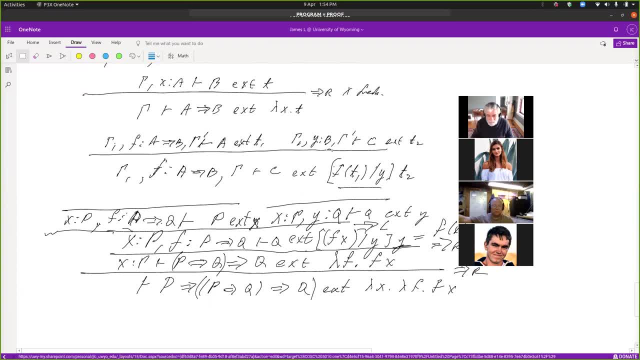 right, so that means that right. that's how we pulled off the X. so lambda X- X is something of type P. lambda F- F is a function from P to Q, and then to get my Q I apply F to X. so that should be perfectly sensible you. 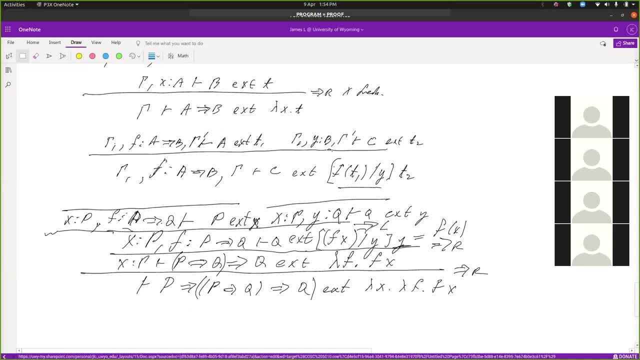 yeah, two y'all. are you there? you, what do you think? can you see this? yeah, I can't see, but it's hard to read for me, okay, Um, okay, Kyle, all right, I don't know. Keegan, do you see this? What do you think? 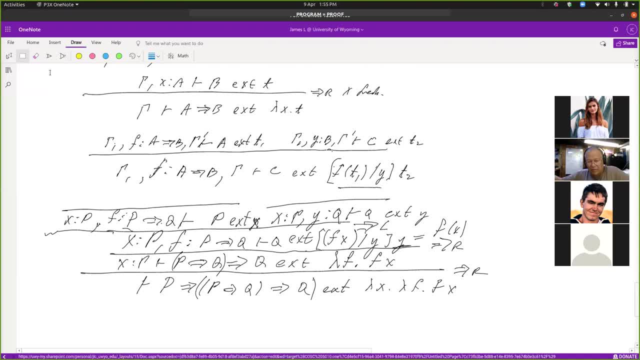 This makes sense. Okay, so this is like a different kind of. it's a similar thing to the Curry-Howard, but you just, I mean it's. you know, it is Curry-Howard essentially, except that you now, maybe in the Curry style, you might write something like: lambda x, dot, lambda f, dot, f of x as type. 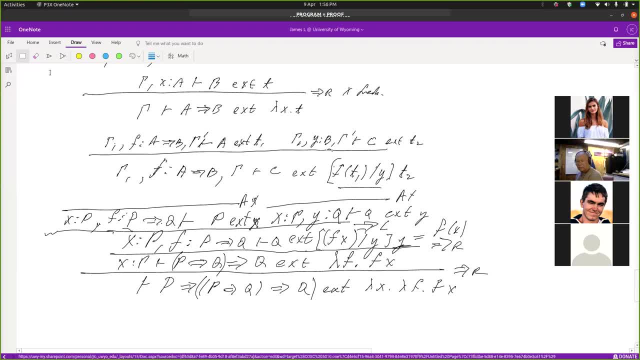 And you might, you might do it this way, where you take this term and put it in here, but in this way, so this is like a verification, would be a verification that this term has this type, Um, but this one. 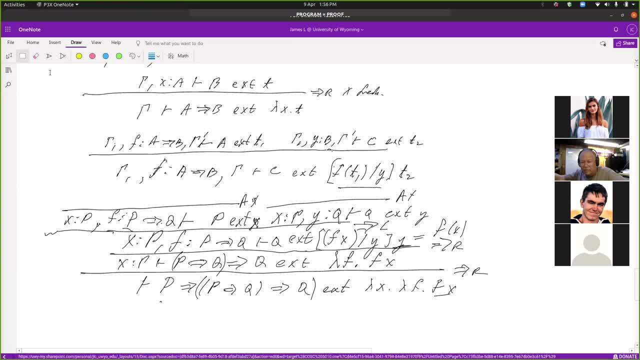 um is: you build the term from the proof, You extract. it's a, you extract the term. This is what Koch does. in the Koch, they get programs from their proofs um by extracting them, as opposed to. I think in Agda you're more like you're building the terms as you go. 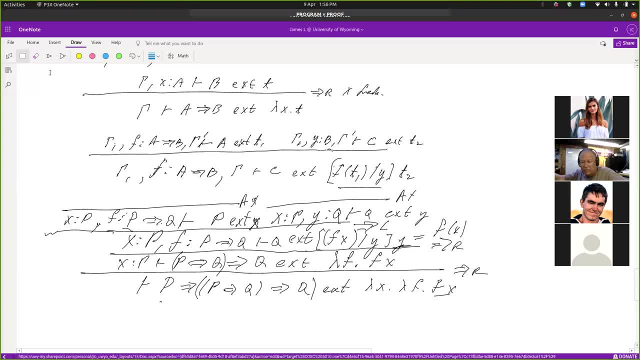 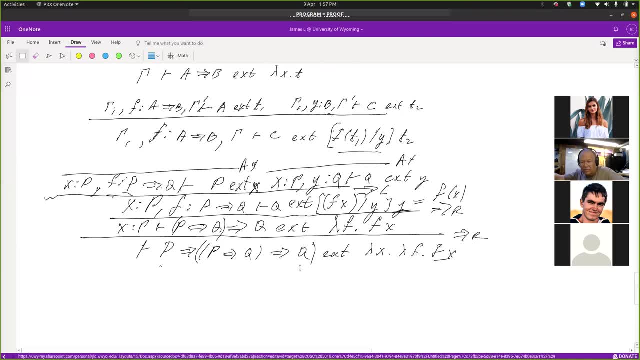 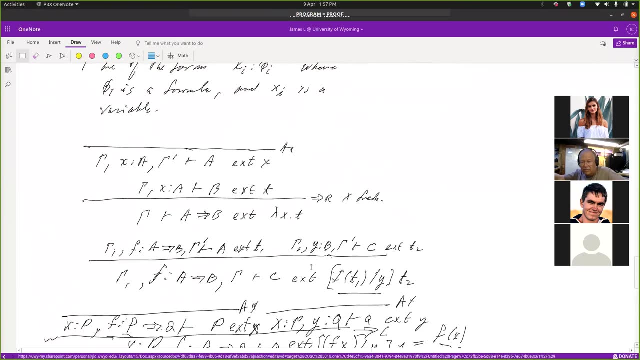 Um, and this is how Neuporil worked: It extracts programs, programs, from proofs. So we're almost out of time. I wanted to do quantifiers. Um, you know, you can design rules like this for all the other connectives. 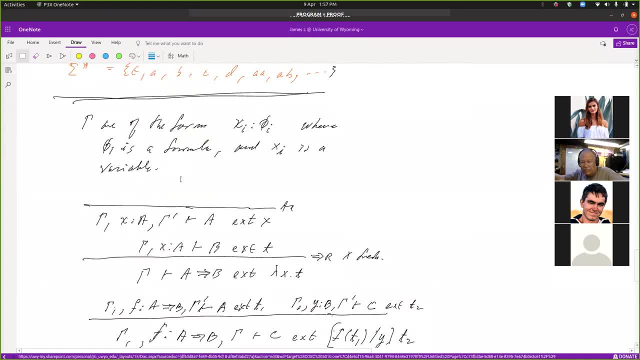 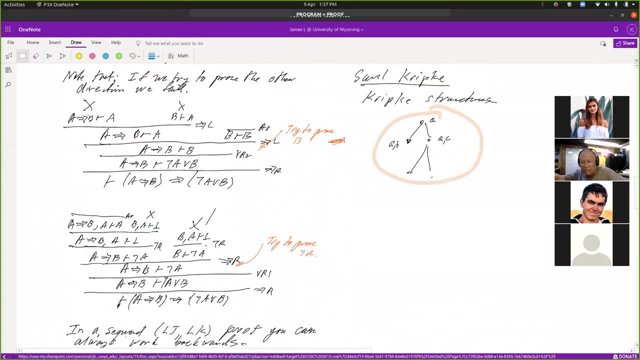 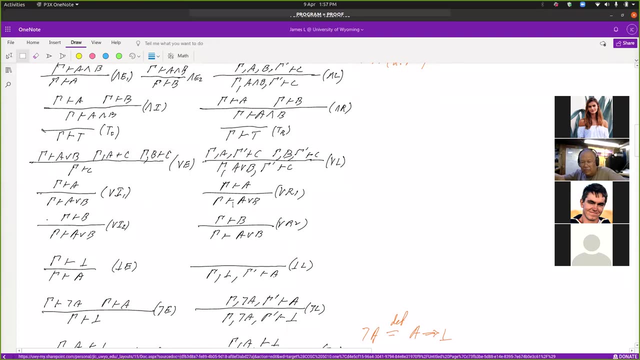 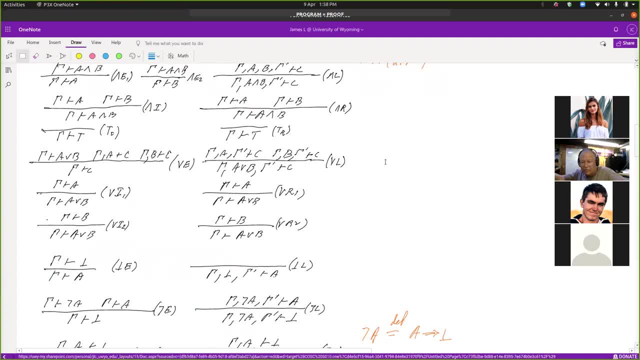 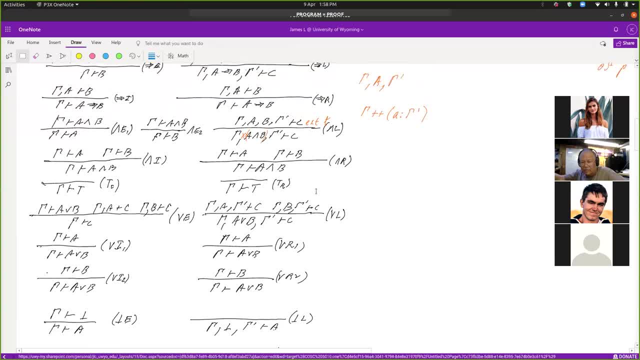 Oh, I need to scroll down just a little bit maybe. and then we got to give these y and z new names, and then you take t and you substitute, you replace all y's by pi 1 of x. Oh, I went orange. 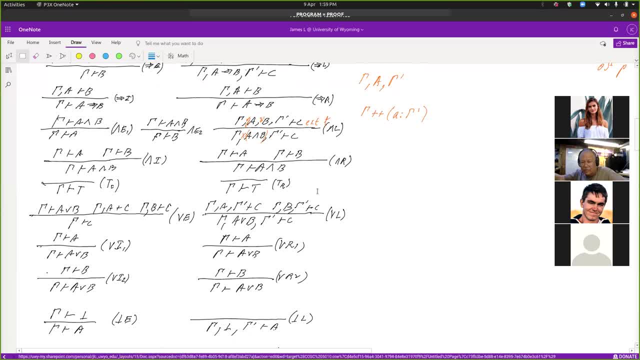 So the extract here is: it's going to be the term t, but every place you see a y, replace it by pi 1 of x. so say pi 1 of x, the first projection of x for y, and replace pi 2 of x for z. 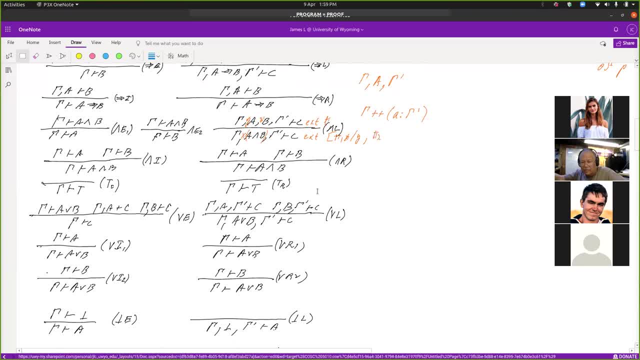 and do that substitution in t. All right, And the other one or is a little weird because. or is a little weird because. or is a little weird because suppose the extract is t here, then the extract down here is left of t. 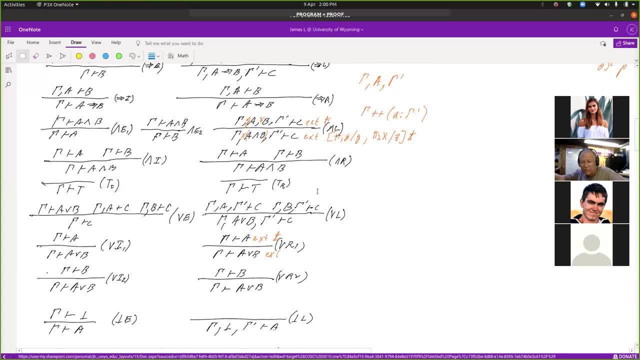 and if the extract here is t, then the extract here is right of t. A lot of times, you see, instead of you know, the either type says in Haskell, you just tag which one it is. So this is like an or type. 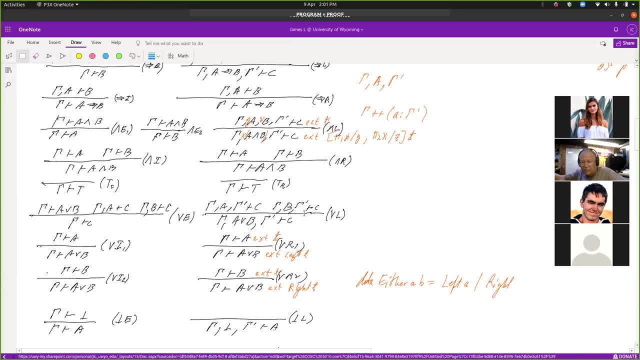 You could also say: you know, um, I don't know, I could still call it either. You could also. it's common to see in left a or in right b. These are pretty common projections, But 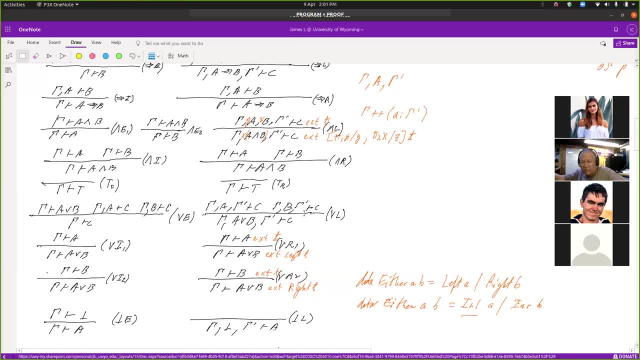 but then when you have one of these, you need a way to operate with it on the left side, Like: what does it mean over here? And I forget, and we're over time, so I'm not going to hold you up. 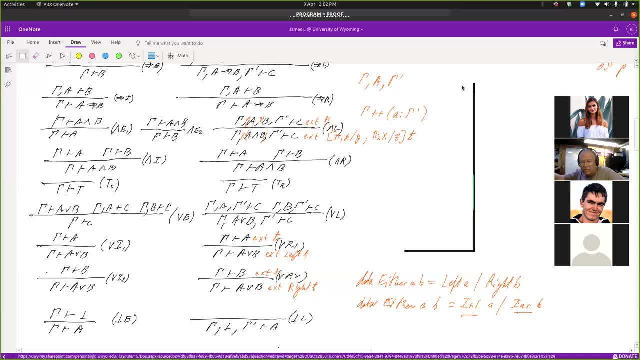 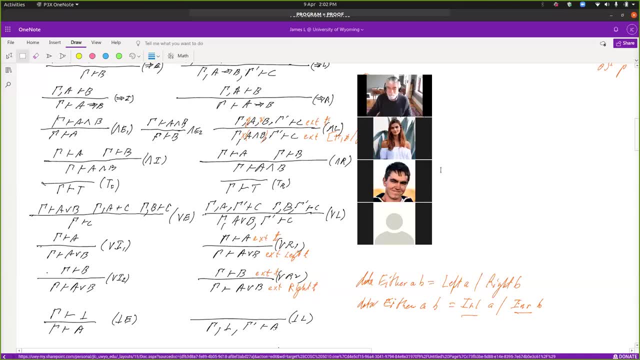 Anyone who wants to stay and talk a little bit more about this is welcome too, But you know, two hours is a pretty long time. Any questions, Comments, All right, look, we're getting down to the end also, So I think next time rather than. 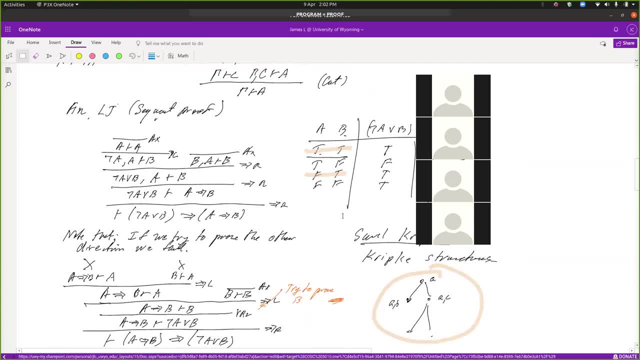 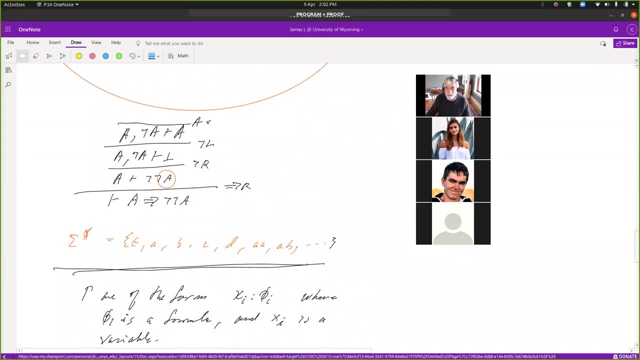 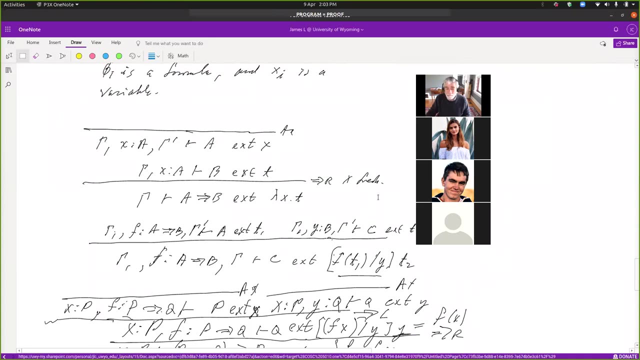 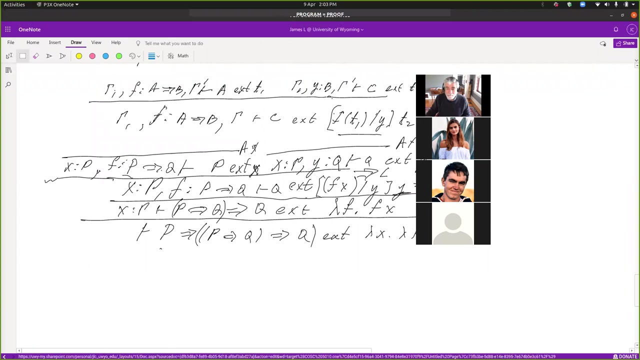 doing the quantifiers. maybe here we'll, we'll see them come up in system F. I think we probably ought to move on and and start working with system F. What do you think That sounds good? Okay, All right. 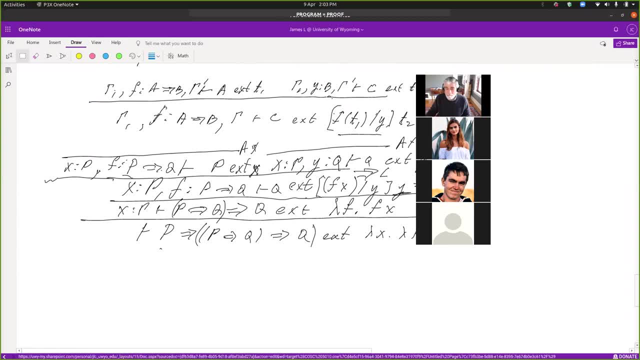 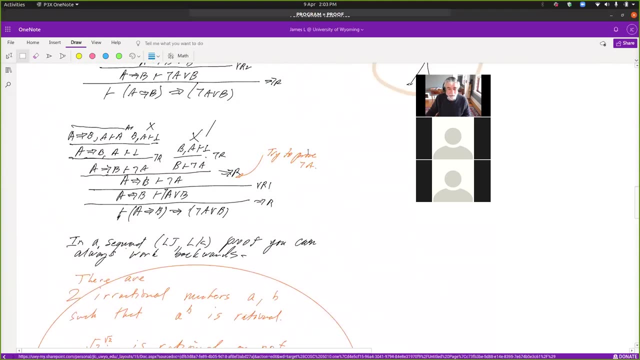 Thank you all for coming. Thank you, sir. Yeah, You're welcome, And are you actually going to go through with the possible homework you just mentioned? I don't know. What do you think? Does this seem- I find it useful, I think. 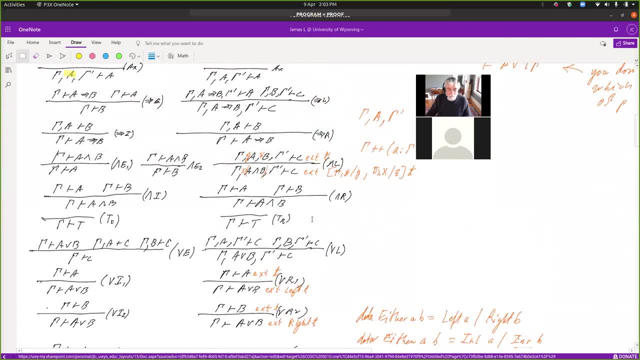 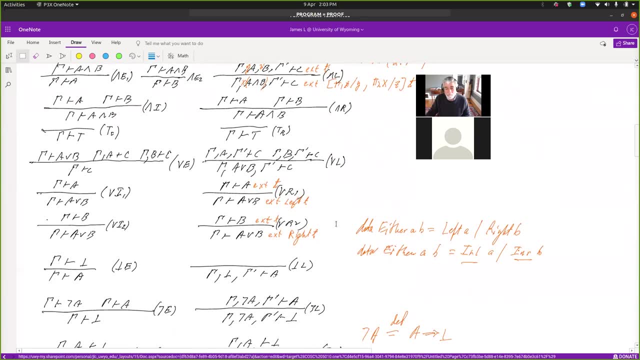 Yeah, Okay, I think I will. I'll put this up as soon as I'm done here on the page, and maybe I'll ask you to Um to write out the extract terms for the other ones. The decide is the one that's hard. 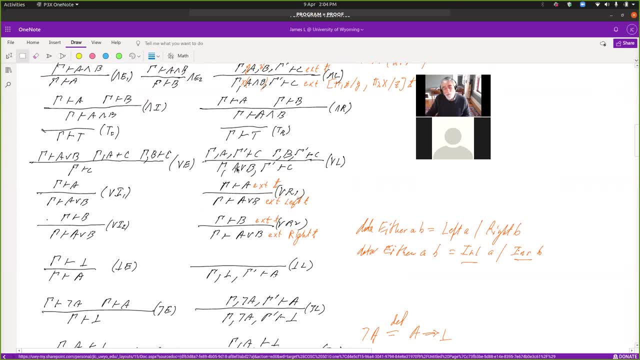 Um, I mean the or there you usually write- and I guess I could write it here, as you usually write a kind of a term that's like um, defined to compute, in the following way: You say: like decide. 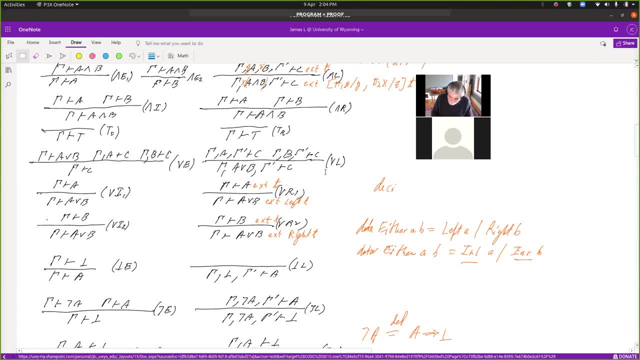 And you say left x? Oh, how do you do it? What do you say? Design? Oh, I think you put two terms in here. Yeah, This one would be very hard to come up with. Well, you might be able to find it in. 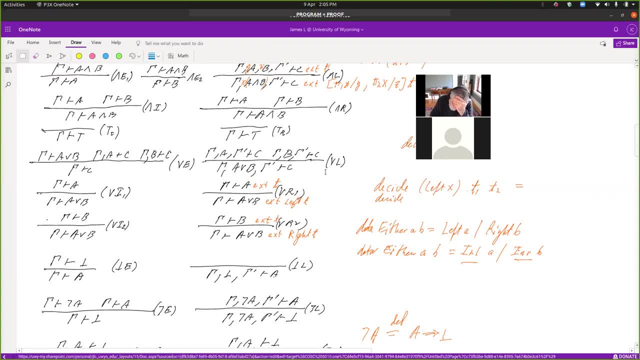 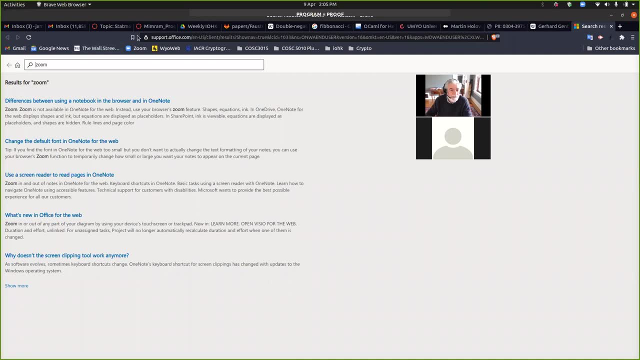 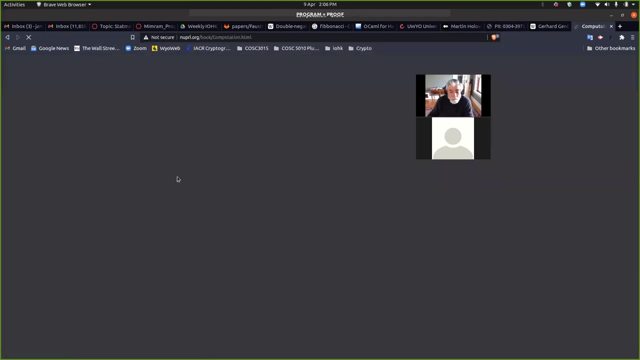 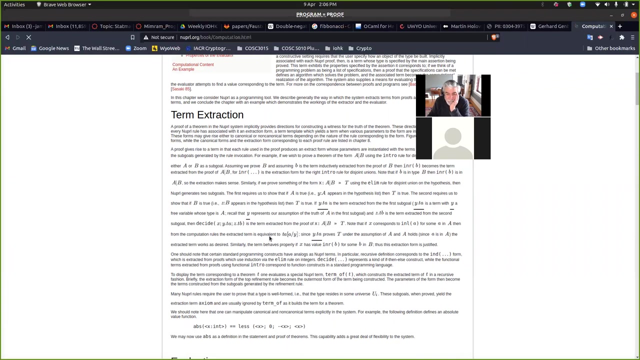 Oh, how does that work? Come on, how can I not remember the decide term? I wonder if I can Google it. All right, Okay, so the side is of the form x. semicolon y, dot. t. a. semicolon z, dot. 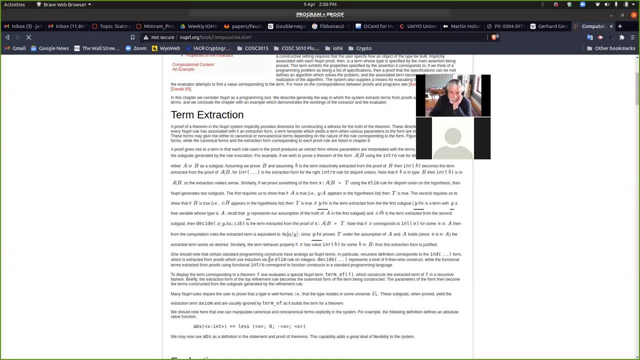 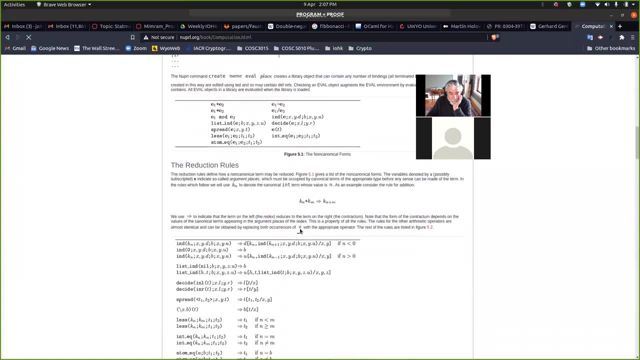 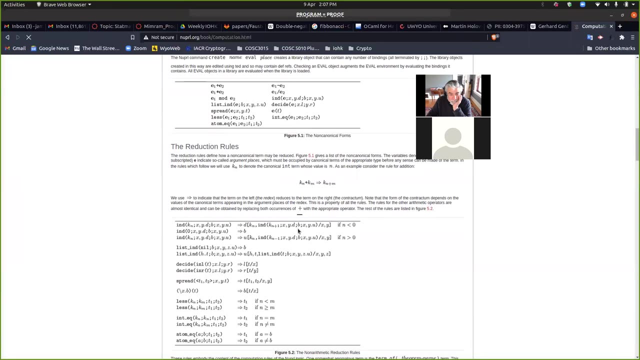 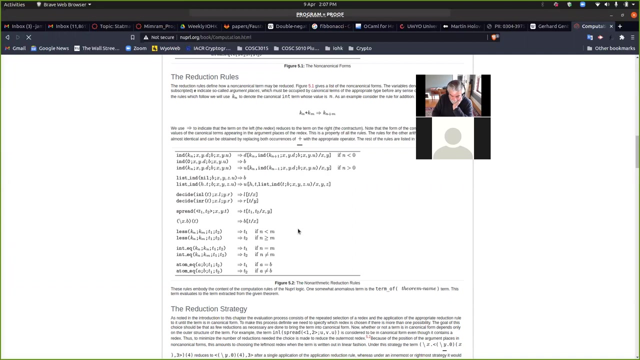 And so I'm going to call this t1, t2.. Okay, so Decide in left t or left t. semicolon x, dot, l, y, dot, r is evaluates to l. Okay, but they changed it, So it's t1.. 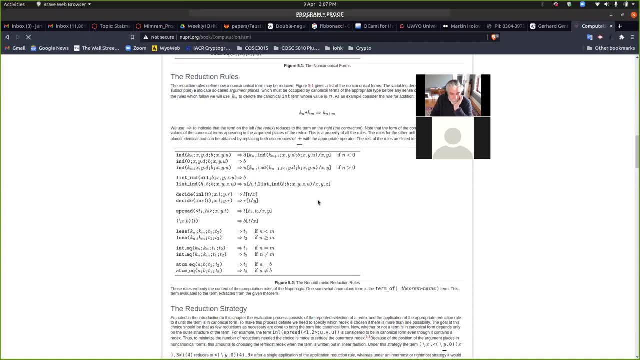 But this is the same. It's not even going to be that Okay, so OK. so I'm going to call this: t1, the left, t semicolon y, dot t, dot y, dot t. semicolon y, dot, x, dot. So l two t semicolon y, dot t. 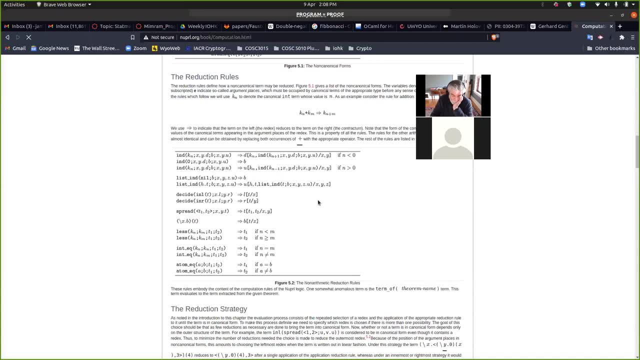 So this is my left t semicolon. I have been using that And I'm not sure if that's too much. I can call it both. I'm going to call it two. t semicolon, y dot and t two, And I'm going to call it two. 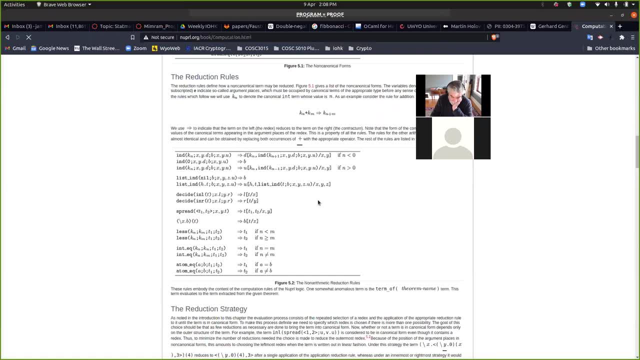 It's going to be one, I'm going to call it two, So that's one. So this is my left t semicolon: y dot t. Let's see it's an interesting operator because it's a binding operator, just like lambda is, and so 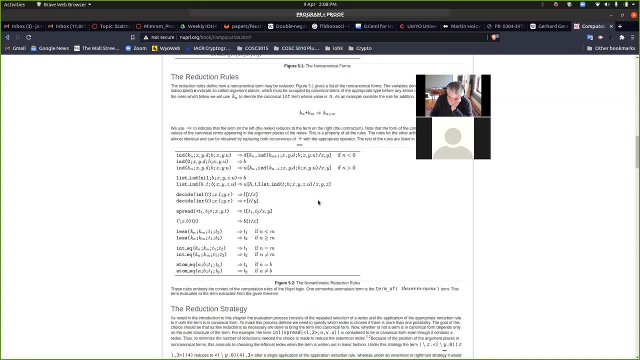 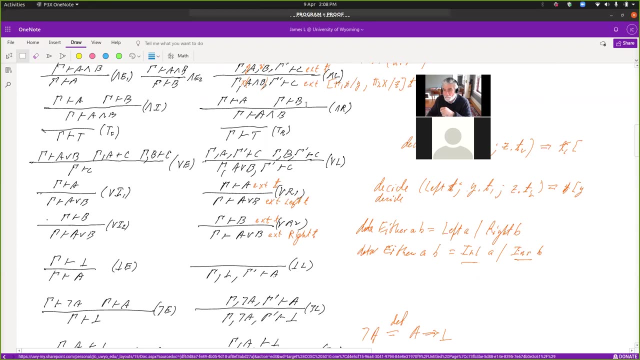 you take t1 and replace all the Y's by T, all right, so let me show you my notes here. I need to erase this one that's gone so you can think of what's the type of decide. I'll tell you in a minute. I can write down here if I 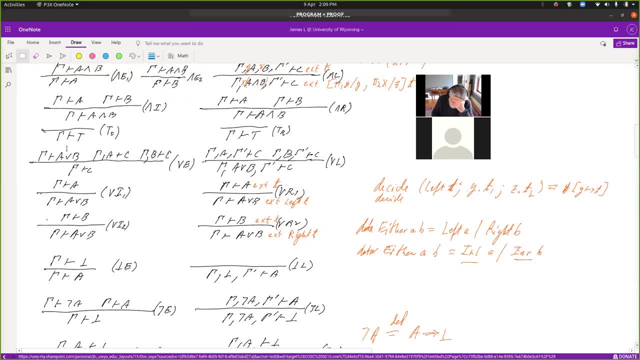 see a write applied to some T and then I have a yt1 semicolon, zt2. that's equal to T two. so this should be t1 up there, t2 where Z becomes T. so this may look really crazy. I think it makes sense. so one way to think of this, one way to kind of like 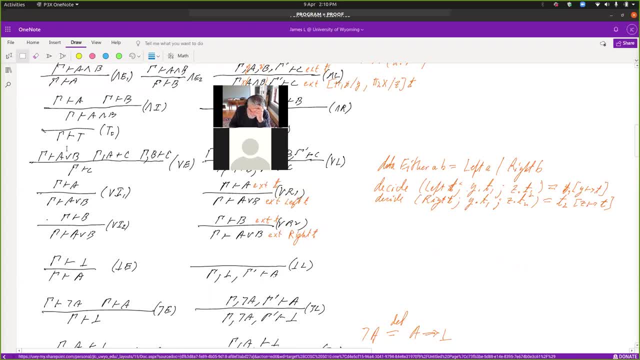 implement this thing is to say in Haskell it'd be like case so, so like you'd say, okay, decide X. and then this is like you could do it: f1, f2 is equal to case X of. if it's a left of some T, then what you do is you apply f1 to T, and if it's a right, 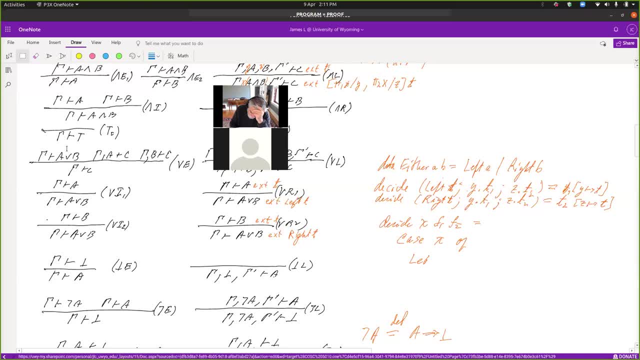 of some T. then you apply f2 to T. so what is the type of this thing? this thing is decide has type. I guess I I could try and let me undo that and break the type above it, but I'll have to move it down a little bit. 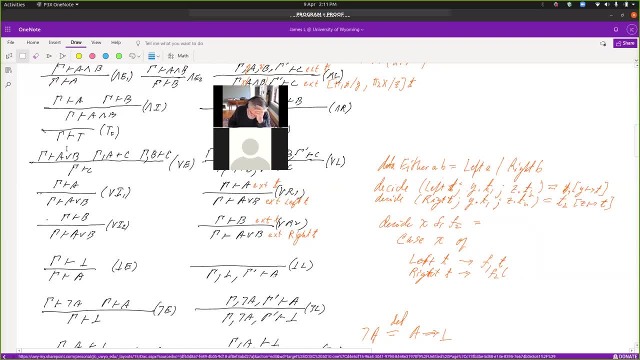 but what you can actually do is if you do x plus something before it and u plus, and then you do u and it gets equal to S, including the layer thickness, if you chop those down. so that's it. then this is plus plus if you give it x. 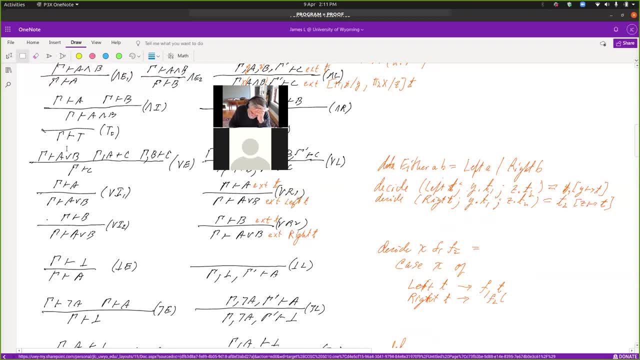 so this goes in that order over here and that's what you're doing. it brings to a nice new combination. so it's easy to get things in that way. if you're- if it's some kind of abstract property for broken sets of is a function from a to c. so that's f1. here's the f1. this is the x. the f2 is a function from b to c. 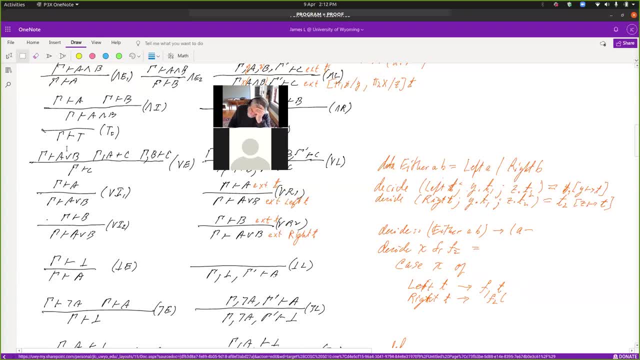 and it finally returns a c. yeah, that makes a lot of sense. good, wow. so here's how decide is implemented. so that means like in practice. if you wanted to actually do it, though, you got to provide like lambda term instead of see in in in the new pearl theorem, prover this dot gives you like a.